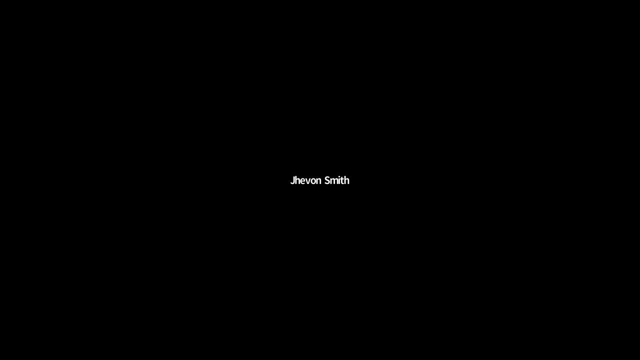 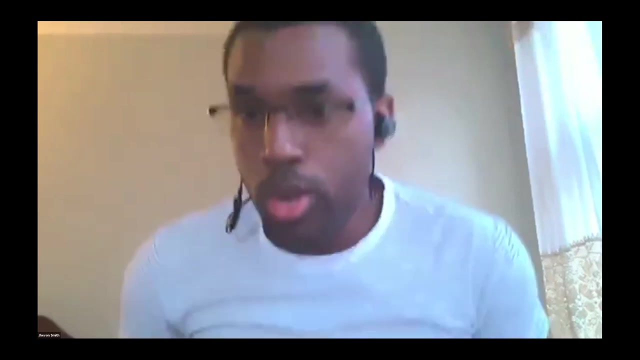 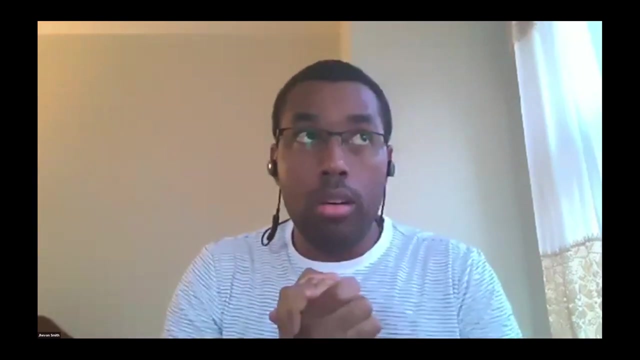 Okay, so let's get this show on the road. Hello everyone, hope you're well. As Jason has been saying today, we're going to definitely start the last topic. Hopefully we can get to finish it up as well. We are going to finish, start and hopefully finish partial derivatives. 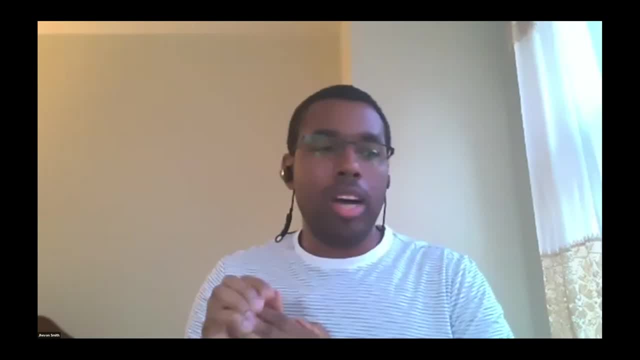 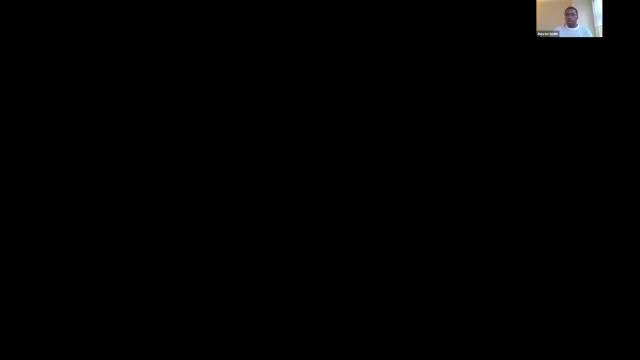 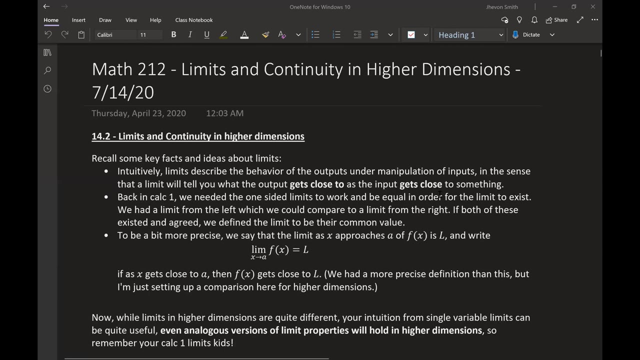 Before that, we had some stuff to clean up from last class, though We have to talk about continuity, So last time we started talking about limits, Let's jump back into that. Boom, there we go And let's continue. So this was on the 14th. We're missing Jason's energy. 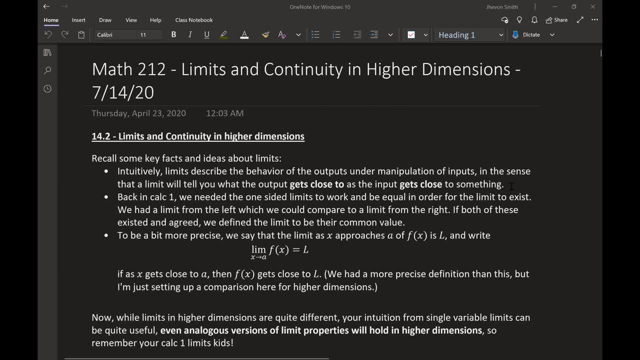 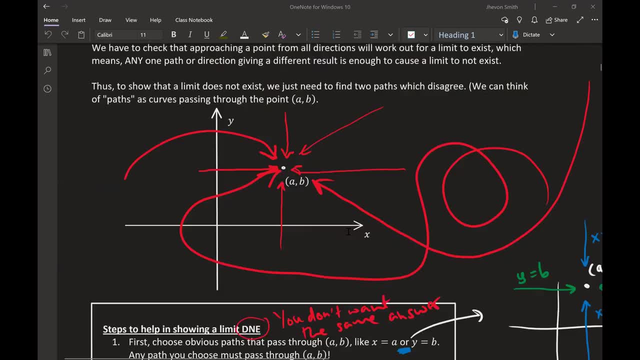 and presence that day, but he's back today, So we're all good. So limits: We have some technical definitions here, but we pretty much went for the intuitive field. We looked at our process to show how, when limits do not exist, 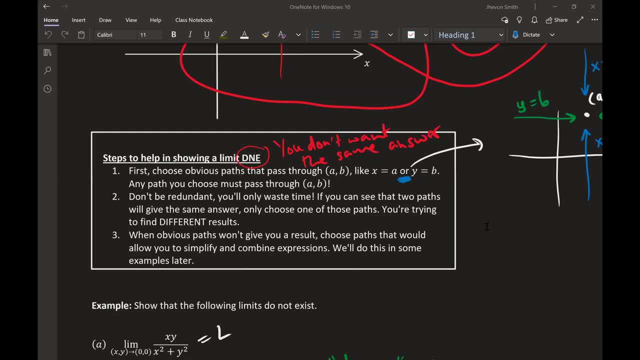 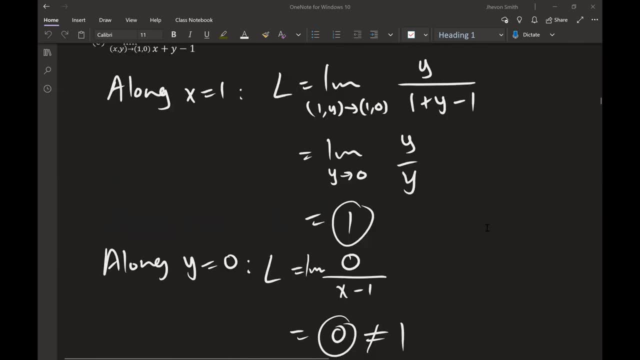 Basically, you just want to approach a limit along two different paths and show that you get different answers. We also saw that we can show that limits do exist via things like the squeeze theorem, via things like simplifying and plugging in, via things like plugging. 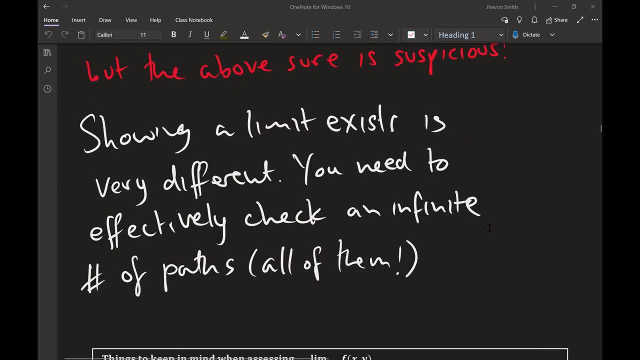 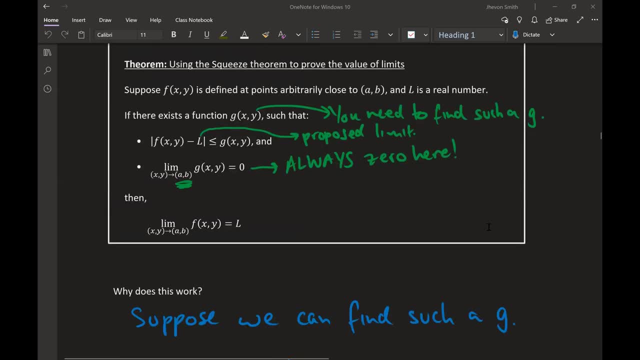 in directly, all that good stuff. So we pretty much spent a lot of yesterday's class just learning how to compute limits, when you would do what, which approach. and yeah, it was all fun, It was all good And we got to. 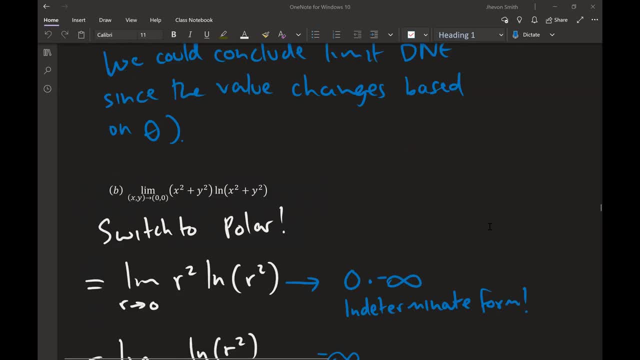 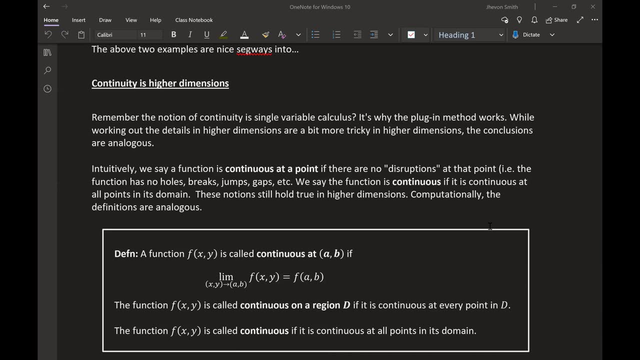 do. a lot of examples, obviously, and we're now boom here. so, um, once we got through limits. how to compute them, how to show they don't exist, how to show they do exist, when to try to show which? um, we got to continuity. now you might may recall doing continuity in calc one, and you may also 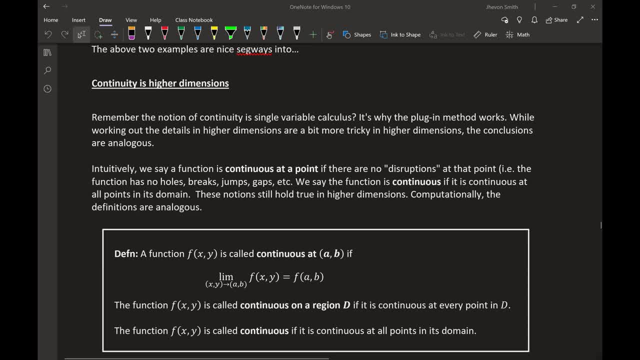 recall that in calc one, continuity was defined in terms of limits. so, uh, we used the squeeze theorem um in the last class, so right now we're talking about a whole different topic. okay, so continuity again. just like back in calc one, it has the intuition that you think it has. so to say that a function is continuous. 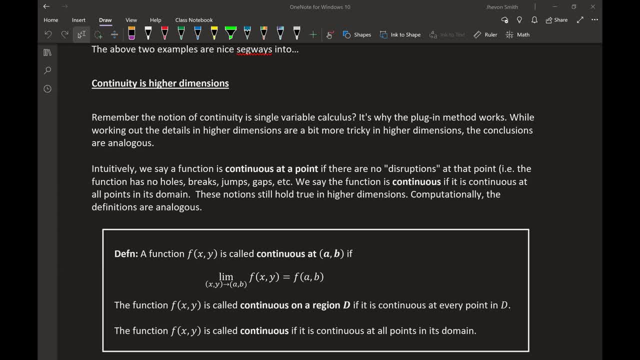 at a point means that there's no gap, there's no hole, there's no break, there's no disruption, and we saw in calculus one that that basically means that the value of the function at a point is actually equal to the value of the limit of the function at that point. and in calculus three, 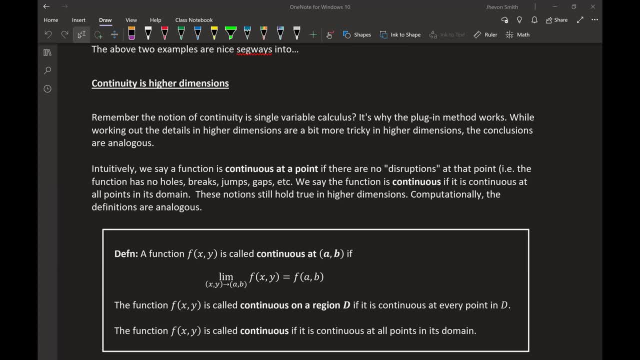 and in higher dimensions, this exact same definition would still hold true. so if we're looking at a two variable function, for example, and we want to know: is it continuous at the point a, comma b, then all we need to do is: we want to know: is it continuous at the point a, comma b? 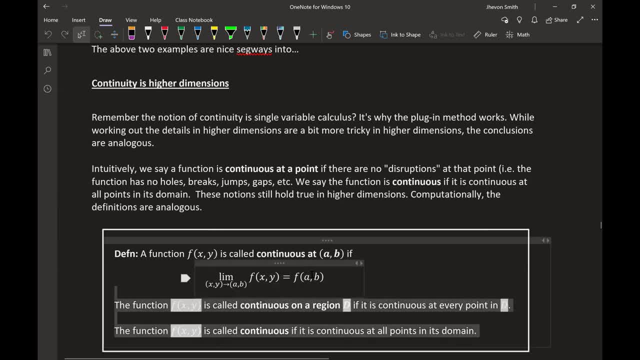 then all we need to do is check this equation: is the limit as we approach a b equal to the value of the function at a- b? and if it is, we say that it's continuous at that point a b? if this works for all points in the domain of the function, we say the function is continuous in general, so that those 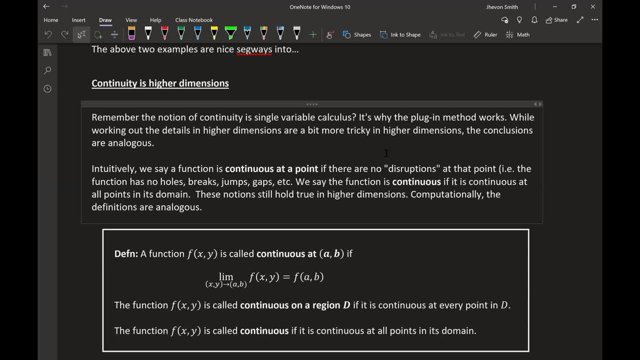 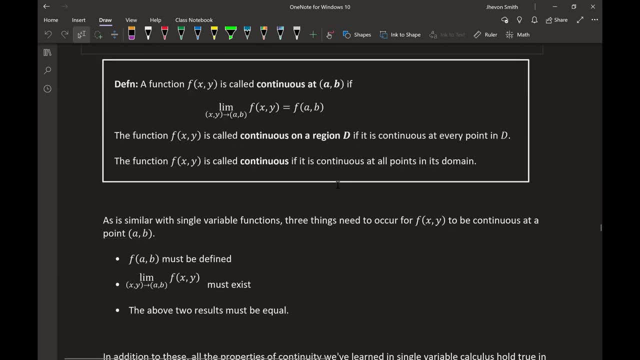 are no new definitions: pretty much exactly the same definition that you had in calc one, except now we have a multi-variable limit, we're talking about a multi-variable function and yeah, so now everything that you know about continuity and limits and all that good stuff from calc one. 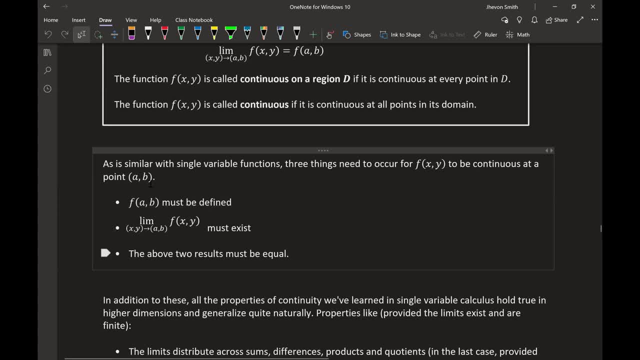 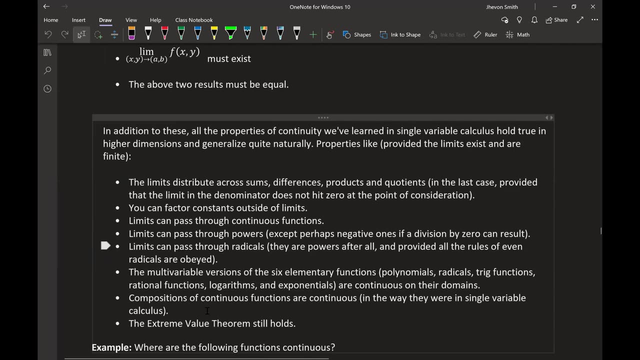 those things are still true. so things like knowing how to check for continuity amounts to checking three steps. the function must be defined at the point, the limit must exist at the point and both must be equal. that you would have gone through in calc one, as well as a lot of the other things are. 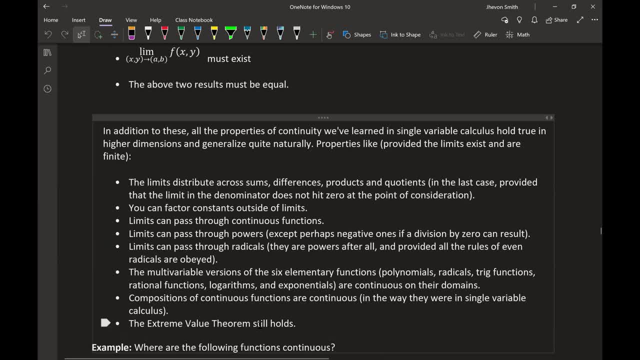 still going to be true. so the extreme value theorem still holds in higher dimensions. limits still distribute across sums, differences, products, etc. you can factor constants outside of limits. limits can pass through continuous functions. um, let me write down an example of what that means. so so, for example, if i want to find the limit of, say, x approaches a of sine of some function, f of x. 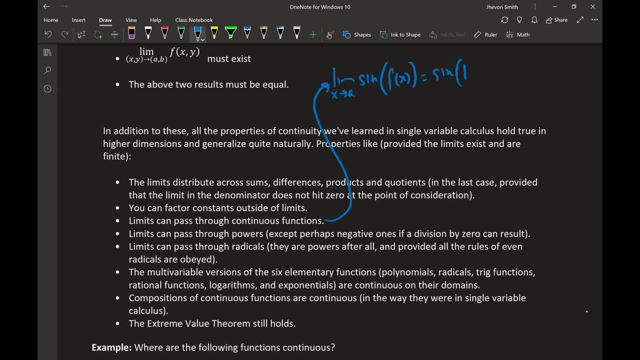 i can move the limit inside the sine function and take the limit of the angle. or if i wanted to find the limit as x approaches a of e to the f of x, then i can move the limit inside of the exponential, etc. right, so all those things that. 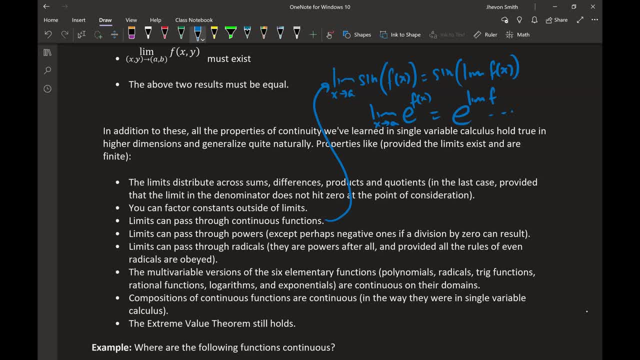 you know from uh limits all those intuitive notions that you have, they're still actually true. uh, as well as that applies to continuous functions. um, composition of continuous functions are continuous. if you multiply two continuous functions, you get a continuous function. If you subtract or add continuous functions, you get a continuous functions. 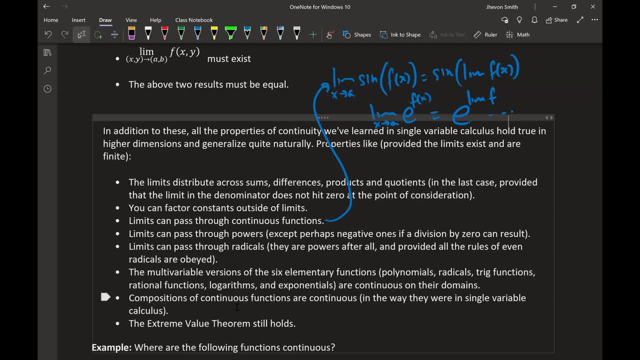 If you divide two continuous functions, you get: the result is continuous as long as you're not divided by zero, et cetera, et cetera, et cetera. right, Lots of things that you guys are very familiar with that I'm just not going to beat anymore. 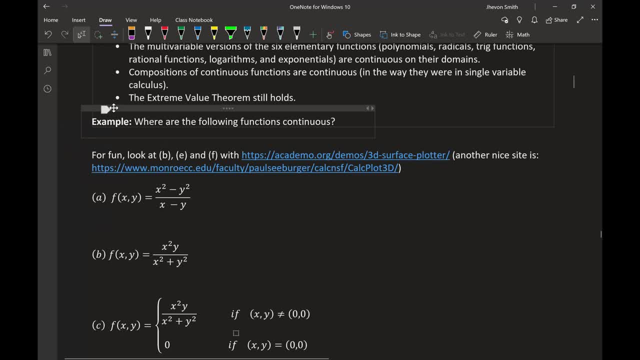 with a dead horse. So we're going to pretty much just jump into some examples here. So we're going to do some examples And today- and this is why today's lecture might spill into tomorrow's lecture a little bit- is because I want to actually show you some visualizations as well, because that's 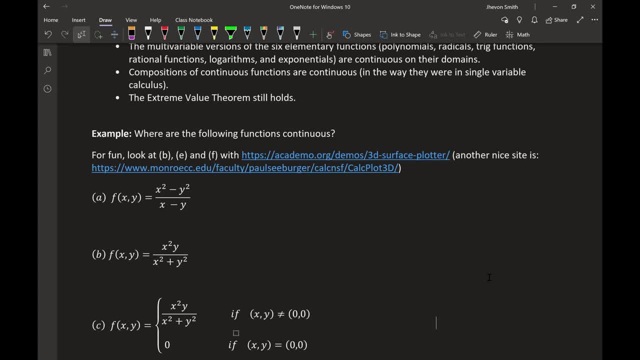 always nice. So we're going to look at the following functions and we're going to determine where they are continuous. And again, we're going to jump in here because a lot of it is very intuitive. So we are just going to get started. 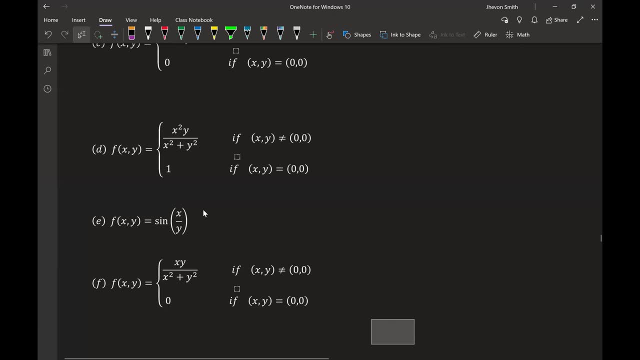 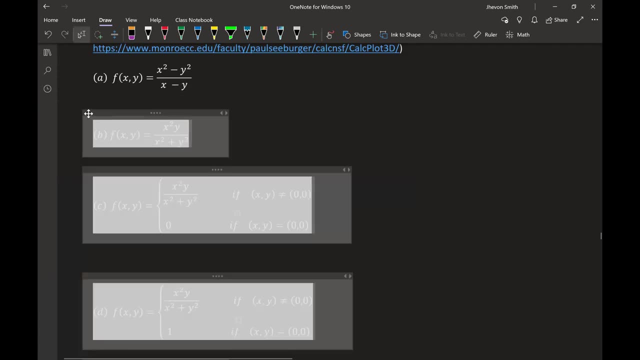 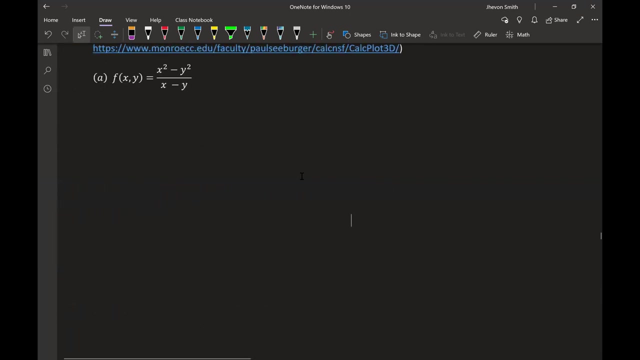 We have six examples here to get through, So let's actually do that, And I'm going to do visualizations For about three of them. So there are a bunch of online calculators that you can use to plot three dimensional graphs, and here are two of them that I will be using. 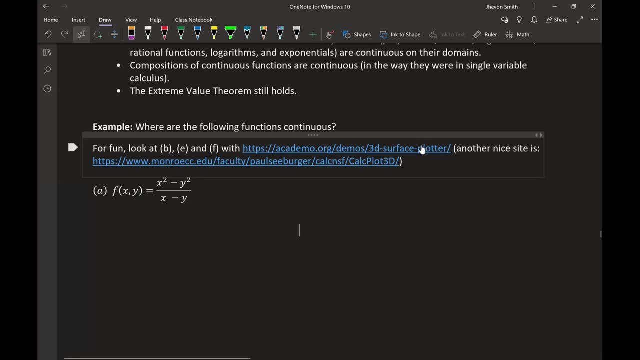 Probably most, mostly the first one, because I think, when it comes to still pictures, this one would look nicer, But when it comes to like a moving picture, that one is nicer, So we'll actually look at these. So let's actually jump in and talk about this. 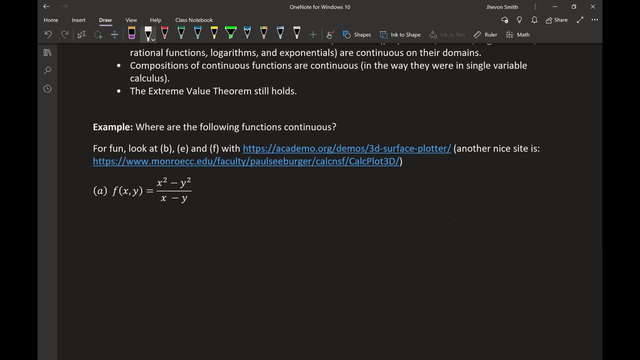 Here's a given function, a. tell me where it is continuous, So go take it away. Someone tell me where this is continuous. Right X naught, equals y, So it's a fraction. So for continuity it would be, I mean. 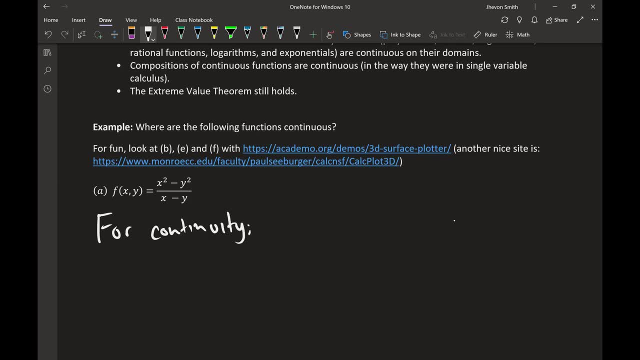 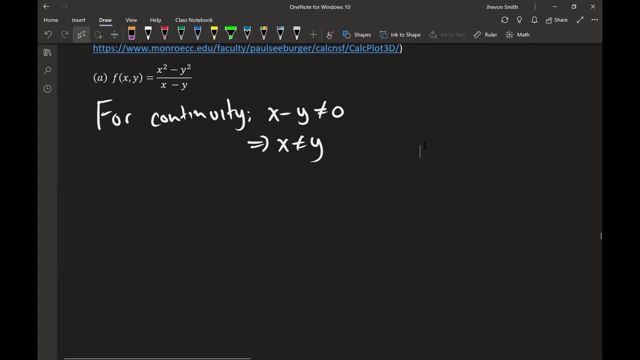 all right, it would be xС, and so we need X minus Y to not be zero. So this means X cannot be Y, And other than that, the numerator and denominator are polynomial, So individually the numerator and denominator don't have any other problems themselves. 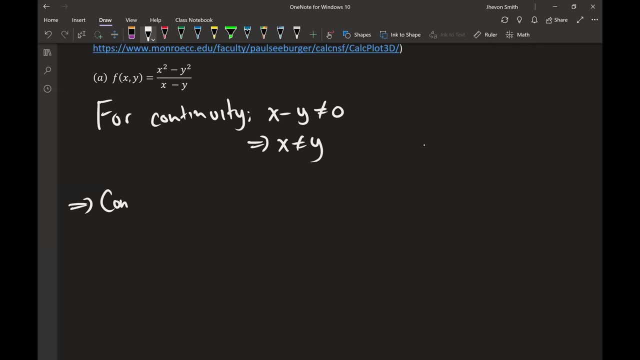 And so, yeah, pretty much, you can basically say it's continuous on the set of all coordinates, such that X is not equal to zero Right, which means that X is not equal to Y. And of course you should have the intuition. 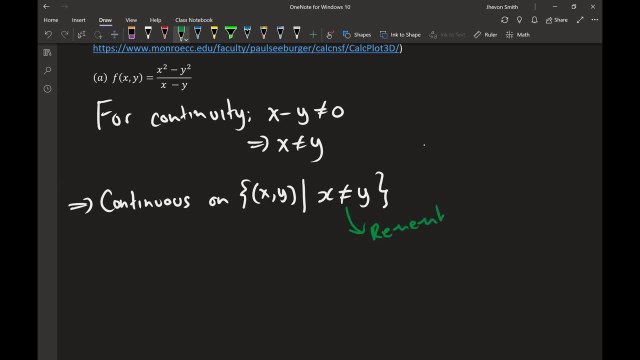 Remember: X equals Y is a plane, So I don't want you to think that this is just on a line. It's literally the entire plane: X equals Y. You cannot touch that part of this function. Okay Now, as long as you're not at that point. 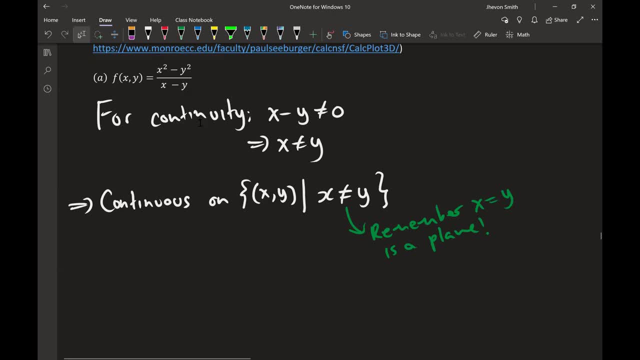 you can use difference of scores to simplify this guy. This guy is going to behave just like X plus Y would behave, except when you're on the plane X equals Y. it will not work, It will just have like a gap. So the plane X equals Y is like a huge gap. 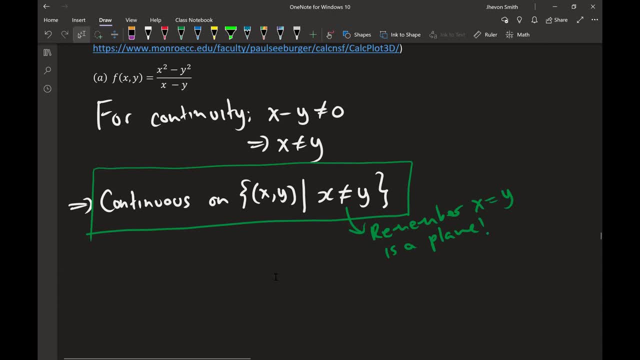 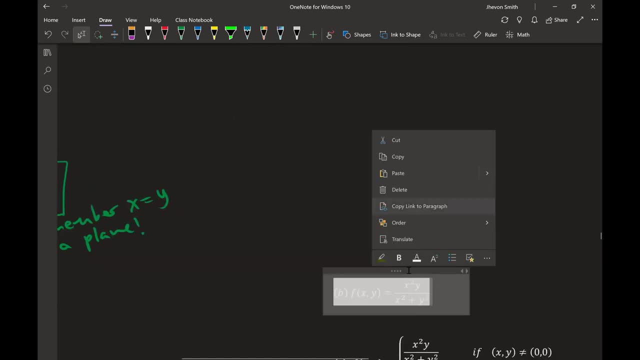 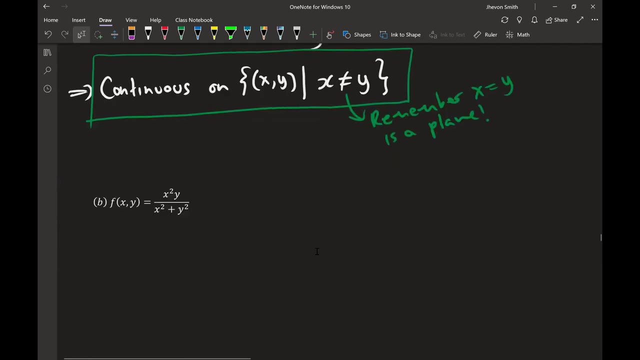 running through this function, It's not gonna work, Other than that it behaves like the plane. Z equals X plus Y. So, Yeah, that example wasn't so bad. Now I'm gonna sketch it. What about this guy? So you might have recalled this guy. 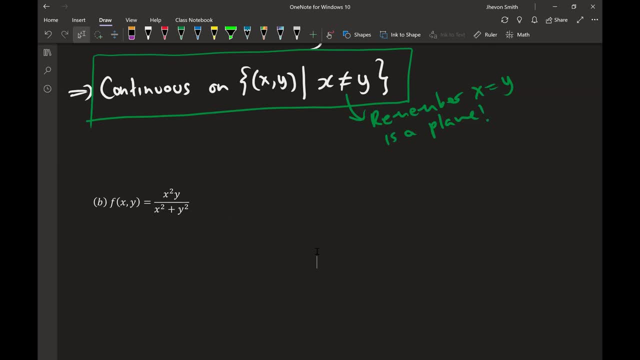 This was the guy whose limit actually existed. but we didn't know that in the beginning And we just kind of started to go through a bunch of paths and we kept getting zero. And then, you know, Abdulrahman was fooling us the whole time. 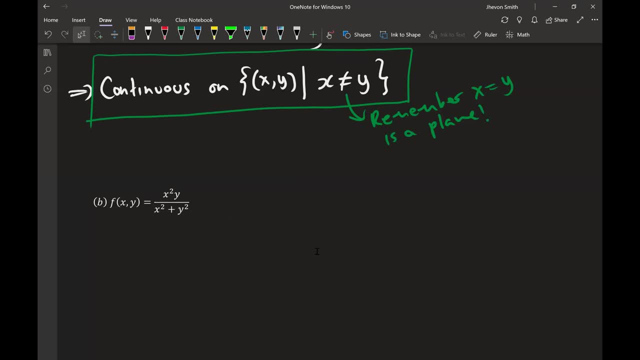 It actually existed, but he never told us. And then he just started. He started laughing at us at the end of the day. OK, So that's this guy. Where is this guy? continues. So for continuity. what do we need here? 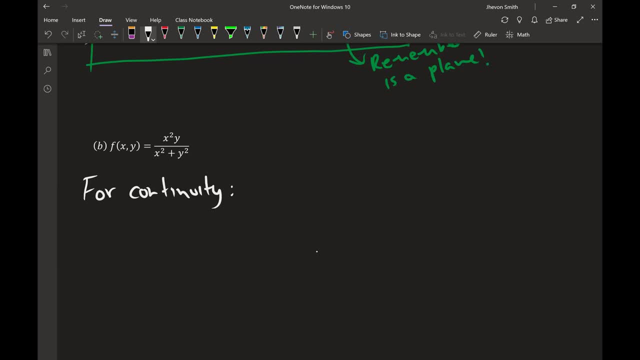 Nobody knows right. So just let's go through these steps all together: check, celebrate and figure out why we actually know about this guy or we forget where those guys came from or where they came up with that. But I want you to recall something. 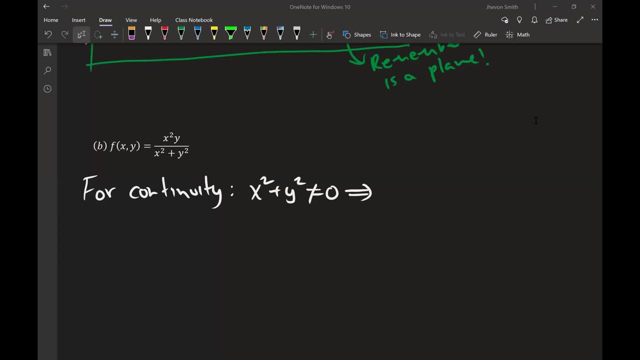 So let me just give you another example. sounds like x is what I said. You don't really need to remember why they came up with that, And let me use this example right here, to zero. so basically it gave me infinite many things, many points, except as long. 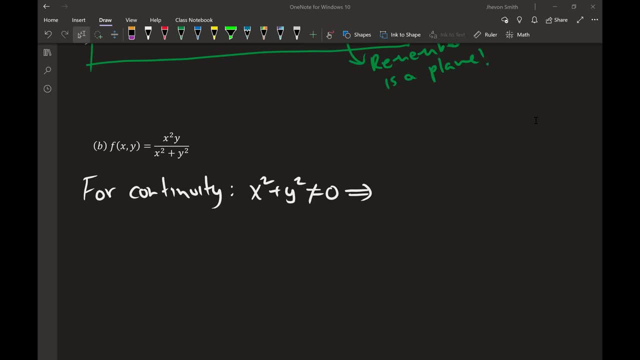 as it does. it does not equal to zero. that's all that matters. okay, tell me where it would equal to zero. or would it equal to zero if the X equals to zero or Y equals to zero? but however, as long as X square plus Y square in the 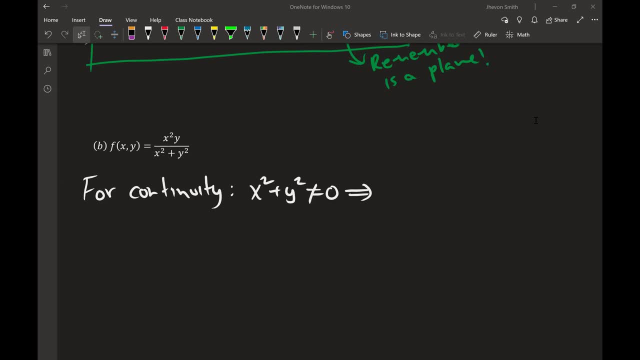 denominator does not equal to zero. that's all that matters, unless it's like it. that's all that matters only if the one of the variables of X is zero, or if Y equals five, or if X equals five or Y equals zero. therefore, it would be like: 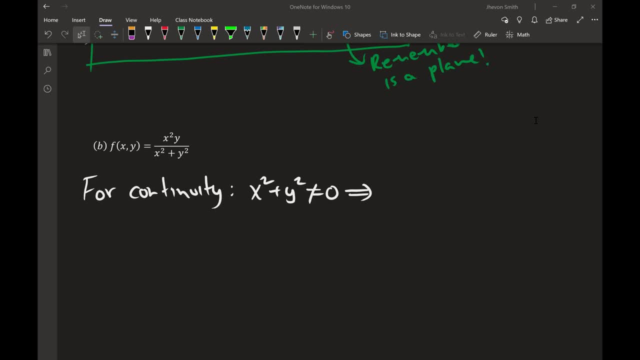 simplify, like: tell me specifically where, where would it be the case? where would X square plus Y square be equal to zero? notice, it's literally one square in the entirety of three space. right, you literally cannot be zero. at the same time, one or the other can be zero, except once one of them is zero, the other guy. 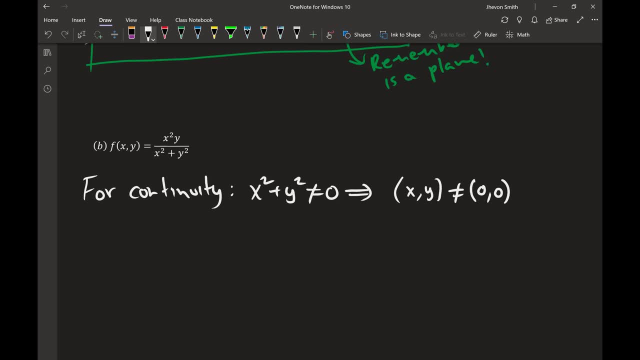 can't be zero. literally, the only time the sum of squares is going to be zero is when both squares are zero. so, literally, the only thing that we're not allowed to touch in this function is the origin. so this is continuous on well, our three, except at the origin. or you can say something like it's continuous on IE. 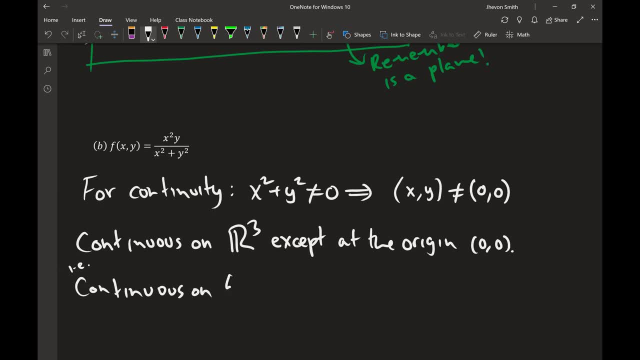 continuous on the set. I don't know what's with me and my set brackets today, set X comma Y, such that X comma Y is not the origin specifically. there's literally only one spot actually where this is going to be a problem, which means other than that, that one. 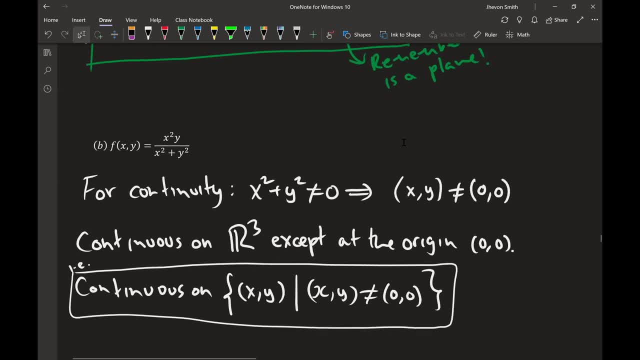 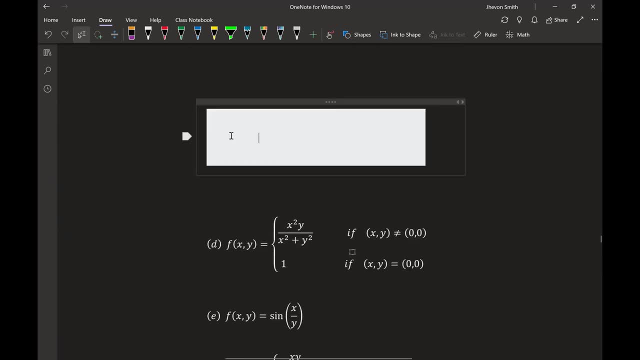 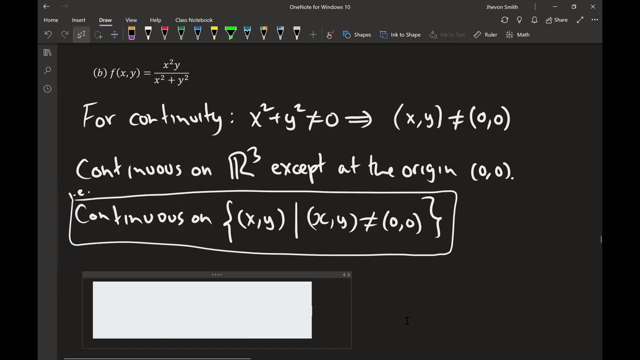 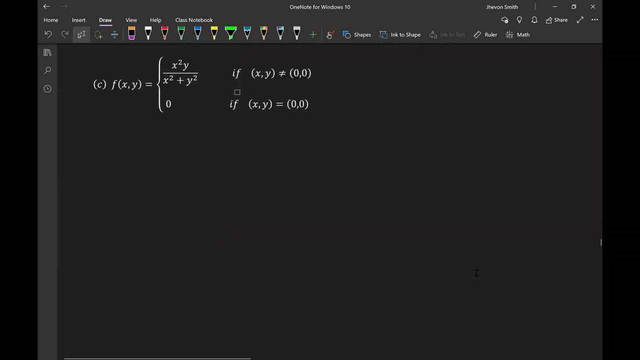 spot. this thing actually looks pretty nice. okay, what if I gave you this function, which notice that it starts out looking like the same function. where's that continues? so you, you, you, you, you. So this one is a little bit more detailed: Negative infinity. negative infinity over infinity. 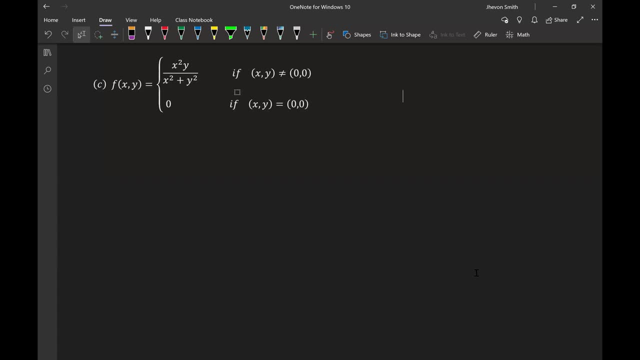 As in negative infinity over infinity. is that what you just said? I mean common infinity, sorry. Okay, so negative infinity. common infinity is an interval. Is that what you want to say? It's continuous on some interval. Yes, Okay. 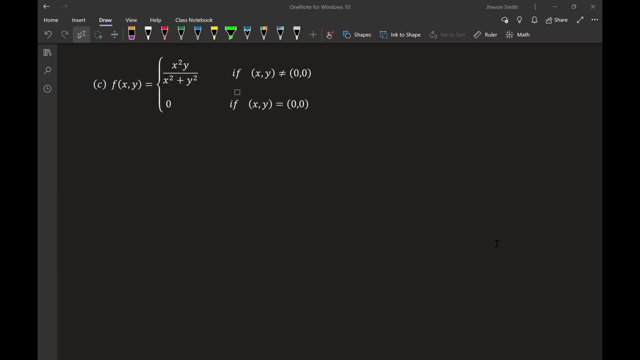 Okay, Okay, And which interval are you talking? Where's that? negative infinity to infinity going On the x-axis, On the y-axis? Okay, so this one isn't as clear-cut as the others because it's a piecewise function. 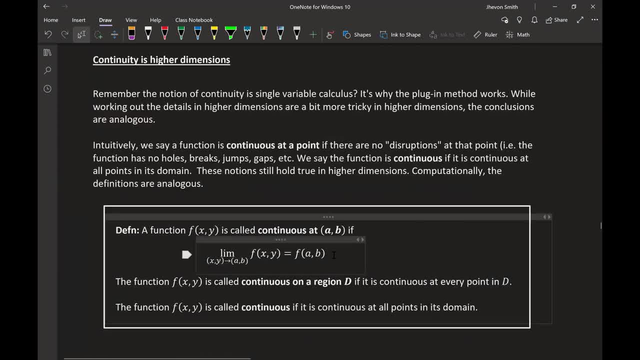 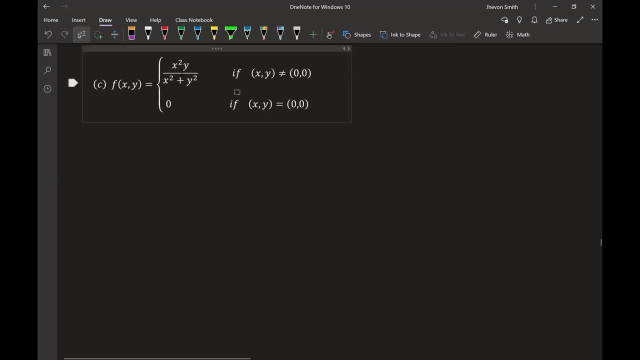 So for problems like this is where you really need the definition. This is what you need to check. okay, So to go over this, looking at this function, We have to just examine all the pieces. So on one hand, it's this guy. 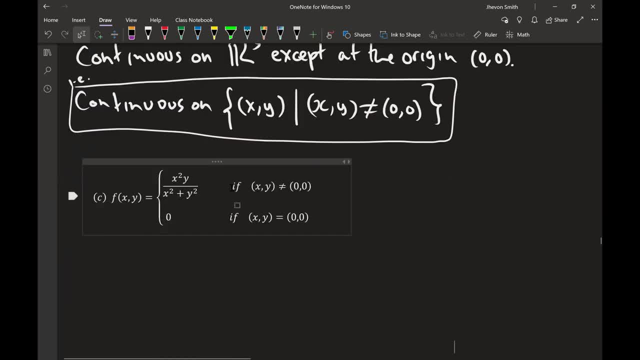 Now we already know that that guy doesn't work at the origin. but we're told that we're not at the origin when we're taking that definition. If you look in the first line, it's that guy, if we're not at the origin. 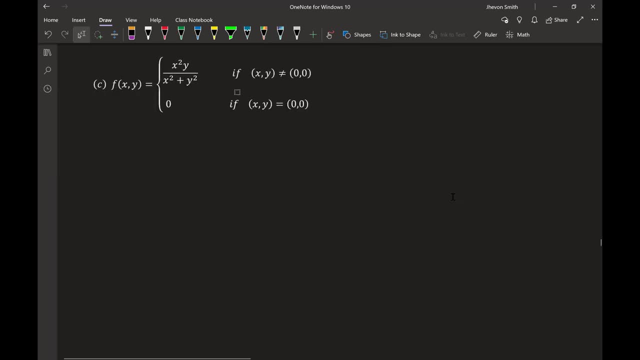 So actually, this guy is actually fine, right? So at this point you can notice here: if we're not at zero, zero, we're fine, Okay, Okay, Okay, Okay, Okay, Okay. So now let's check at zero zero. 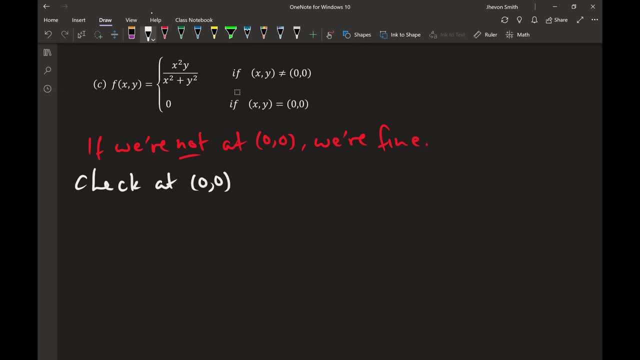 How would we know whether or not we're continuous at the origin? What would we have to check? Well, we'd have to check the definition. We'd have to check: does the limit as x, y approach zero, comma zero of our function equals? 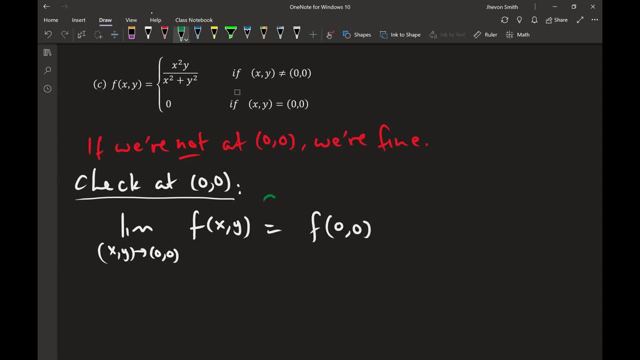 f of zero comma zero. Okay, if that is the case Now, this we actually found yesterday was zero, right? so this found last class. Now, if I didn't find it for you, of course you'd have to actually compute this limit which as of last class. hopefully you guys are all experts. 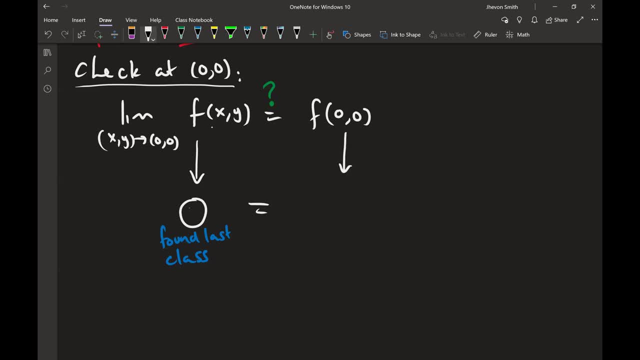 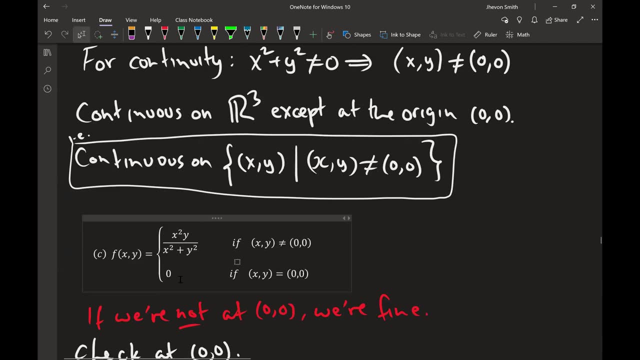 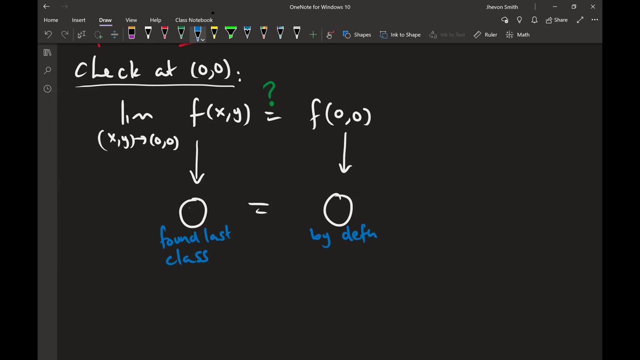 at that, and this guy here is actually equal to zero by definition of the function. If I look here, I'm given that if x comma y is zero, comma zero, it will be zero. So this here is zero by definition of the function, And so this would mean f. 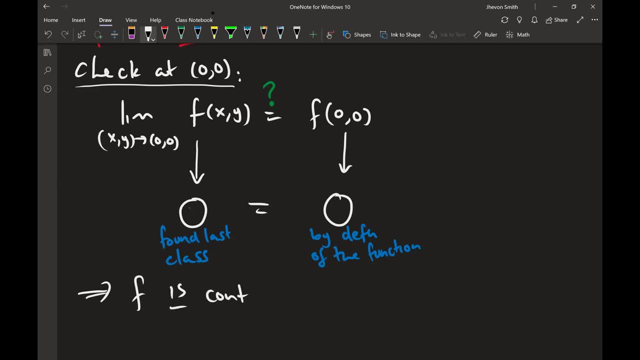 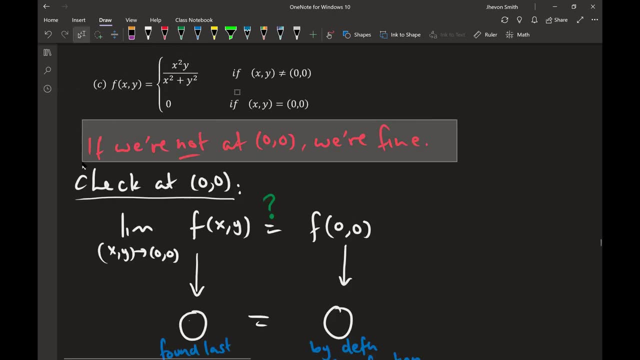 is continuous at zero. Now, since I know, if I'm not at zero, zero everything is okay, because I'm not divided by zero. I have a ratio of continuous functions and each of them individually behave, and I'm not divided by zero. so everything is fine, as long as 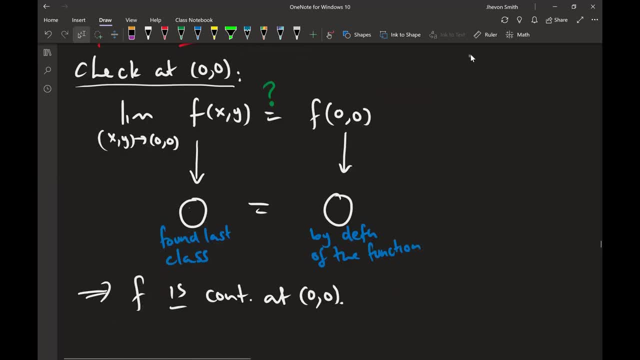 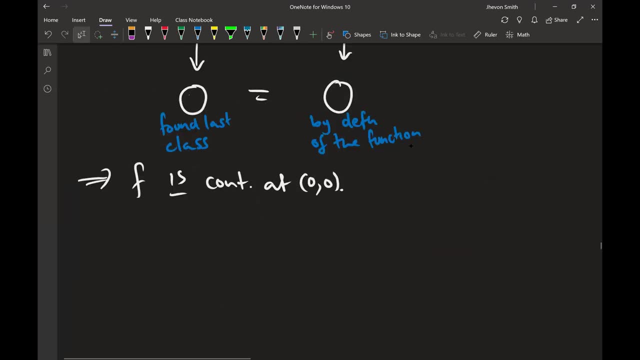 we're not at the origin, Then I go and I check the origin specifically, because this is only the potential bad point, but the limit checks out. and so here we can finally conclude: f is continuous Everywhere, and someone did mention this in the comments. but I want to know, I want. 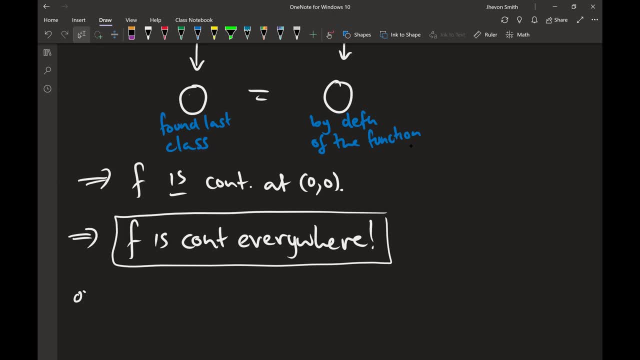 you guys to know where that reason actually came from. Or you can say something like f is continuous on all of r3 or something like that: Isn't it except the origin? No, it's also continuous at the origin. That's what that's literally. that's literally what I. 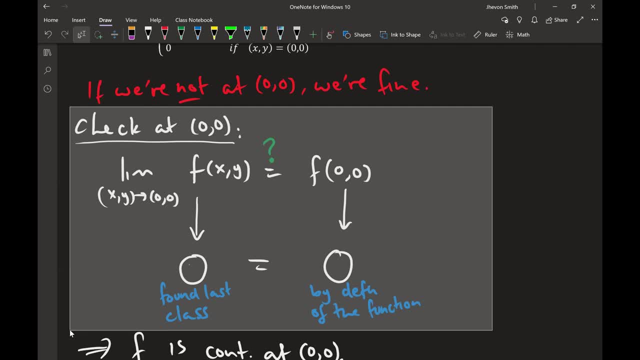 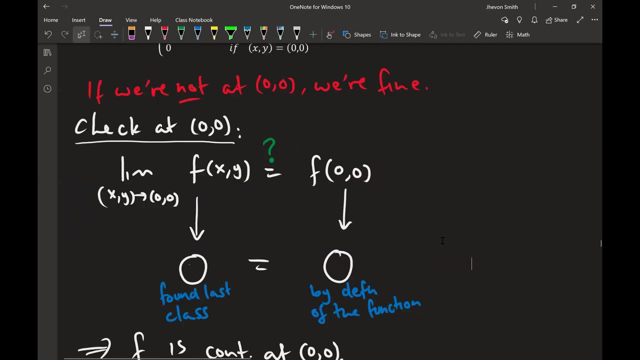 just proved. I checked at the origin and the definition of continuity works. The limit, as I approach the origin, is equal to the value of the function at the origin. Yeah, that part. but whenever it, when it came to x squared times y over x square plus y square, it didn't really work Well, that's because we didn't have this. 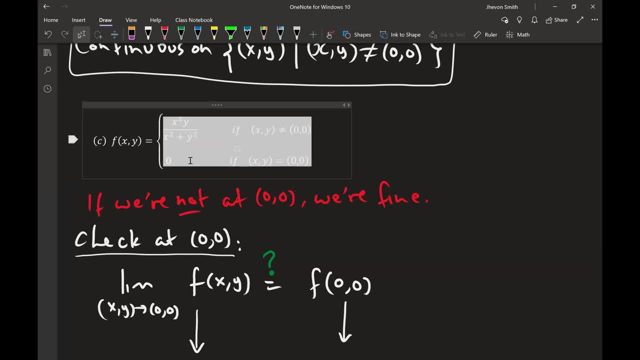 second line right, We put in a piecewise function. There's like a second line here right Where we're equal to zero. this line was added right, So the function is not the same as the last one. This one has just given us this part. 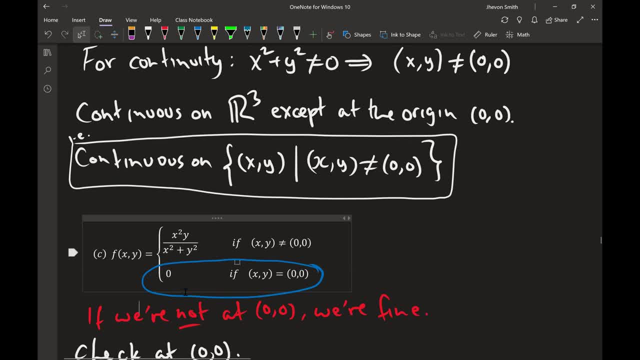 Here the function added, we added a piece to it. We said it's this definition if we're not at the origin and it's zero if we are at the origin. So this is some new information that we're given. Basically, this is like when someone comes in and 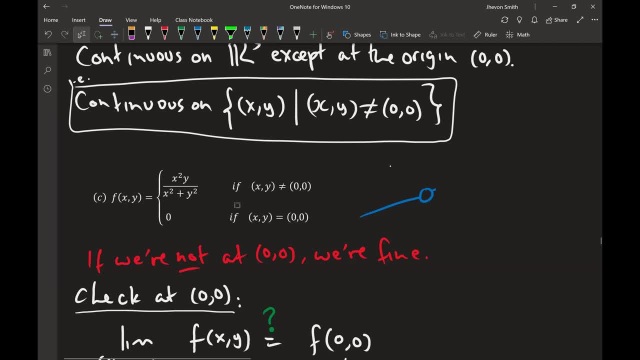 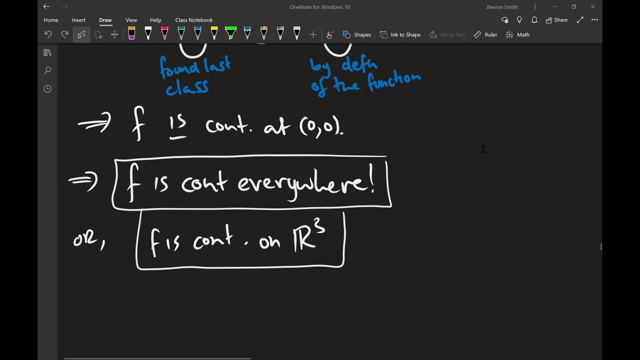 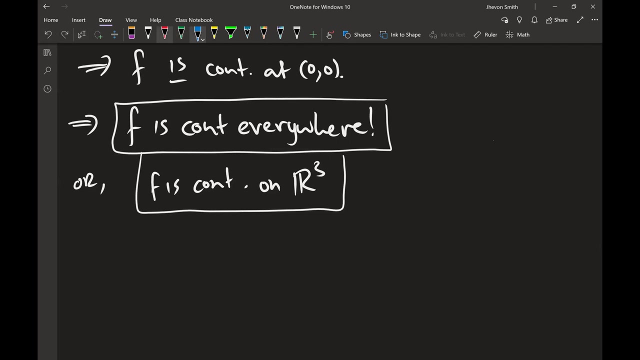 they see that a line has a hole in it and then they fill in the hole. So now it wasn't continuous before, but they made it continuous by adding some more information. What brackets notation You mean? something like In bracket notation you would say, f is continuous. on the set of all such 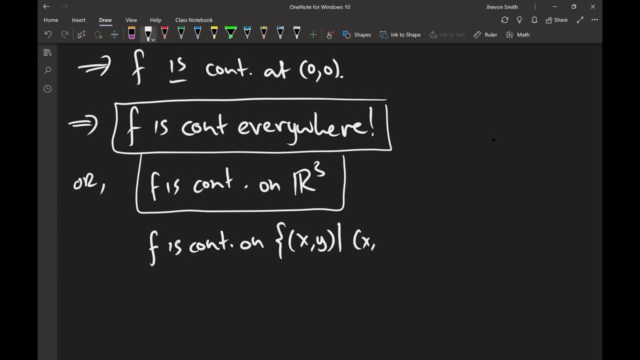 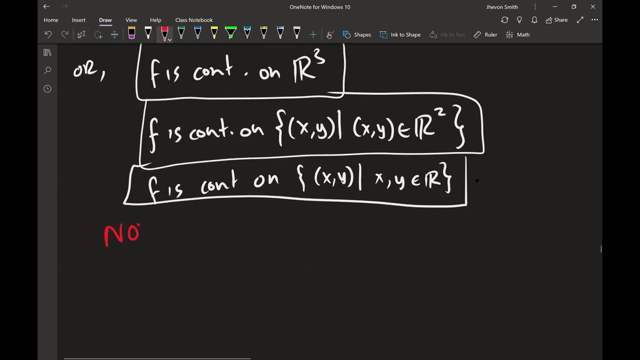 that is in R2.. So that's another way to say it. Another way to say it: f is continuous on x comma y, such that x and y are real numbers- Another way to say it. One thing you want to know that it's not correct. to say not correct is to say f is. 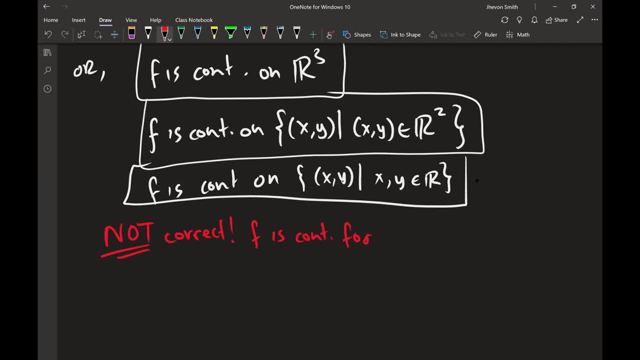 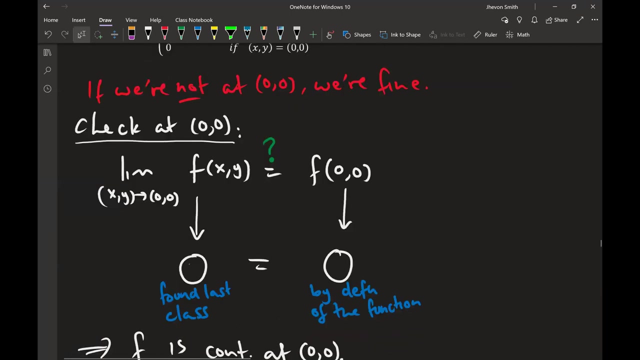 continuous for, like, negative infinity to infinity. That's not correct, because that guy is an interval, It's not a two-dimensional space. Now I want to actually show you guys what this guy actually looks like, And so what we're going to do is we're going to head over to 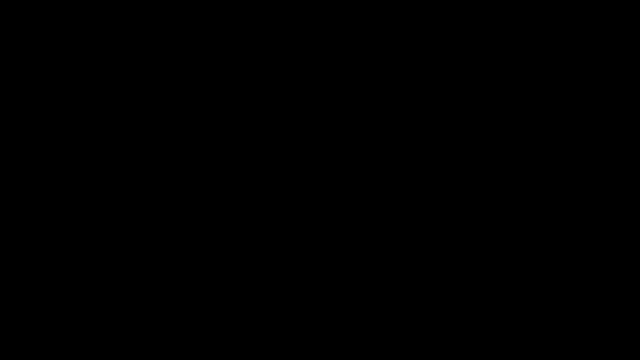 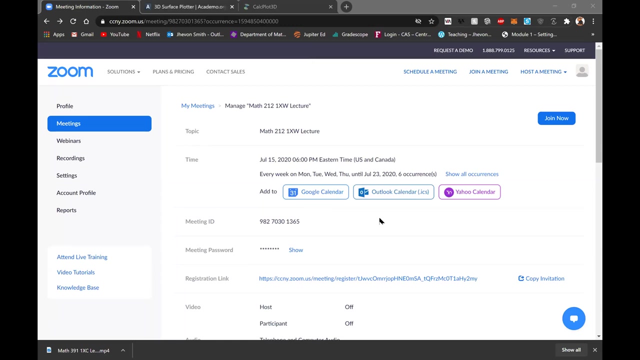 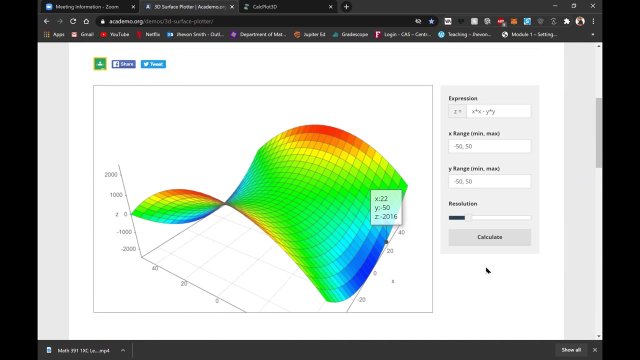 my browser, So there is the, the zoom chat. That's where the magic happens. Okay, So here is a plotter, a 3d plotter. The link is already in the in the notes. So this guy is our Pringles potato chip. This is the hyperbolic paraboloid. You. 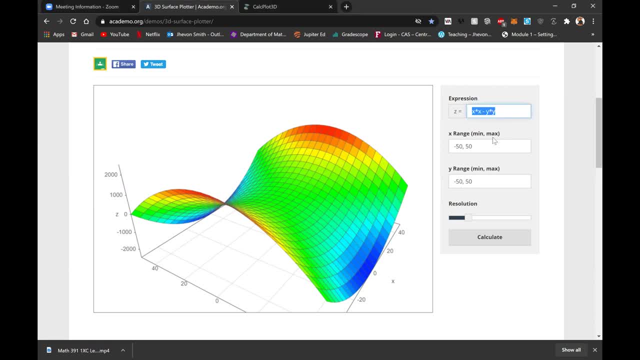 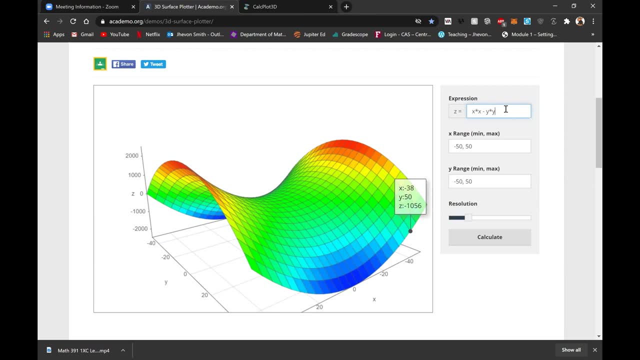 notice. here is the equation: x squared minus y squared. Looks like this guy. So now let's look at what the guy we were just looking at looks like. So this would be x squared times y divided by x squared plus y squared. So that's the guy. 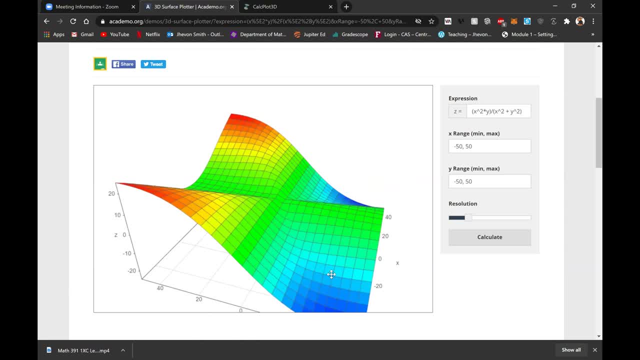 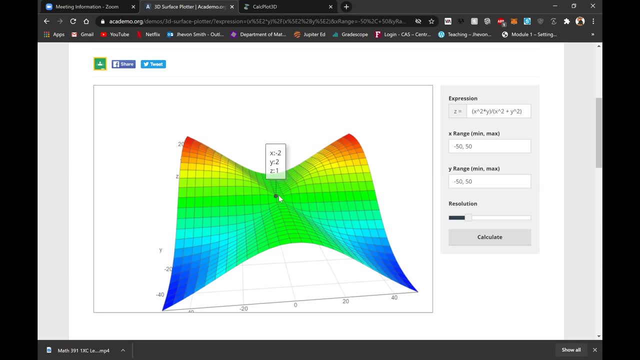 that we look like Now. he looks pretty nice, In fact, here. there you can see a little kink. The origin is like: right here, where my arrow is, There's a little kink. but you can't really see the problem from this, And so that's how we're. 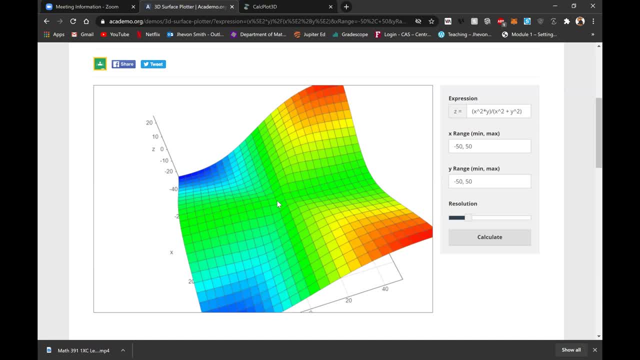 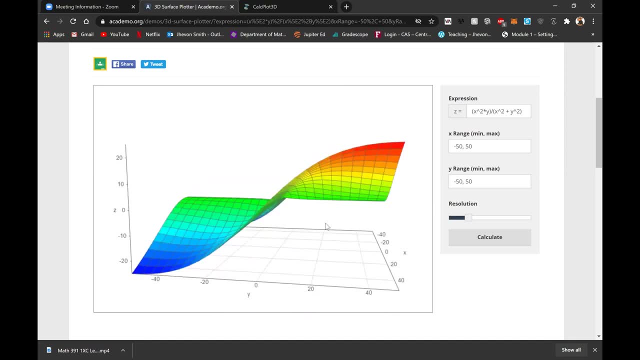 going to do it, but essentially there is an issue in the middle right here, but we filled in the issue, But literally it's only one point that's missing, so it's not gonna show up very well on this graph, but that's what the guy actually looks like. 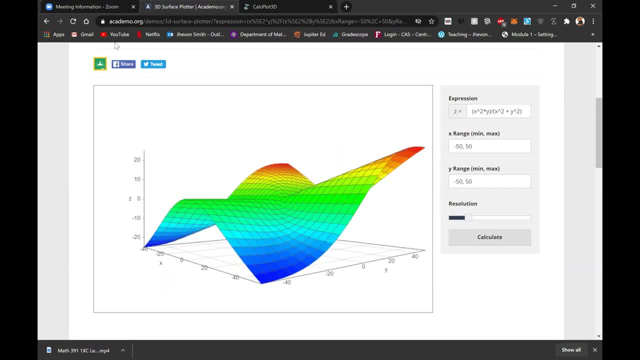 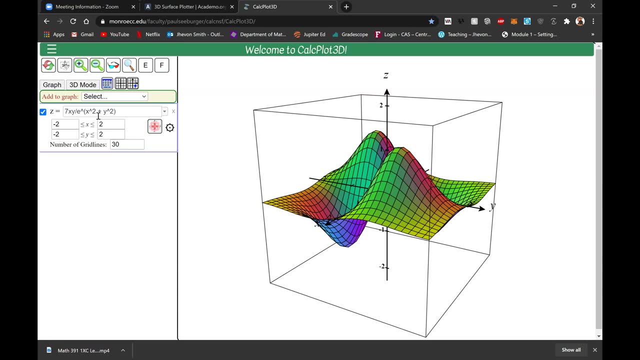 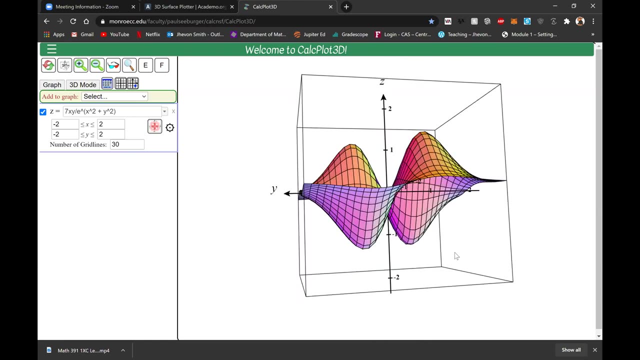 which is very nice, as you can see Another one. here's another one, And this is the function that you're looking at right. here is seven X, Y divided by E, raised to the X squared plus Y squared. it looks like this: See, this one can rotate. 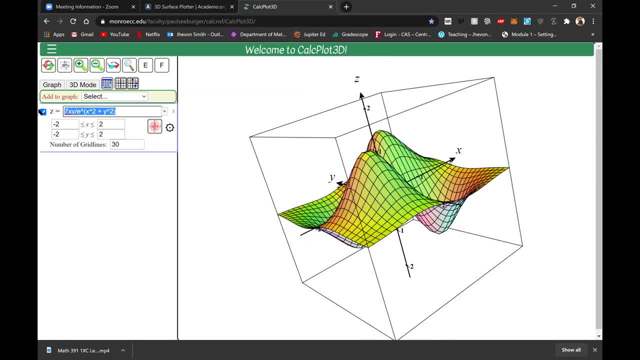 So you can look at all these guys that we were looking at earlier And if I put back our original function that we're looking at, X squared times, Y divided by X squared plus Y squared. there he goes. that's what the guy looks like. 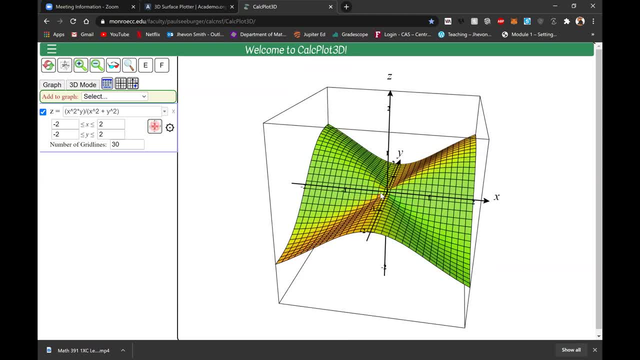 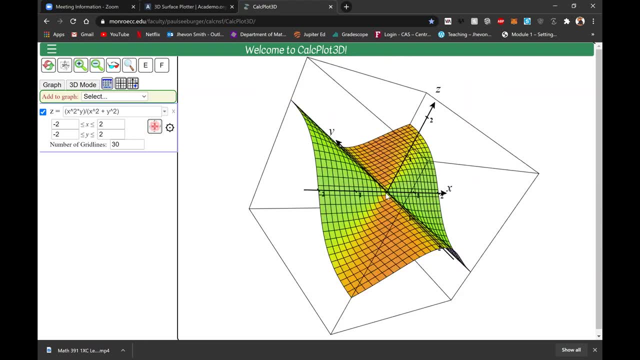 And at the origin. like I said, it's right there in the middle of that little kink. You're not going to like literally, it's literally one point that's missing. You're not going to be able to see it from this graph. 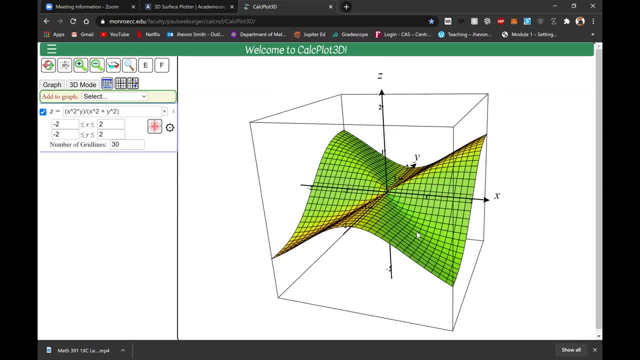 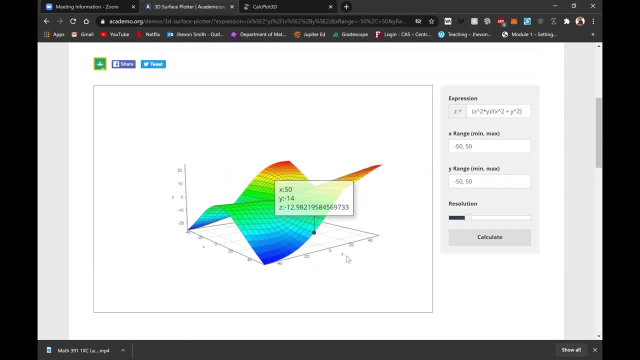 Later on I'm gonna show you some guys where you're definitely going to be able to see visually: Yep, this function definitely has a problem right there. No ambiguity, right? But this is our guy right here from the example that we're just doing. 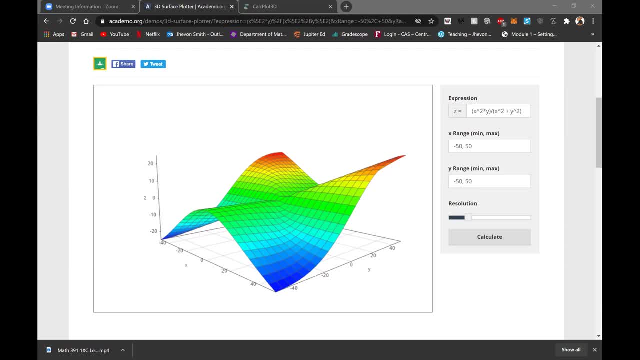 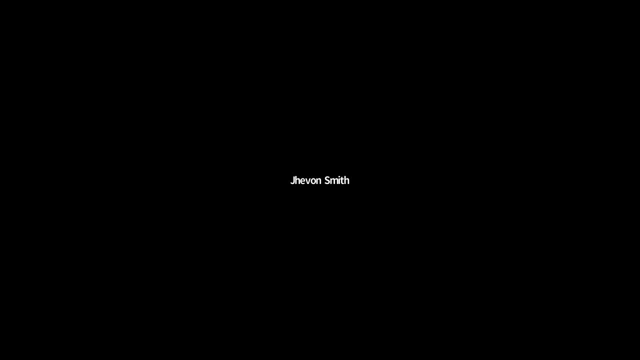 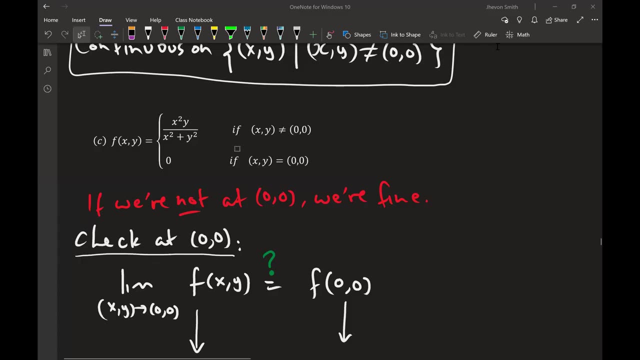 So let me right. so that's what it was looking like, And if you guys want to look at any of these functions that we're looking at yesterday or anything, you can go to that website and you can see it. So this is what that guy looks like. 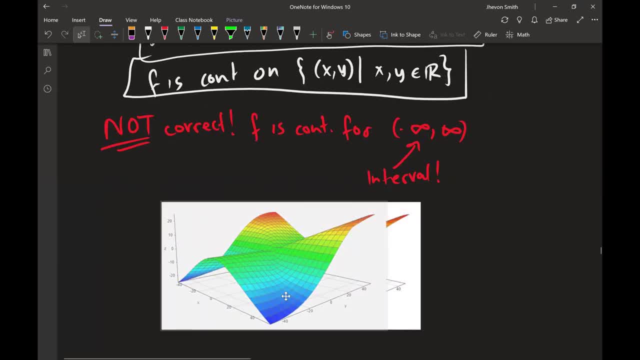 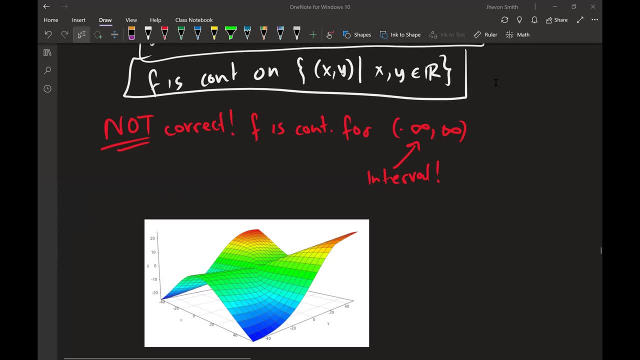 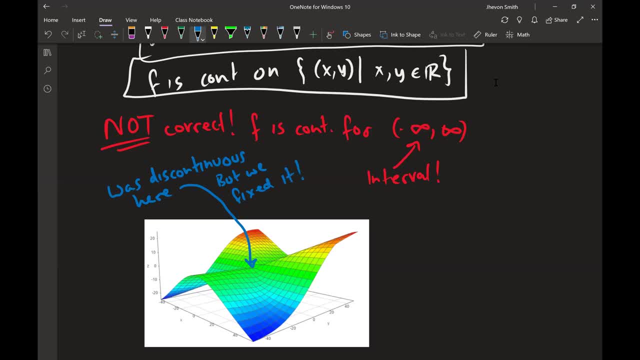 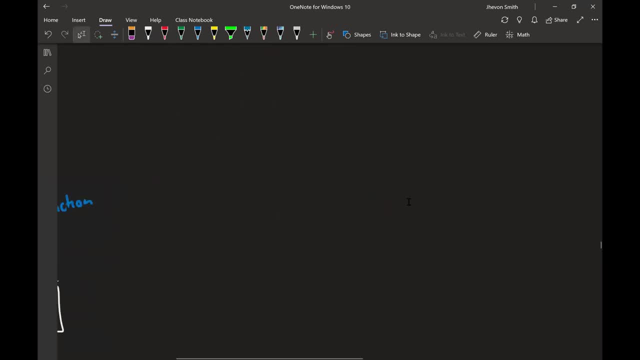 of a removable discontinuity, But that's, that's actually what we're looking at, So it's nice. All right, let's look at another example Now here, because I just wanted to give you another example where you would see that 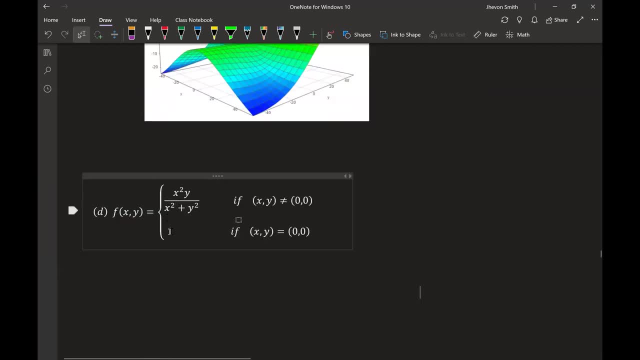 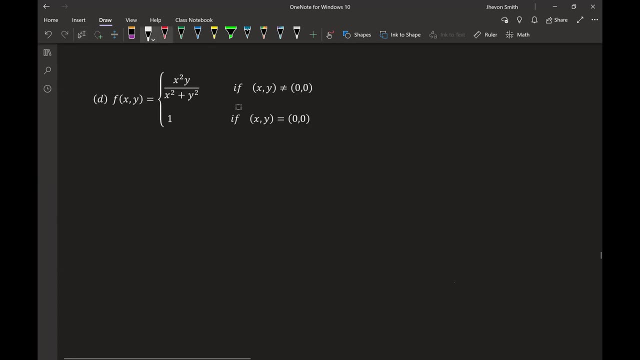 Again, it's the same guy essentially, but I modified the other part. Now down here is one. So let's pretend that this was the problem. you would actually approach it very similar. First, you will notice that if we're not at the origin, 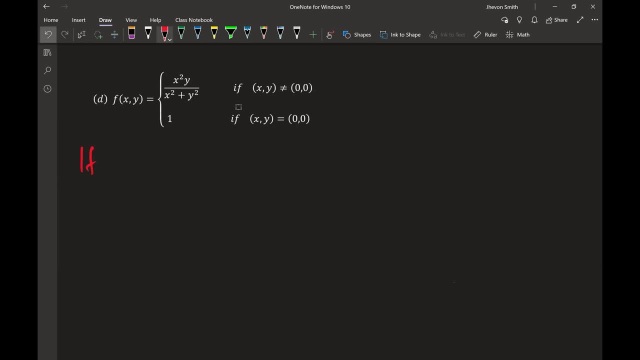 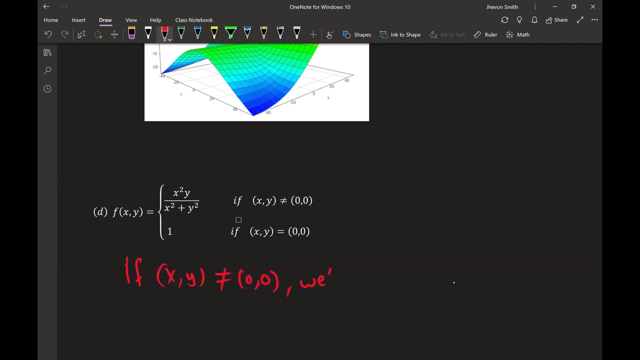 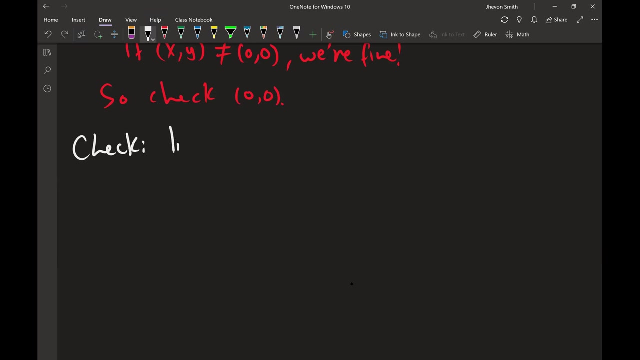 Or So if our x, y is not zero, zero, we're fine. So check Zero, zero. Now what you would do to check zero zero Is you would check is the limit as x comma y approaches zero comma zero of the function. 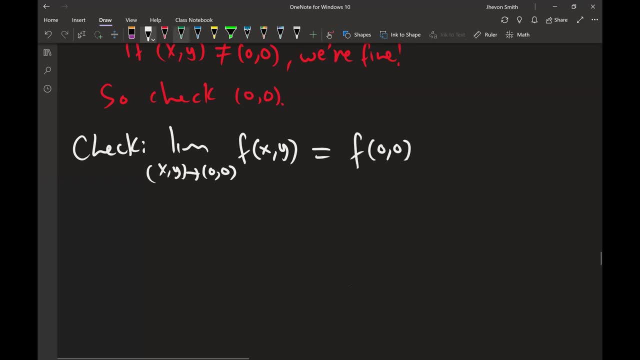 Equal to the value of the function at the point. right now we don't know if this is the case, So I put a question mark here Now. this one again, we know is zero from the previous class. This is one From the definition. 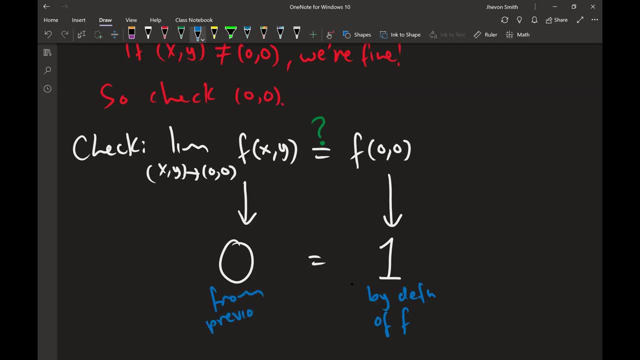 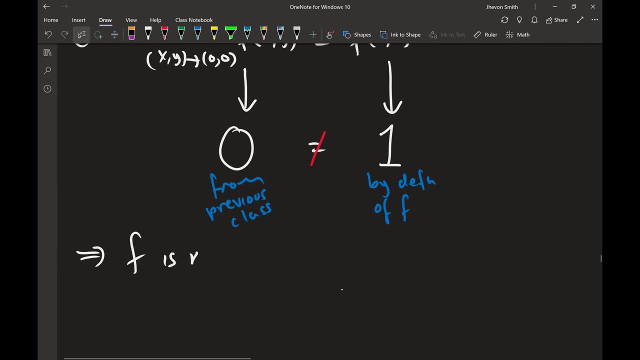 This from previous class. So now you'd realize that they're actually not equal. So at this point you can conclude: F is not continuous at the origin Meaning. now f is continuous on what the original guy was continuous on the very original before anything. 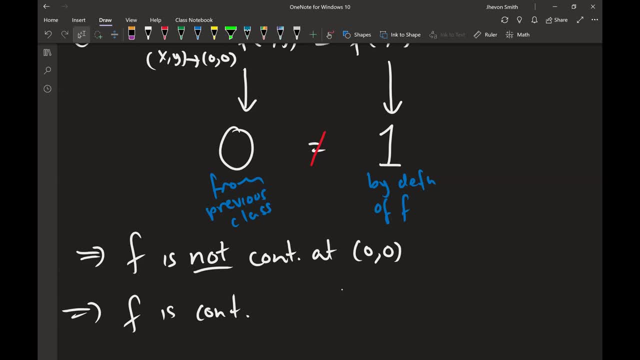 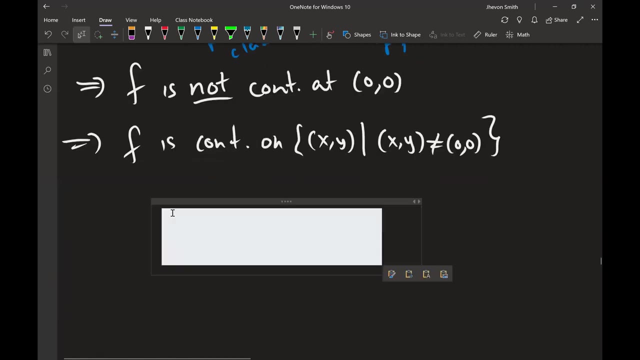 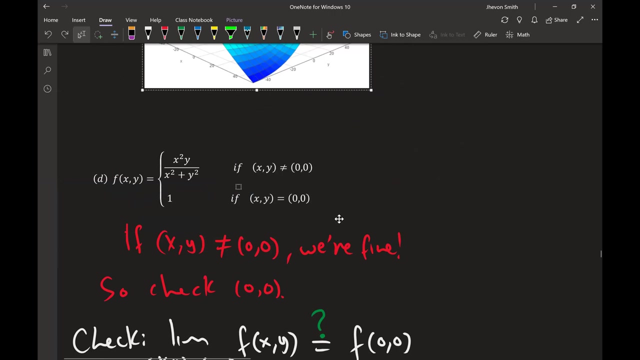 The set of all x comma y, such that x, y is not zero comma zero. So at this point it's like we had the guy. At this point it's like we have this guy, But we filled in the wrong point. 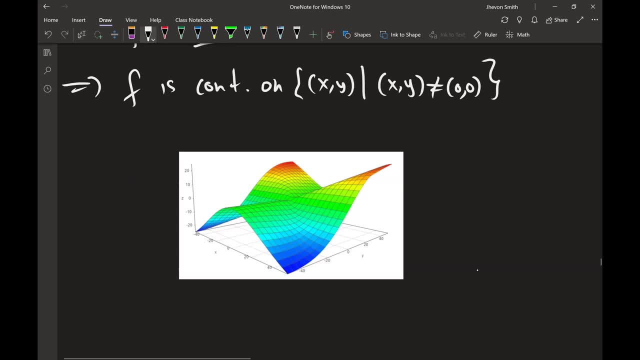 So it's like we have this, but we literally filled in Some point, hovering one unit above where it needs to be. We filled in this point, But the problem was down here, So now it's remains discontinuous at the origin. So some visual aids there. 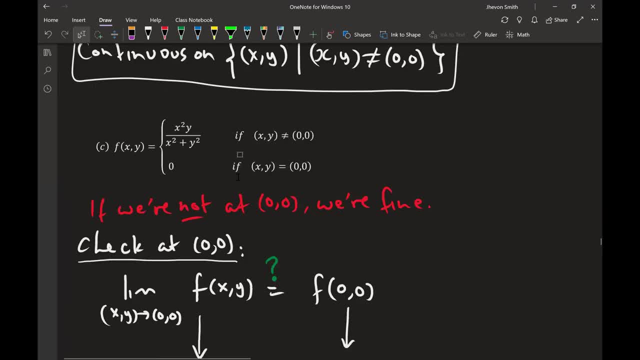 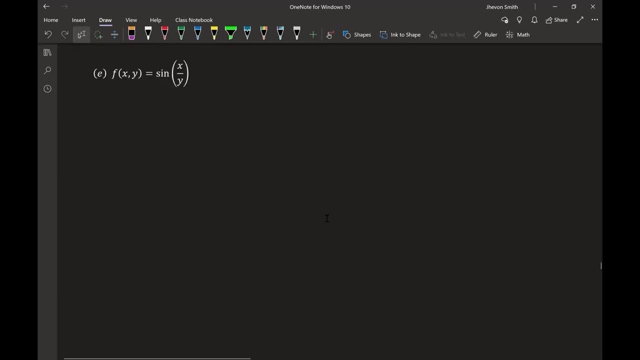 Look here This function. Okay, So Here's another function. And again Remember: composition of continuous functions are continuous functions. Divisions of continuous functions are continuous functions. So obviously here the issue is division by y For continuity. Why cannot be zero? 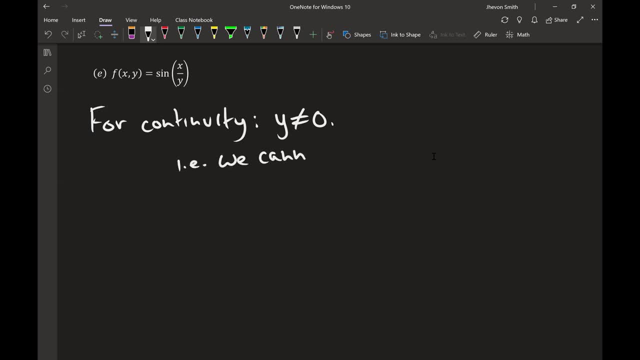 I E We cannot be on the plane Because you spent years of your life being ingrained that y equals zero is a line. So every opportunity I get after remind you that y equals zero is actually a plane. So literally on the entire exit plane. 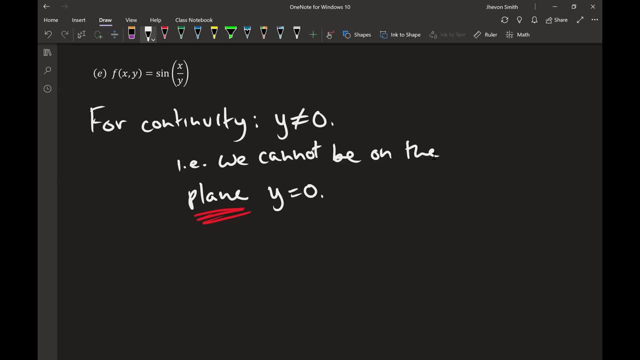 This function cannot exist. It's it's. It has disruptions along that entire plane. So F is continuous At x equals zero and y does not equal to zero On x comma y, such that Just y not equal to zero. Now 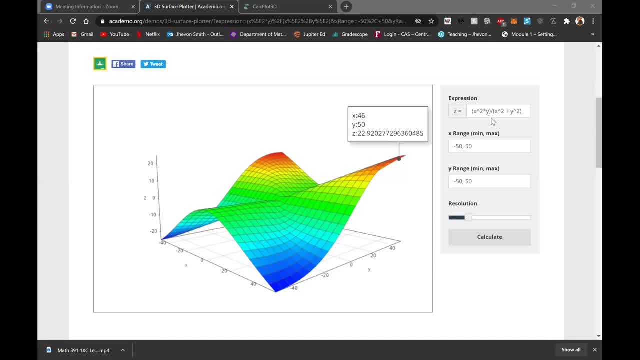 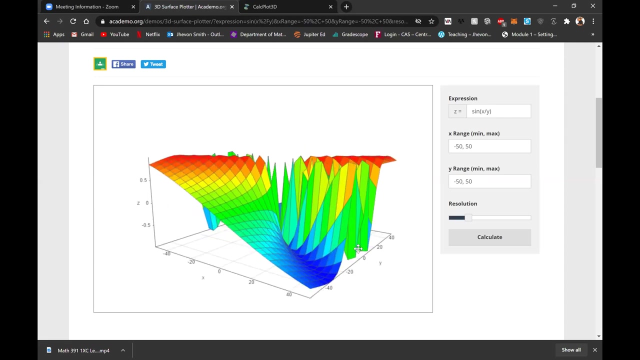 If we go back To this guy, Let's type that guy in. It was the sign of X divided by y. Now look at that. Notice what, where all this thing is going, Notice where all this disruption in the middle is. 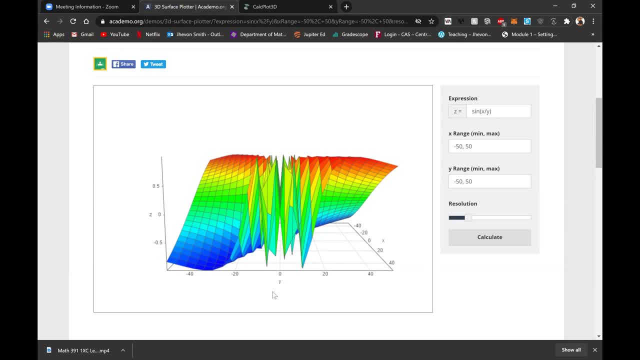 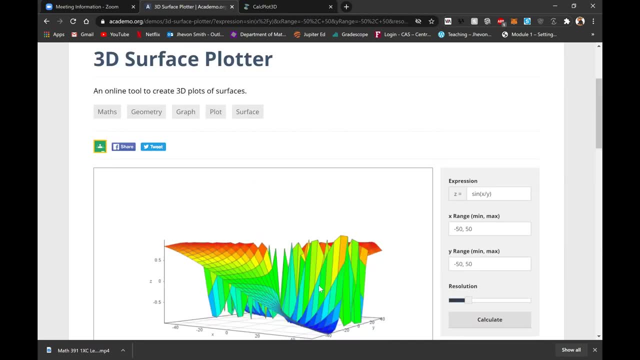 Here's the y axis here. Here's where y equals zero, right here. Literally, going through there, Through that path, Is No bueno, Right. The farther we get from zero, the nicer this thing starts to look. But look at what happens. 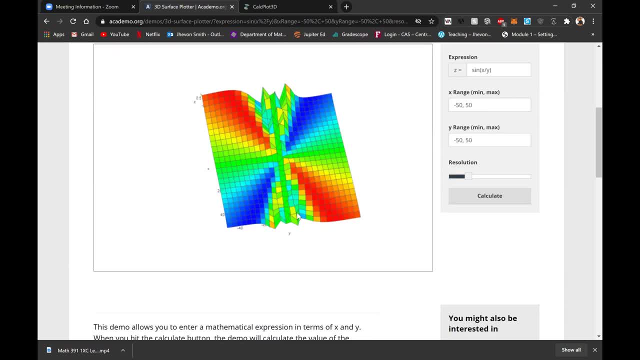 When we are Lining up With. This is literally the, the- the Y equals zero- line. right here is where the disruptions are happening. So that's our picture. You see that the function starts getting crazy Once you start getting close to division by zero. 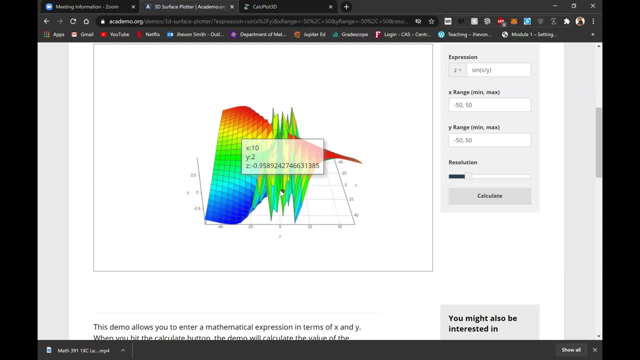 And then it's a sign function. So it starts oscillating like crazy, But then it can't actually settle at a value. Okay, So that's, that's the guy right here. It's a. It's a very, very crazy looking function. 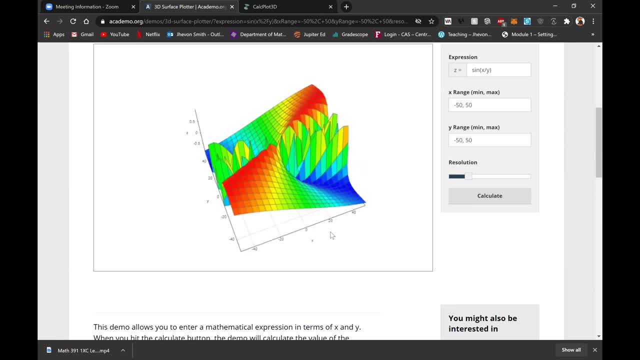 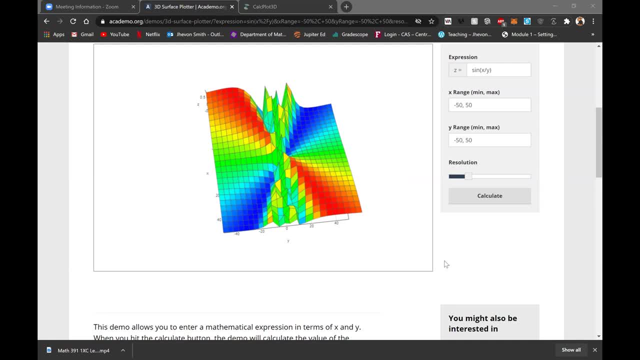 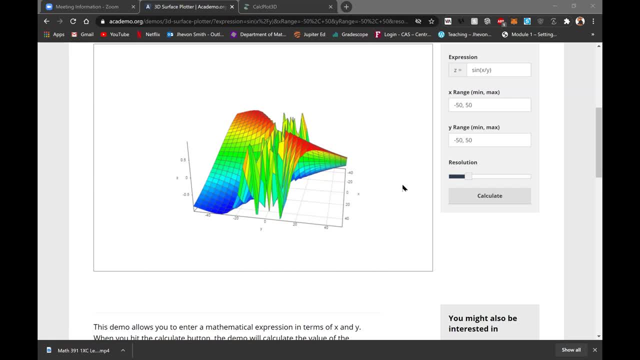 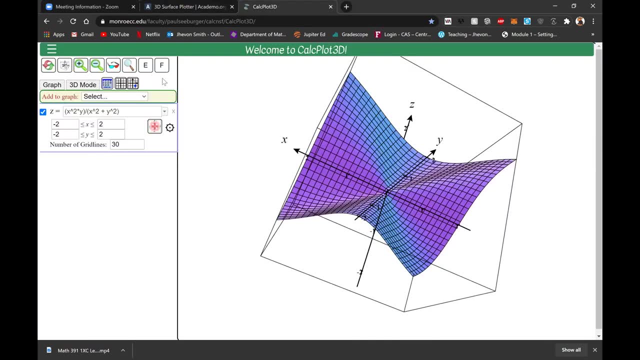 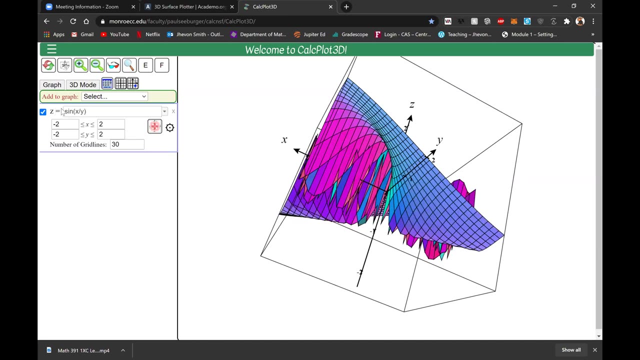 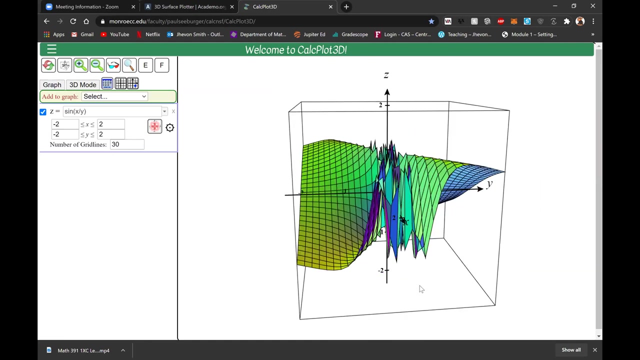 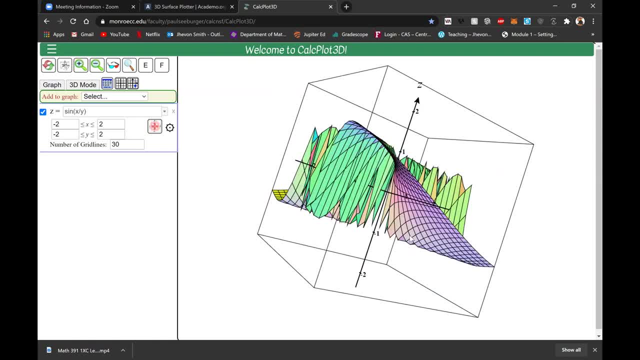 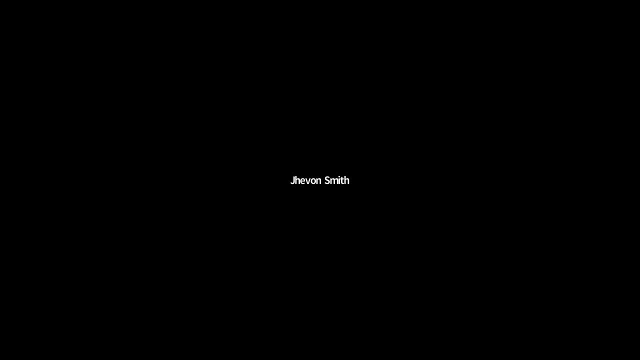 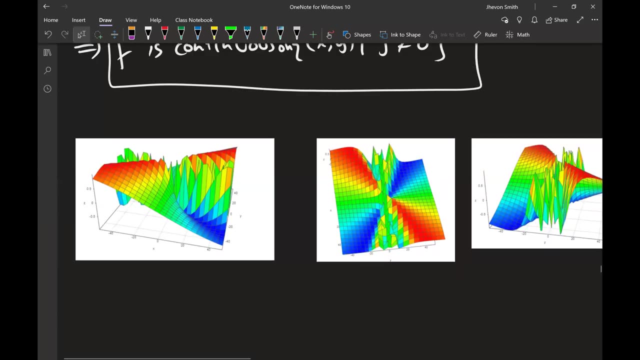 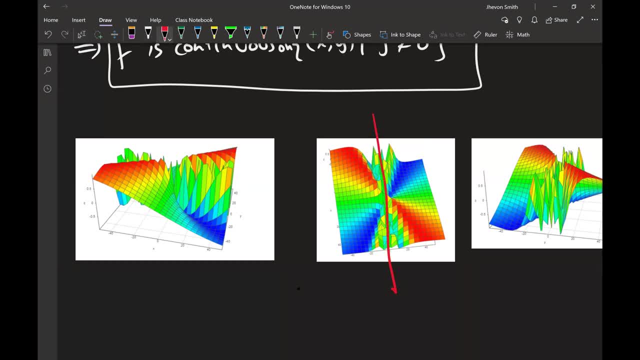 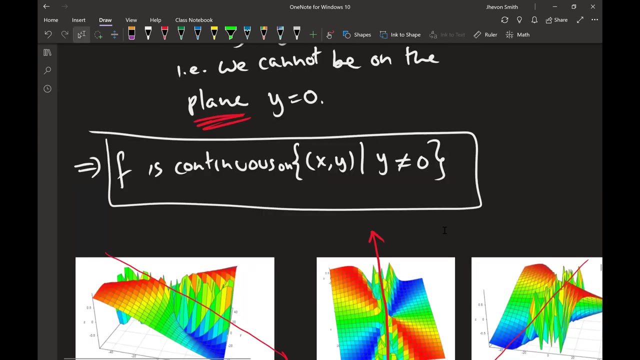 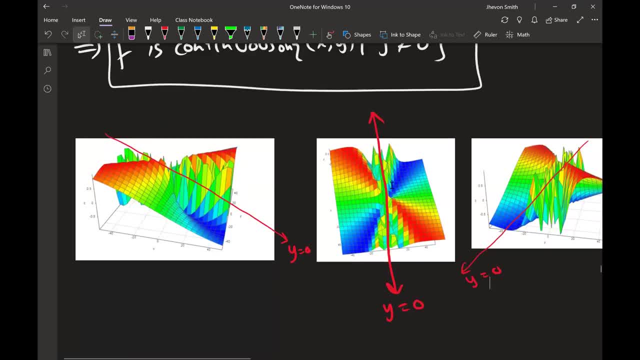 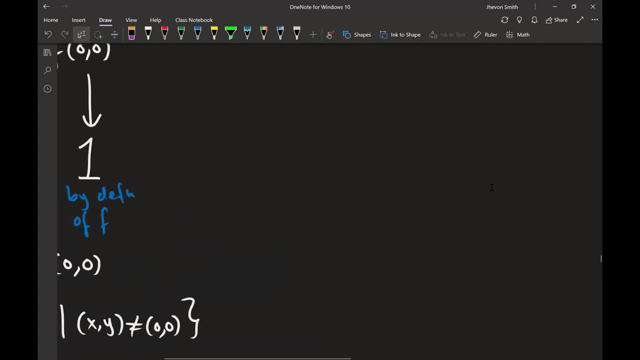 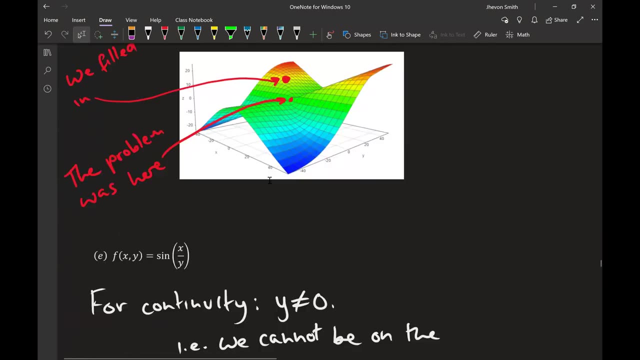 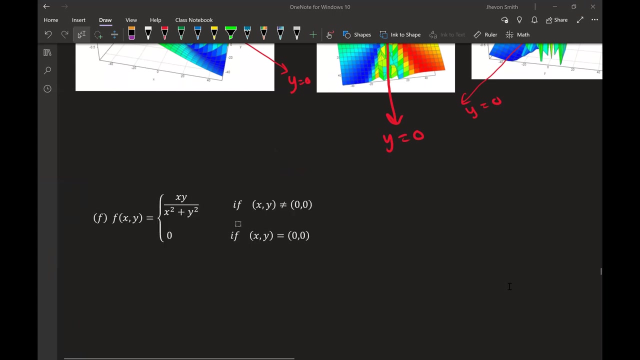 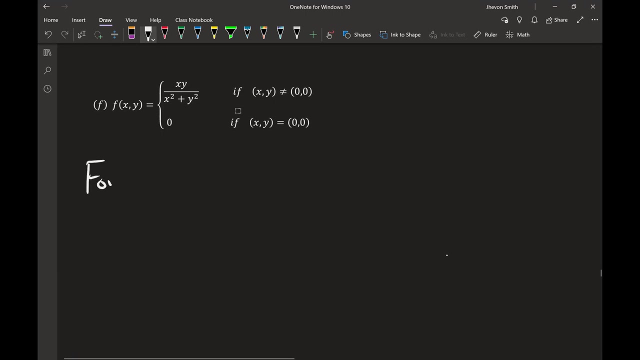 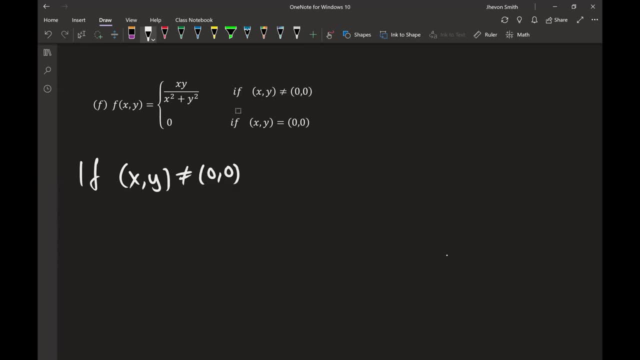 So now I go and I check at 0, 0.. So now I want to check: does the limit, as I approach the origin f of x equals the value of the function at the origin? Now the value of the function that is given? we're told it's 0. 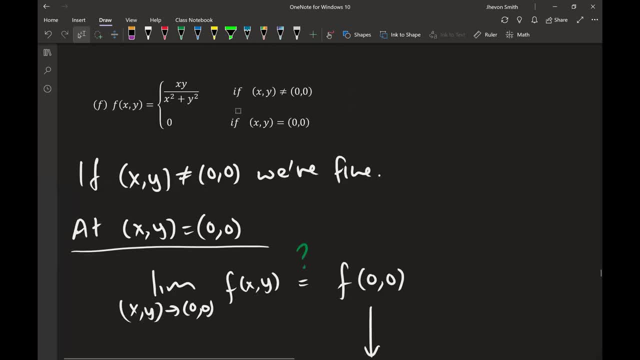 What is this limit? What is the limit as x? y approaches 0 of this guy? Are you sure it's 0?? I mean answer quickly, but not too quickly. Oh, so now you're just guessing 1? Is that what we're doing? 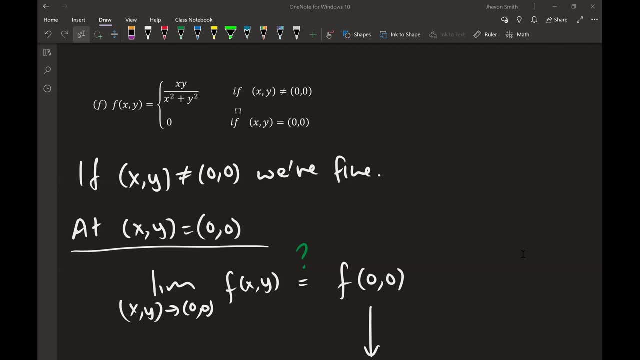 We're throwing out random numbers now. How did you get 1?? How did you get 0?? Minus pi. I vote for minus pi. E to the pi. maybe Remember your training grasshoppers? Examine that limit. 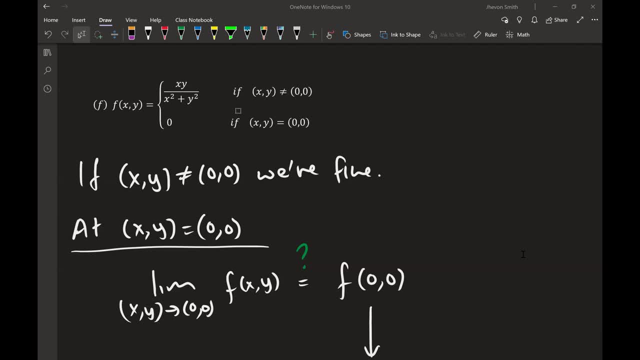 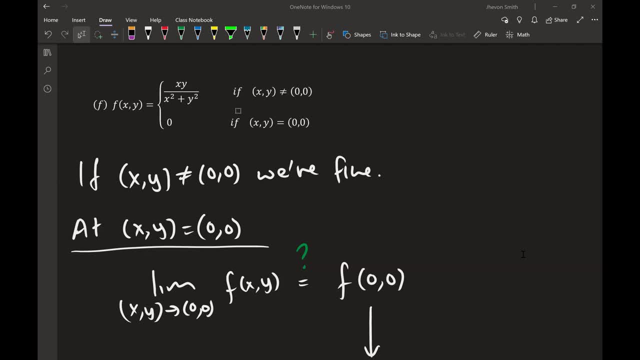 None of the above: Yup, that would have been on the test. None of the above: I select choice F. This isn't a trick. In fact, we actually did this problem before, so it's literally not a trick. You've literally seen it before. It was one of the examples we did yesterday. 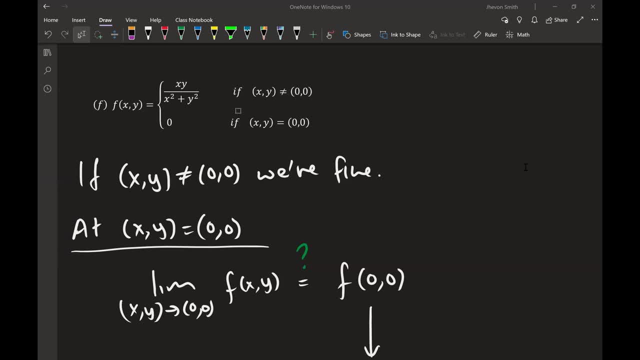 Well, don't look at what we did yesterday. You're supposed to be looking at that right now. take it at its face value and then evaluate it. Don't look back at what we did yesterday. Try to figure it out. You're supposed to question everything. 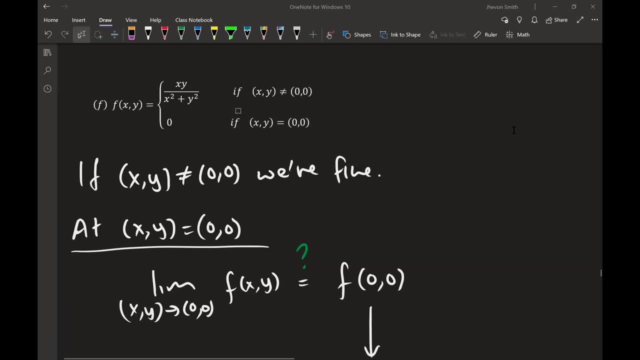 Of course, don't go overboard with it, Jason. what do you think? Mm-hmm? Well, what I would say is that it's not a trick. You're supposed to look at what we did yesterday and say: as long as we're not in the origin, we're fine. If that's what. 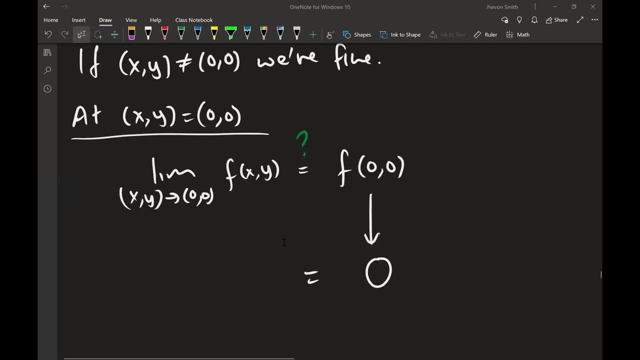 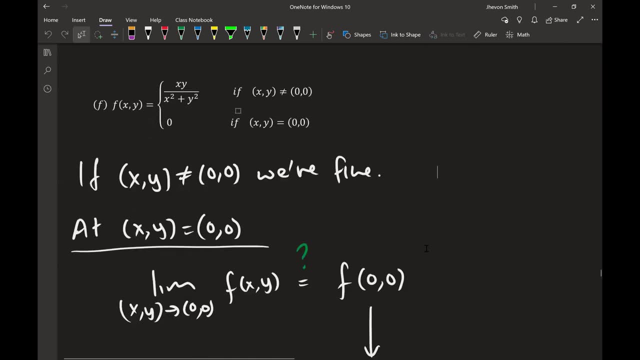 you think if X, Y- No, I mean this. The question is, what is the limit as X, Y approaches 0, 0 of this thing? 0, 0?? I mean, it would just be infinity, infinity over infinity, That. 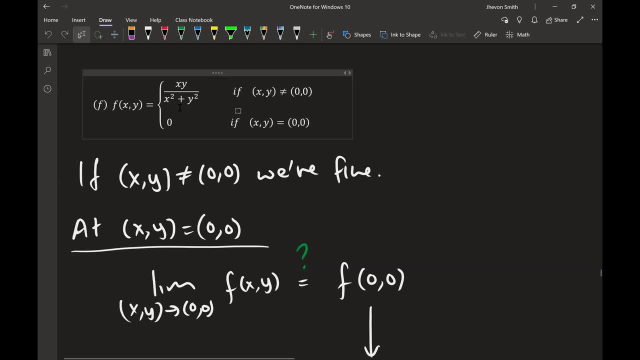 would be an indeterminate form. That's what I would be. Well, it would go to 0 over 0, but no, that's not how you examine limits. 0 over 0 is indeterminate. You can't say anything from 0.. 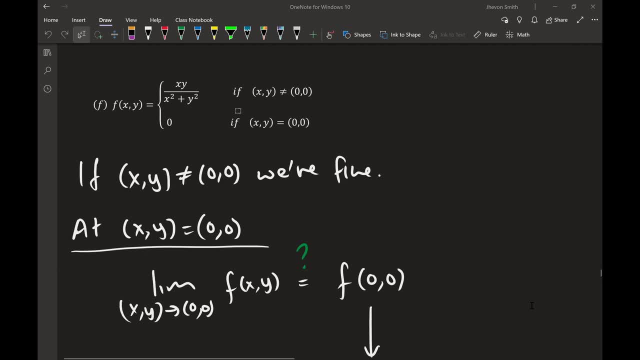 0 over 0.. Yeah, like I said, it's an indeterminate. That's what I said just now. I mean, however, it wouldn't work if for the origin, 0, 0, for this part, the first half- Why? 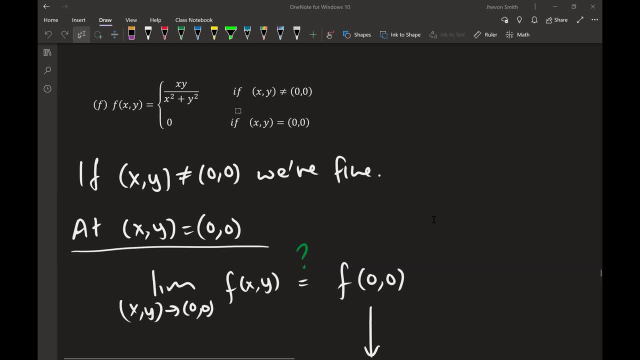 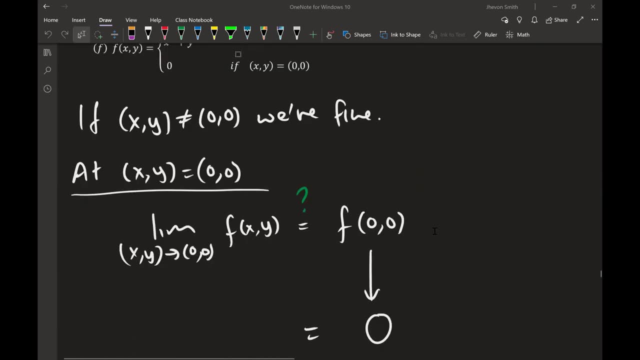 Because it's indeterminate form. Indeterminate doesn't mean the limit doesn't exist. We did examples yesterday where we saw an indeterminate form and the limit didn't exist. Indeterminate means you can't tell what it is at face value. You have to do. 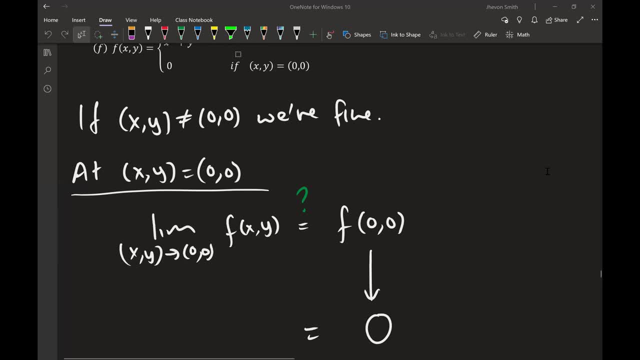 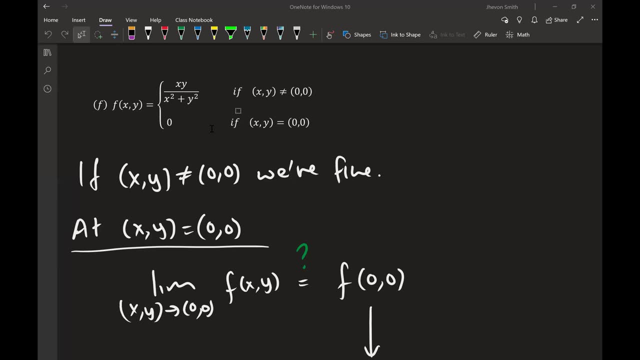 something. Okay, so remember your training, grasshoppers. You see a limit that you don't know how to deal with. What do you do? Step one: try to show. it does not exist, which means you should immediately start thinking what happens if I? 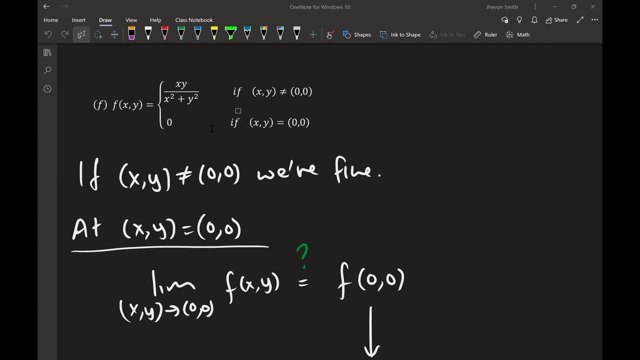 approach this from different paths. What paths? One path is going to be the obvious path. Let's approach along x equals zero. I get the answer: zero. Okay, what's another obvious path? Well, something that allows me to combine the terms of the denominator y equals x. You'll notice that if you approach from 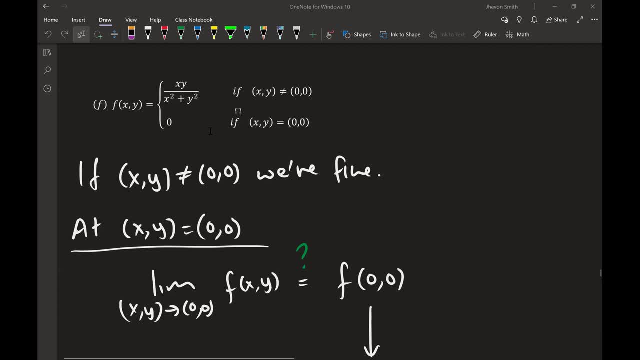 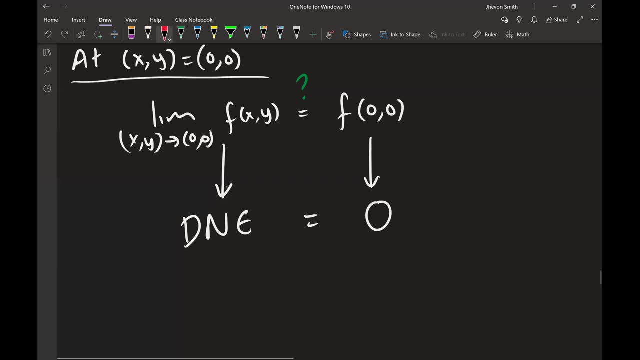 y equals x. you'll get the answer: 1⁄2.. 1⁄2 is not equal to zero, therefore does not exist, Right? That's what should go through your head. That's how you're supposed to think about a problem. You know, what did you want to do in? 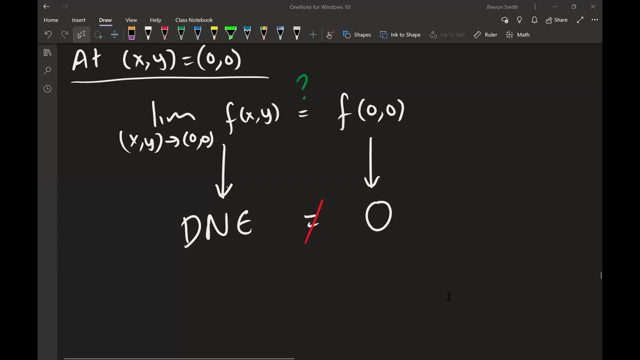 his notes What's going on Like no, You have to remember the strategy and you just know. when I'm in this situation, when I'm faced with this problem, this is how I get myself out of it. This is where I look for first. This is where I look for. 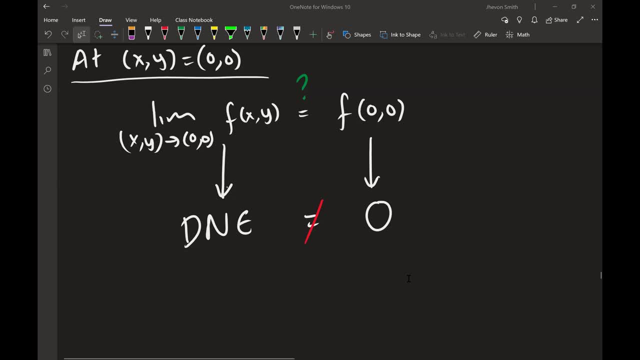 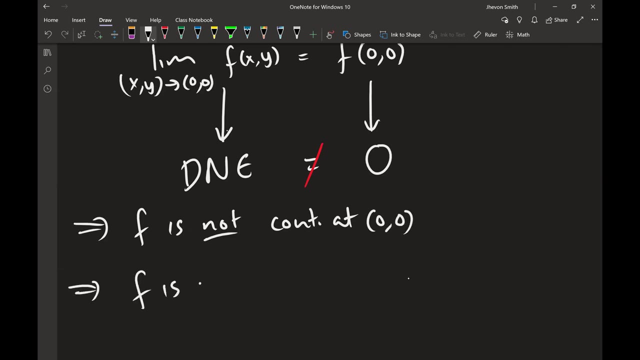 second. This is where I look for third. Okay, so this actually does not exist, which means it's not continuous at the origin, which means f is continuous well, ever except the origin. So here it's like you have to use what you learned about limits, but at the same. 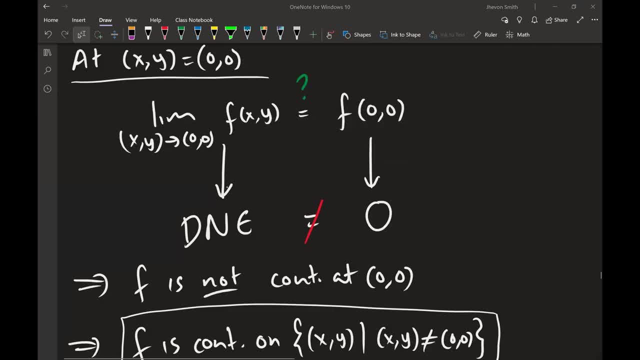 time. you need to match that up to the output of the function at some point of interest and you have to see: does the limit and the point of interest agree? If they agree, then it's continuous at that point. If they don't agree, then it's continuous at that point. If they don't agree, then it's. 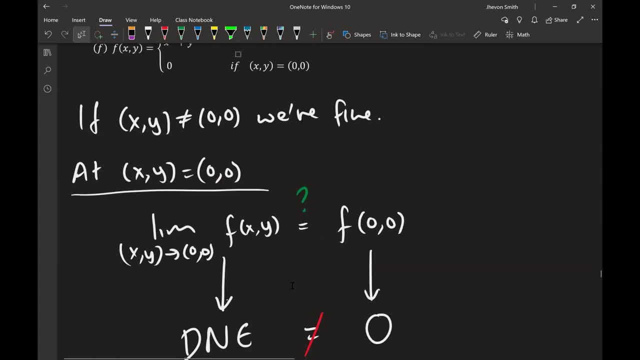 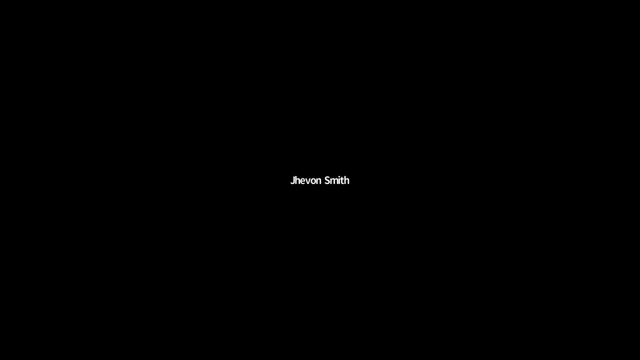 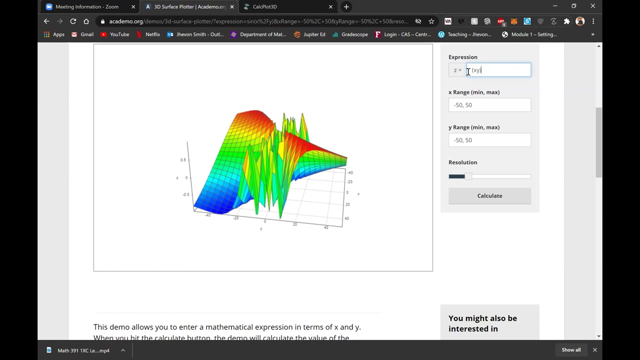 not continuous at that point, But ultimately you need to know how to find limits. We covered that a lot yesterday. Let's look at what does this guy look like. So last time we looked at x squared y divided by x squared plus y. 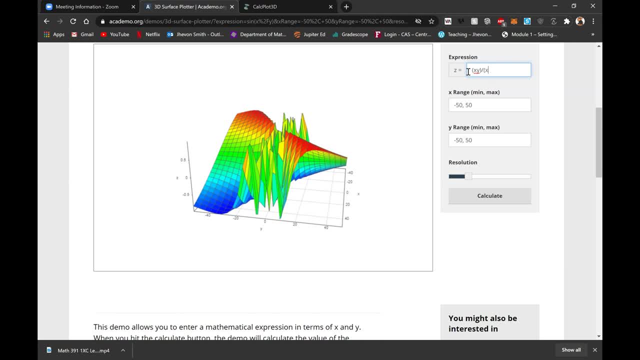 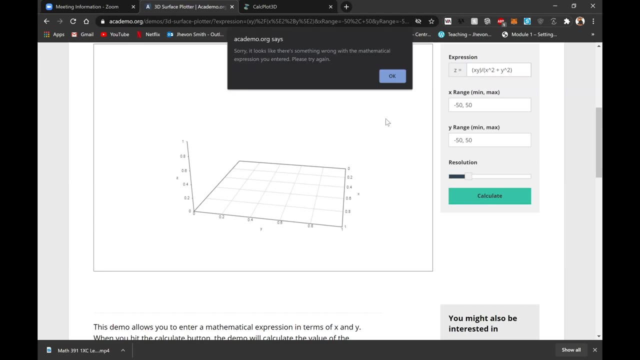 squared. that guy only had a problem at one point. Now we're looking at x times y over, x squared plus y squared. Did I type something wrong? The spaces- Oh, you think it doesn't like the spaces. I put spaces last time. Maybe it doesn't like. 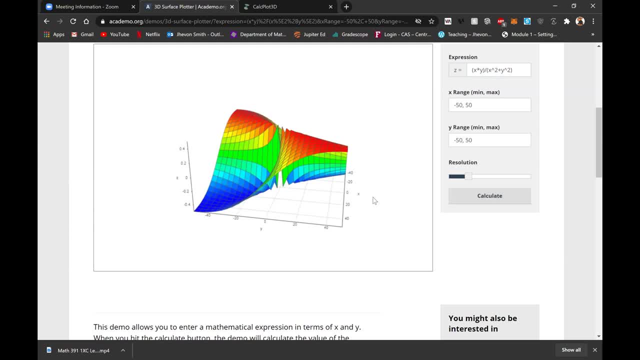 the multiplication. Maybe I need to put an asterisk. Oh, that's what it didn't like. So here, notice what happens when before you can compare this to what we saw when it was an x squared y versus an x times y in the numerator. Notice, with an x times y there's 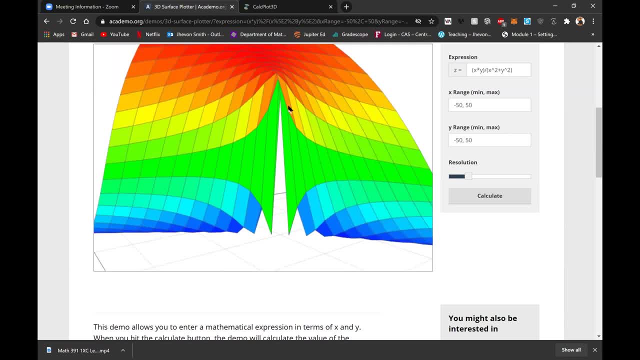 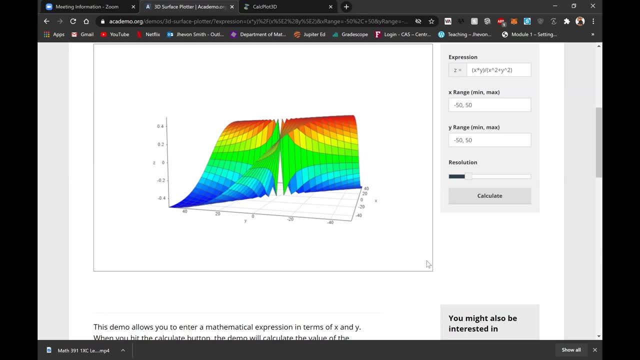 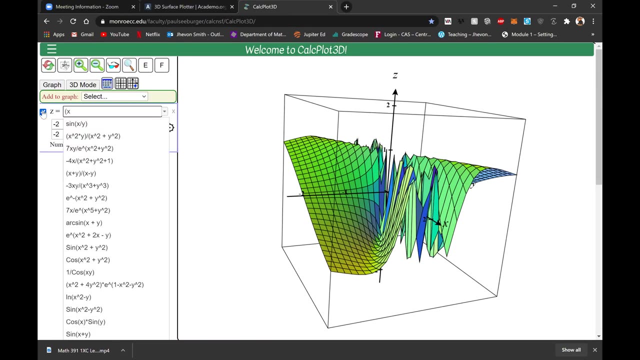 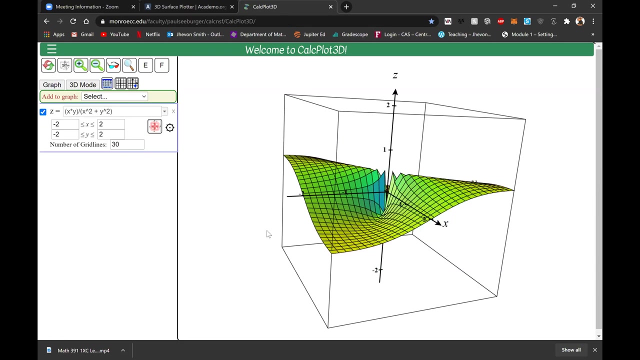 like this huge little chasm right here in our function, Right? That wasn't there before. So here: x times y, less than over x squared plus y squared. So that's what our guy looks like. It's not as bad as the one we had just before, but compared to your x squared y. 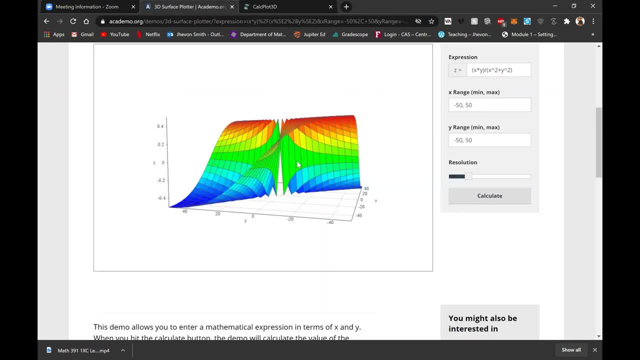 you know, look at that guy. That's what's going on at the origin. Now you guys can just watch. Let me take some pictures of this. Oh, that's all good. Yeah, I remember hearing about it earlier, but it's not as much of an issue right now. 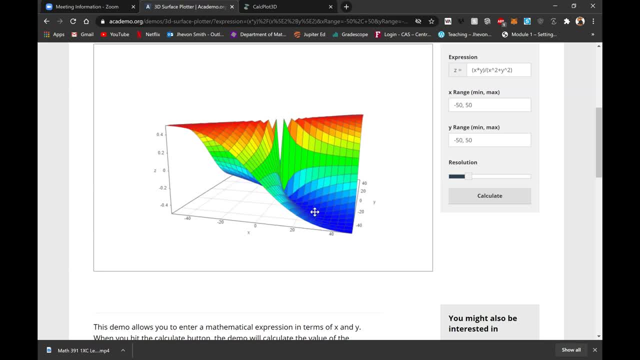 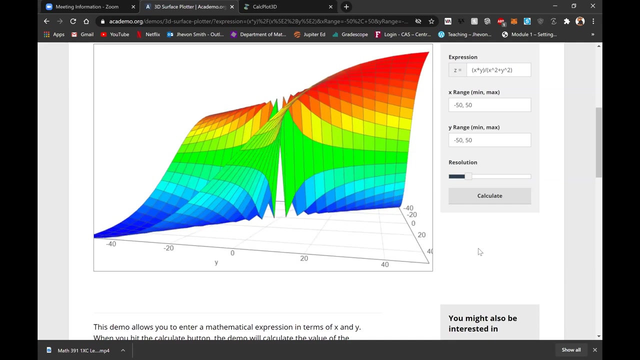 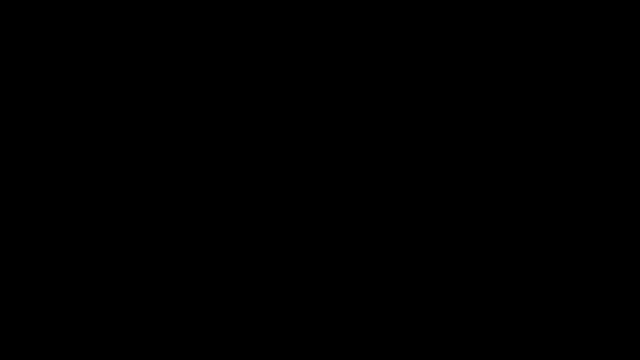 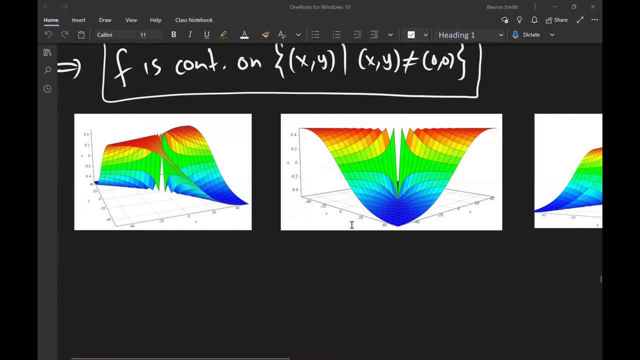 So I'm not calling it x squared. Okay Yeah, Okay, Okay Okay. So now we're just looking at this guy from different views. Here we go, Here we go, Here we go, Let's go back And we're back. So these are just some different views. This guy. 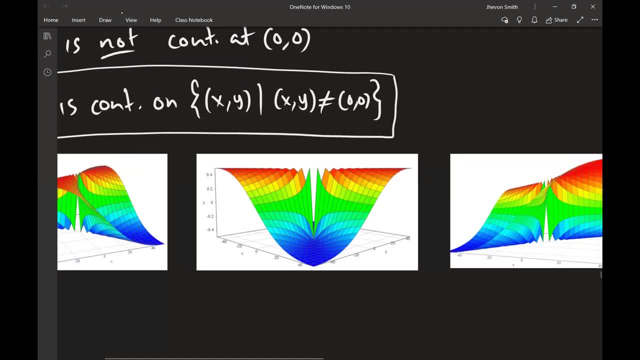 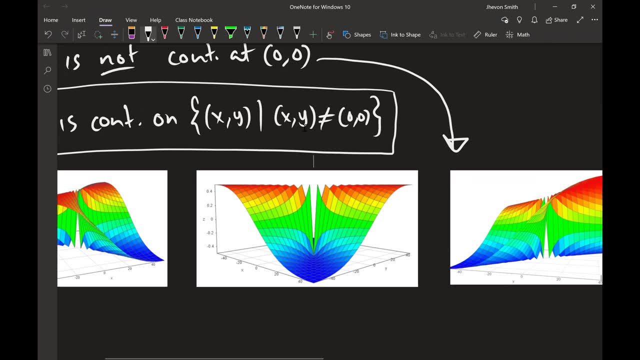 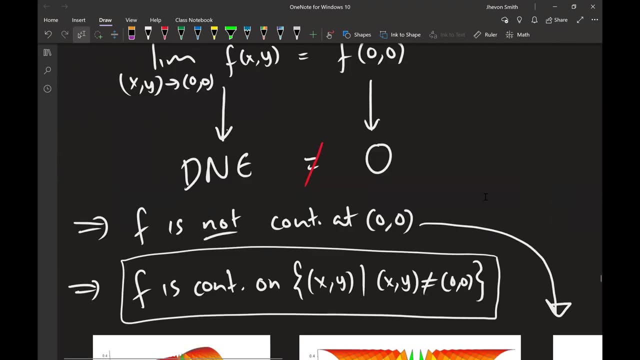 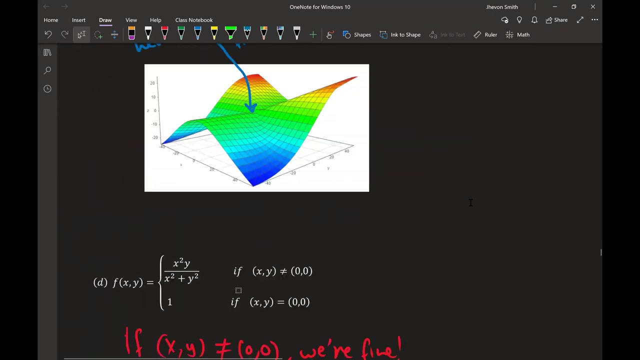 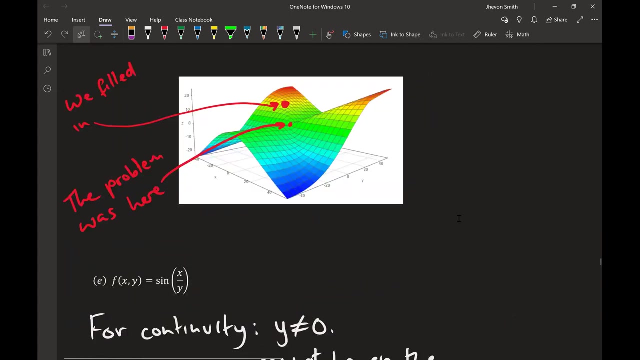 Now I see some pictures And you guys have the websites. I sent links to both of these websites up here. Where I'm taking the snapshots from is the first link, But the one that you can just have things rotate, It's rotating. It's the second link. That was example F. I believe that was the last. 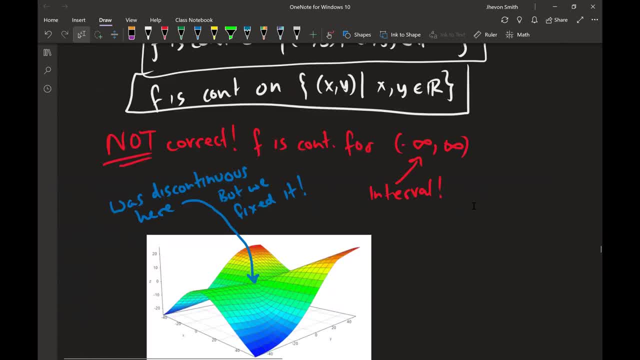 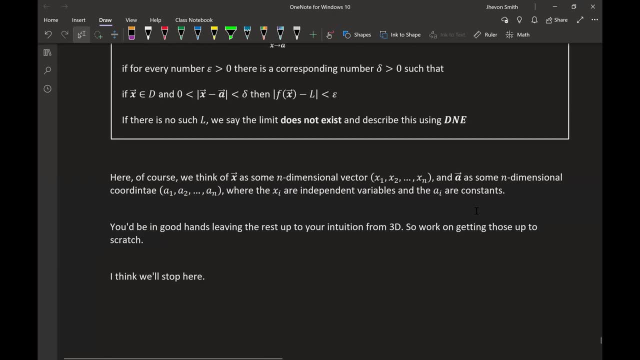 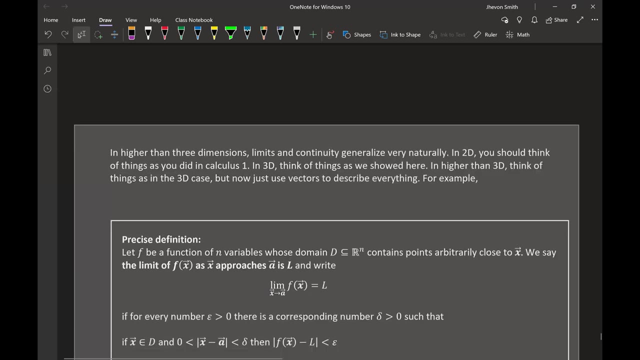 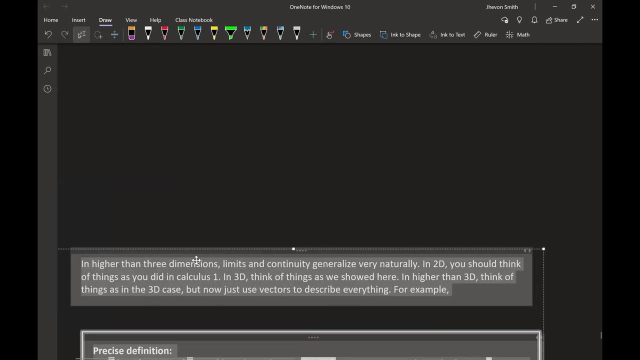 example in this section. All right, Okay, And that's pretty much all I wanted to cover over there. So you should know how to find where a function is continuous. Here I kind of put the name of the function. I'm going to use this little blurb here for the sake of completeness. 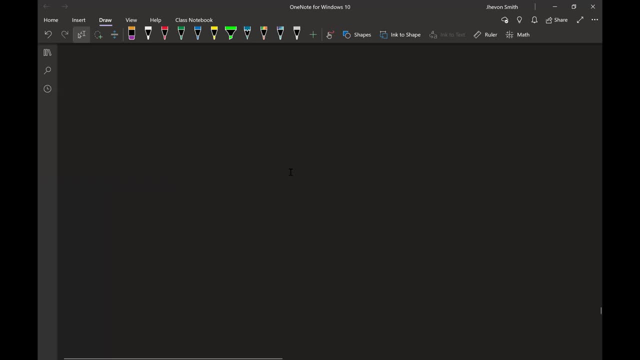 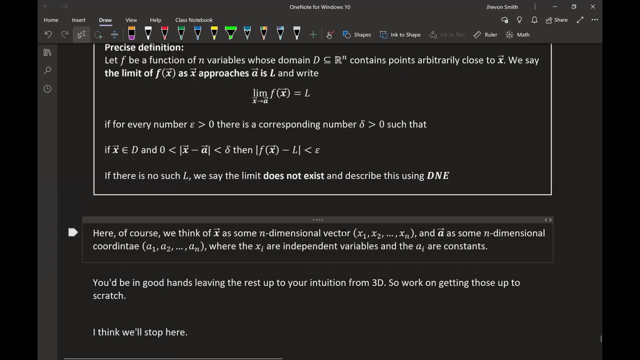 Technically, I don't think you'll ever need to actually know this stuff, But just to mention what we were doing here can work in higher dimensions as well. It just gets a lot harder the moment you start bumping up for dimensions. So for higher than three dimensions once. 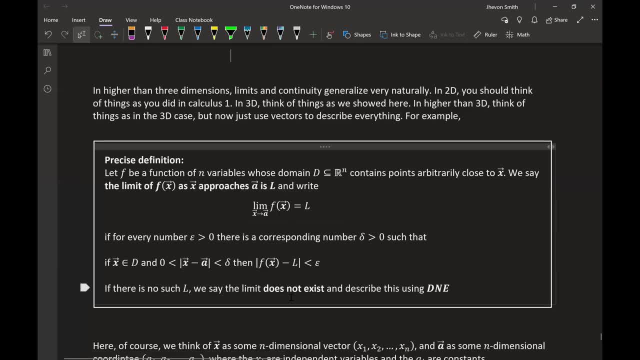 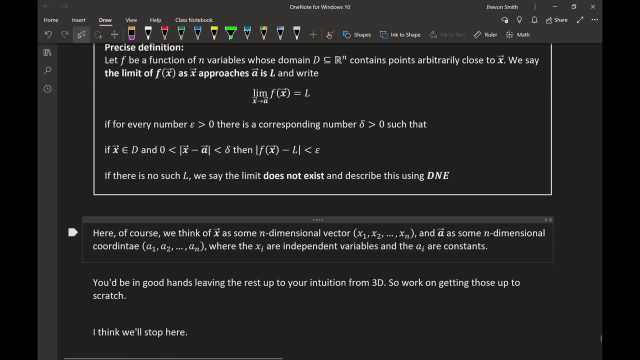 you're in 4D or higher, it becomes much more efficient to use vectors to describe everything. So you describe a point, a variable point, as just a coordinate. You'll describe a constant point that you're approaching as a coordinate of constants. 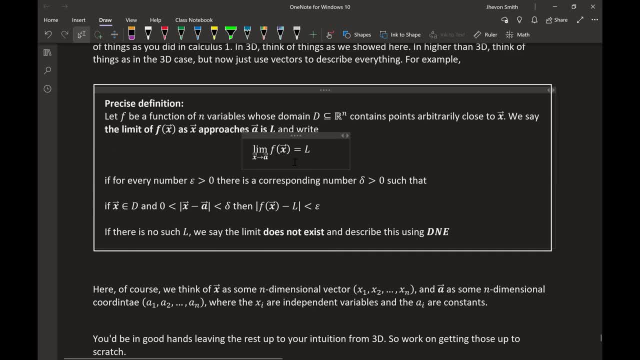 And you can actually use vectors to talk about this stuff, And the squeeze theorem would apply in the cases of vectors as well. Of course you have to be when you take the absolute value. in this case, of course, that means you're taking the absolute value of a vector. 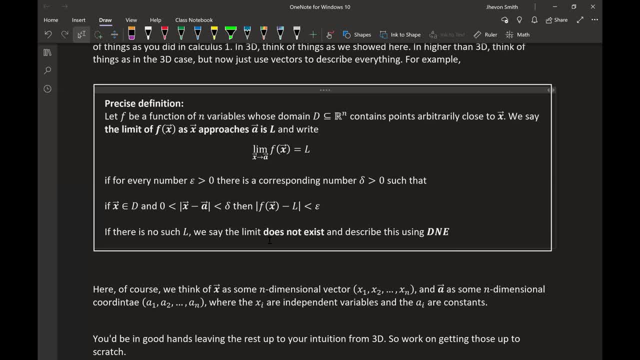 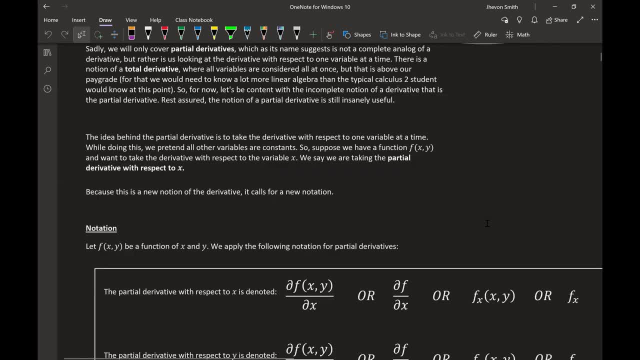 more efficient to use the formulas for the magnitude of a vector, and etc. But when you get high enough dimensions, it becomes much more efficient to use the formulas for the masters. Okay, so for now. what we're going to look at, though, is the partial derivative, And this is 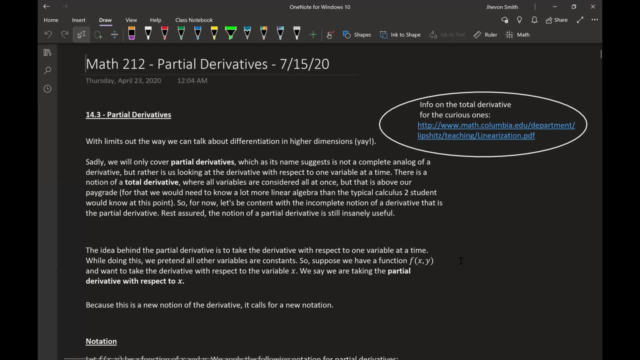 really what you can think of it, as is the derivative from a certain perspective, The derivative from the perspective of one variable at a time. So essentially what this is going to be for a multivariable function. you can talk about things like, say, you have a function of x and y. you can 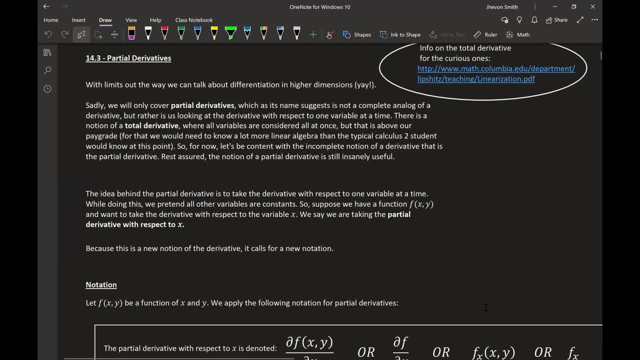 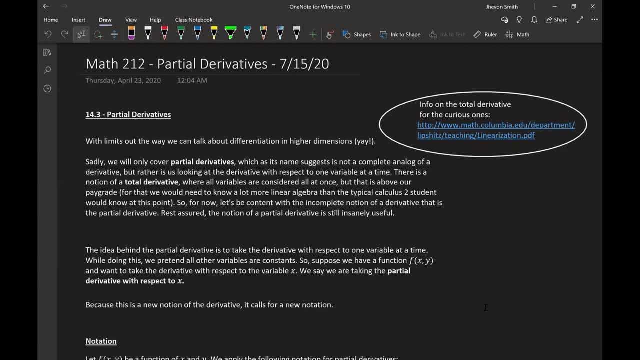 talk about things like the partial derivative with respect to x or the partial derivative with respect to y, etc. And basically what this means is that you're looking at this multivariable function where it has variables x and y as independent variables. However, what you do is 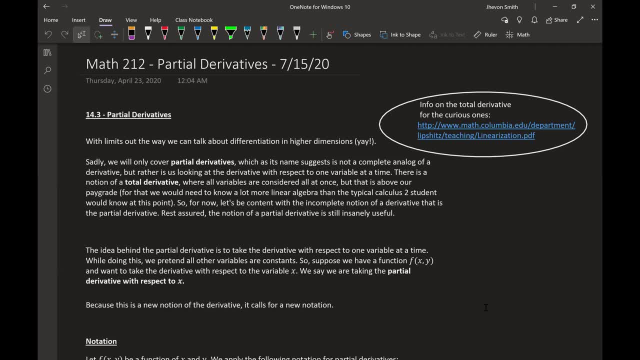 you look at x as a variable and you pretend all other variables are constants. They might as well be constants. You freeze everyone except one guy and then you look as the derivative in terms of that guy, right, And this is what you call a partial derivative Now, to indicate that you're 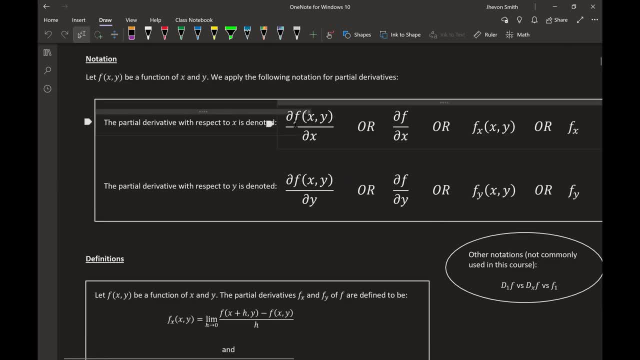 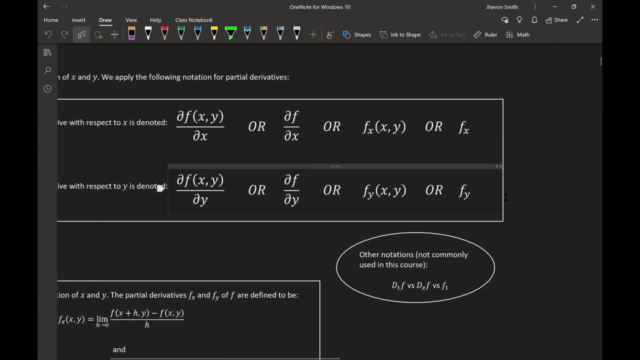 looking at a partial derivative, you actually change the notation. So we're upgrading our notation here, right? So you know, we're moving out the hood, we're getting a nicer car, everything like that. When you want to talk about a partial derivative, you draw a curly d right. So when someone writes something like: 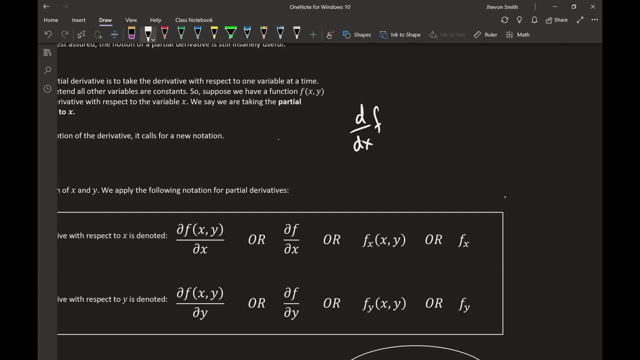 d, dx of f. this we think of as an ordinary derivative. Here we are thinking of things like: this is like the kelp. So if you were to write something like this, you would say that f is a single variable, a single function, And here you'd assume that f is a single variable function. 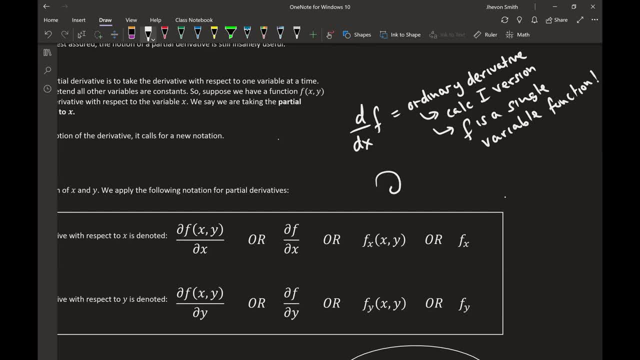 However, you can get bigger, You can go something like this and you draw like a curly d, like that. This is what's called a partial derivative, Meaning it's a derivative with respect to the x variable, But with the awareness there are other variables out there. 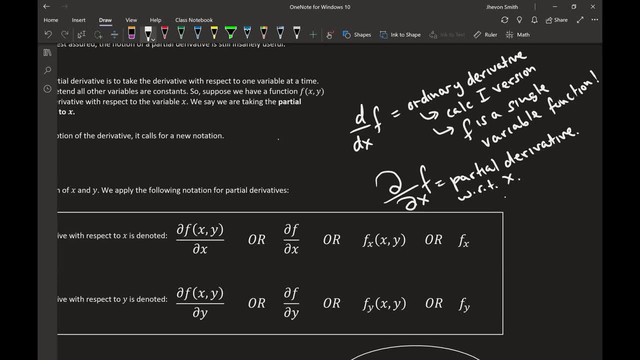 So the partial derivative with respect to x. But f is a multivariable function, So there are other variables out there. So you draw a very curly D. Yes, it looks like a backward six And it turns out that some students write their Ds like this anyway. 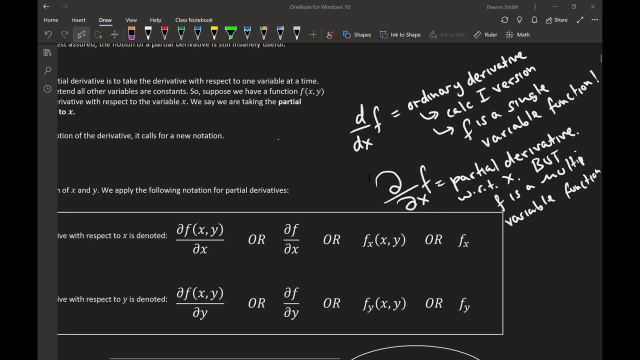 And so there were tons of students where in calc one, I had to correct them when they were writing derivative. They would write their Ds like this, That or something like, instead of like this, And I had to correct them: like no, write it like this. 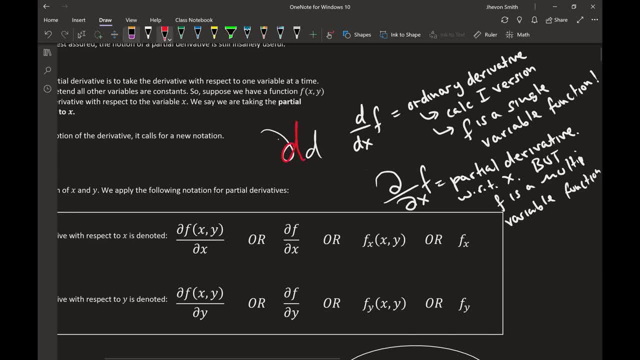 And I'd write over it and go, no, you should be writing this instead. And they're like, oh, he's just trying to take off points for no reason. And I'm like, no, you don't understand. There's going to come a point where things are going to change. 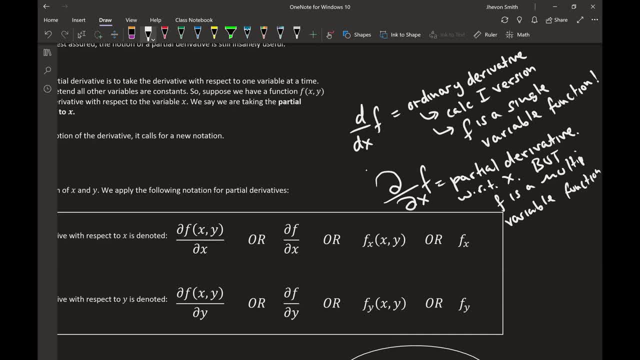 Like I was telling you guys, language is important, How you write things down is important, because there comes a point where, if you're not doing everything correctly, there comes a point where, when the notation changes on you, you 're not going to notice. and you're going to read something and you're going to have 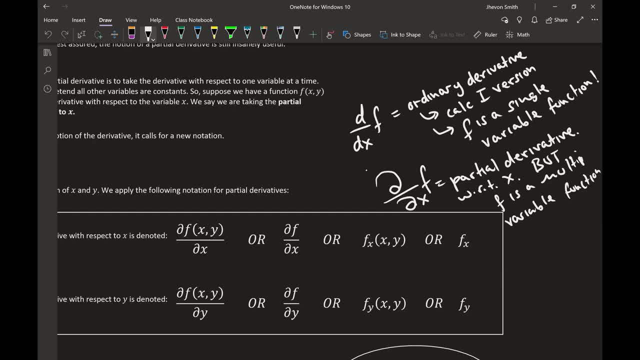 a completely different picture in your head than what's actually going on. And then you're going to be there studying for hours a day and still getting bad grades, because you're all confused And a part of it is just language, Part of it is just you never were writing things down correctly in the first place. 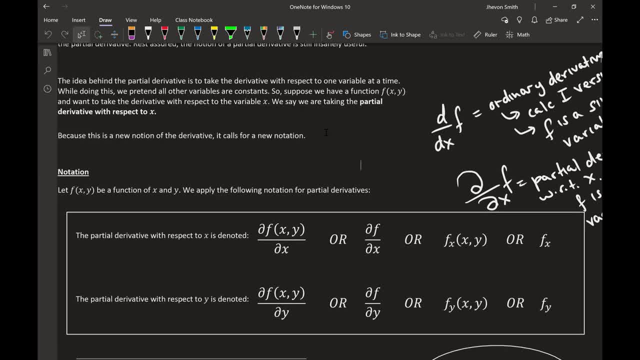 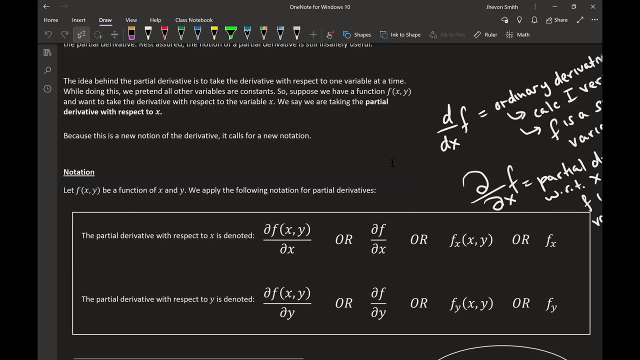 So it wasn't that I. sometimes I mark people take off points for things and they think I'm being mean. but it's not that I'm being mean. I just know where you're going and I understand This thing that you don't think is a big deal. 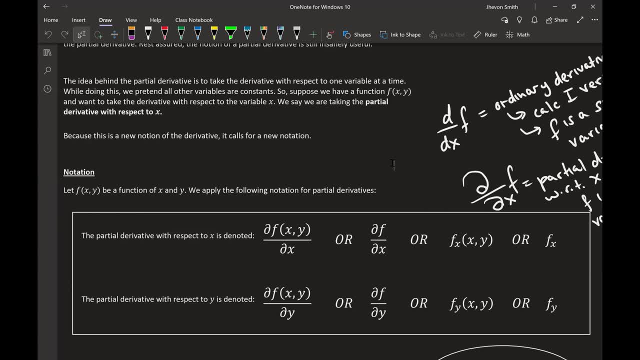 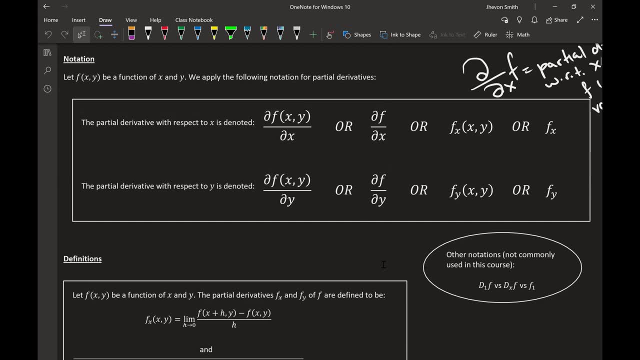 Big deal right now is a bad habit that you're going to pay for later, So correct it now. So the notation is the following: So we do have a Leibniz version of the notation here, but we use curly D, So this is still. 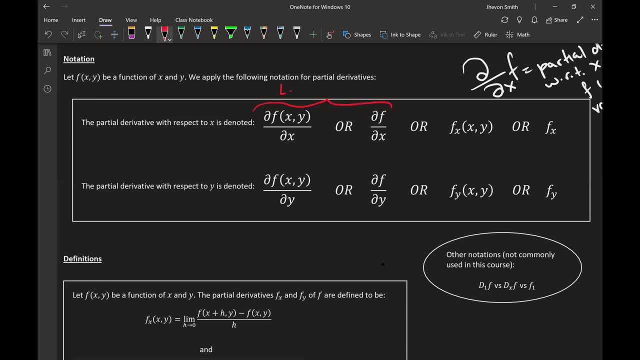 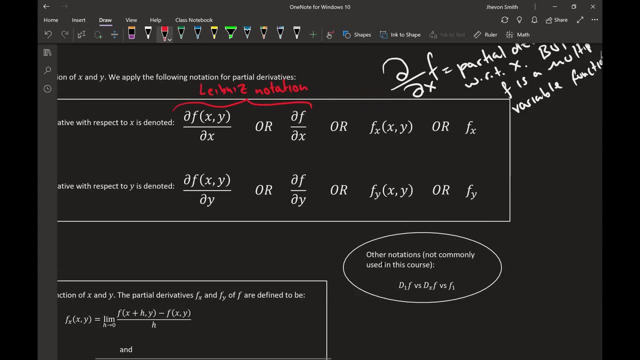 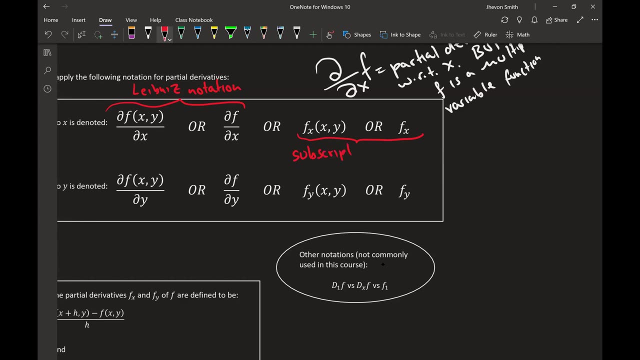 called the Leibniz notation. And there's another notation that we have, this guy where we do a subscript. This is called the subscript notation. There is no prime notation anymore. So to say f, prime of x, not a thing anymore. 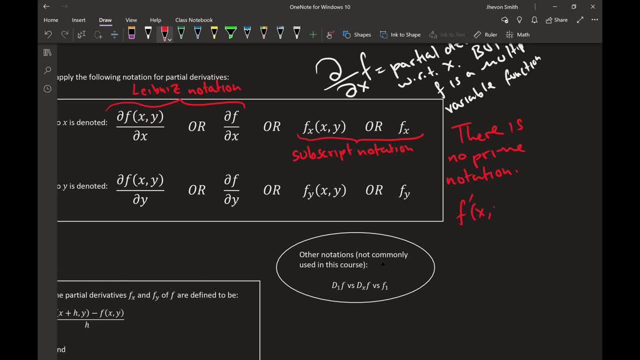 Right. because if someone says f, prime of x, comma y is too vague. right, The prime indicates you're taking a derivative, but it's too vague. It's too vague. It's too vague. Right, The prime notation indicates you're taking a derivative, but you're not sure. with respect, 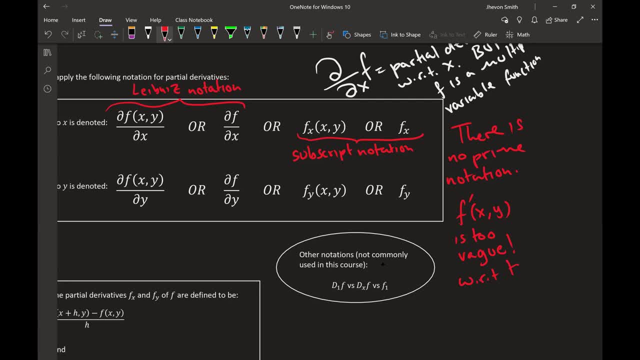 to who? Is x the variable with respect to who? You don't know if you're taking the derivative with respect to x or with respect to y. So the prime is very vague. It's not used anymore. Once you go into a higher dimensional kind of situation, you either use the Leibniz notation, 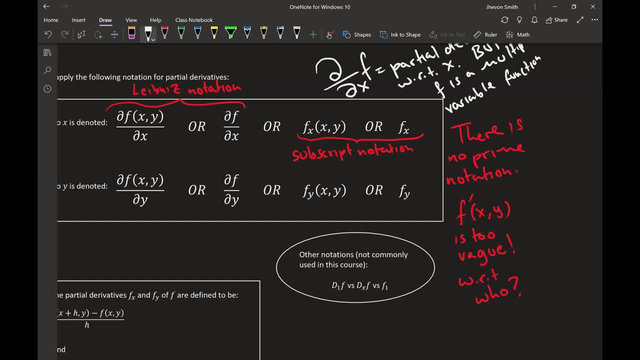 or the subscript notation, And they actually behave differently. They mean the same thing, But you have to be careful. I'll talk about that later in how these notations behave. There's some other very common notations, but we're not going to be using them. 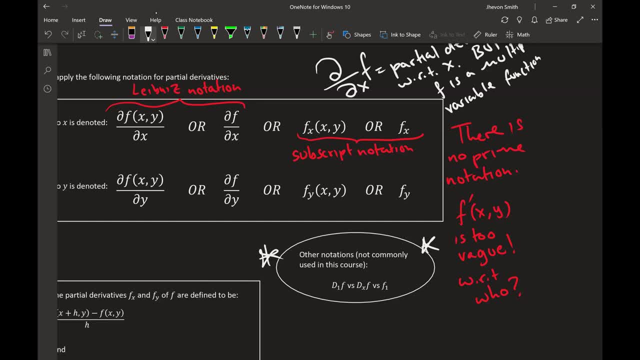 I'm going to use either the Leibniz or the subscript notation, And most of the time I'll write down the subscript notation because it's actually just easier to write down. It's easier to write just an f sub x instead of a squiggly df divided by squiggly dx. 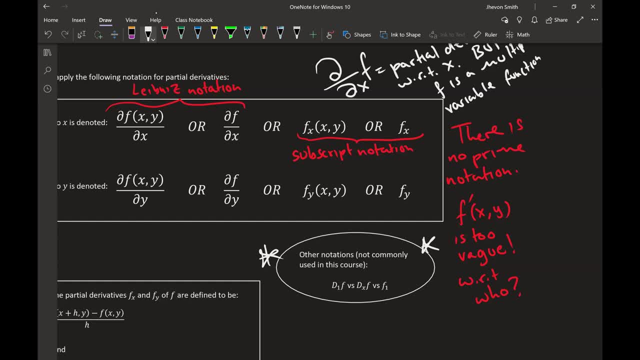 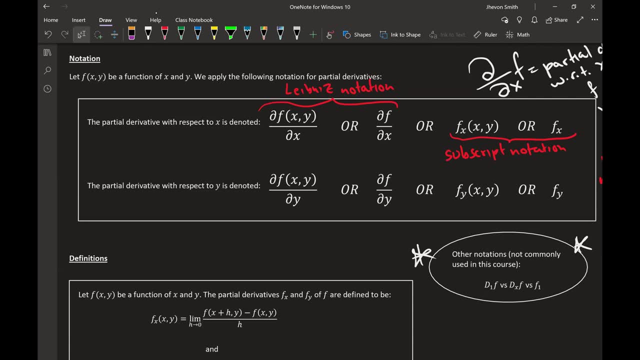 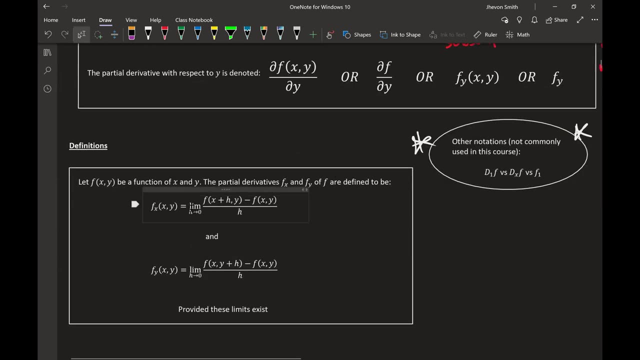 There are times where the Leibniz notation is actually quite useful, But at this level, whichever notation you want to use is fine, Just don't mix the notations. Now, what is the technical definition of a partial derivative? It's like this guy here. 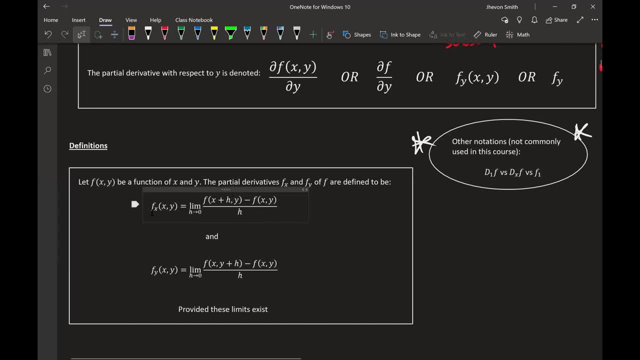 It looks very much like a difference quotient. However, you'll notice, for the partial derivative with respect to x, the x plus h, the x is what's changing by h, whereas the y is being left alone in the partial derivative with respect to y. 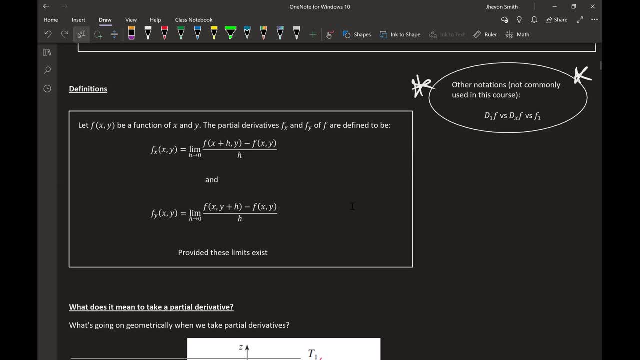 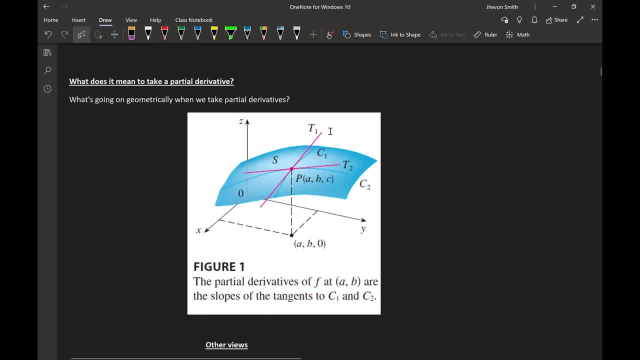 The y is changing by the h and the x is being left alone. So this is called a partial derivative. Visually, what does this mean? It means I have this surface and I just I look in the x direction for the derivative and I'm looking at the slope just in the x direction. 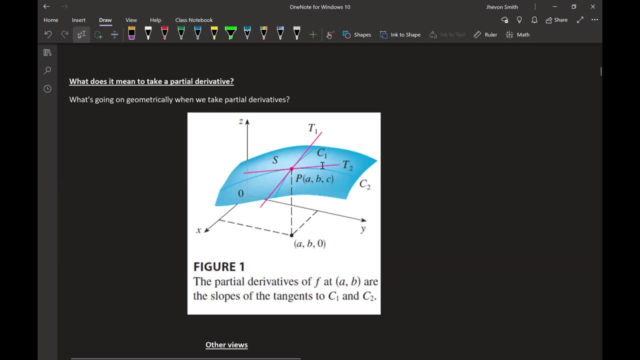 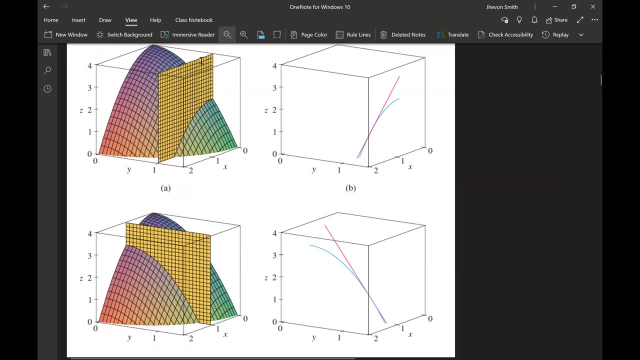 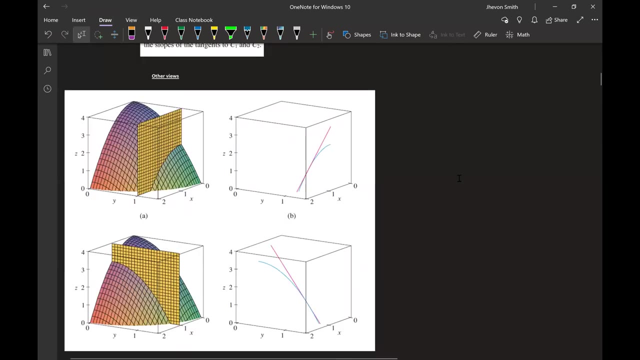 It's very different from the slope in the y direction, right? If you want another visualization, here's like a surface. let me actually reduce the size a little bit. Here's like a surface. When I take a partial derivative, it's like I'm slicing through a surface with a plane. 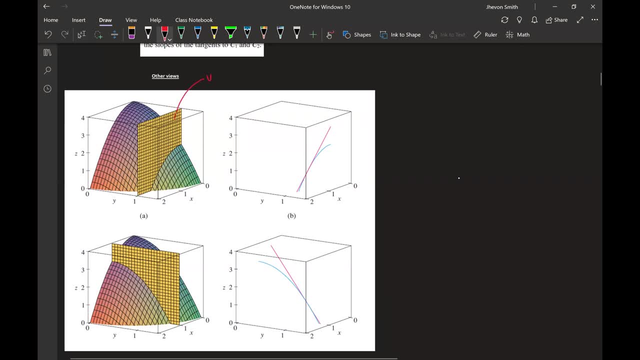 So this here is some plane. Let's say this here is: y equals a constant. It will slice through this curve like here, right, Then I can find a tangent line to that right, Which brings you over here. Now, the slope of this tangent line is the partial 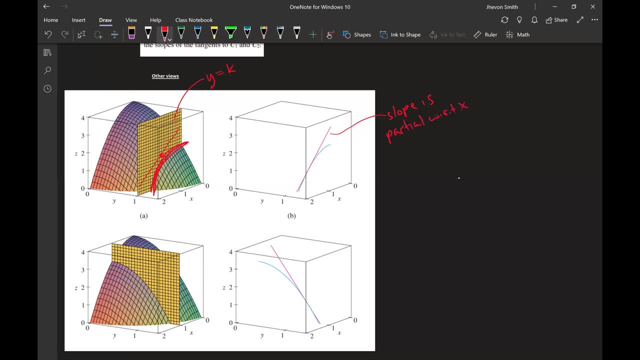 Okay, With respect to x, at the point or points where y equals k. So if I slice through with a constant, so I'm thinking of my y as a constant, which means I'm thinking of it as a plane in three space When it slices through my function. if I imagine the cross section as the curve I'm measuring. 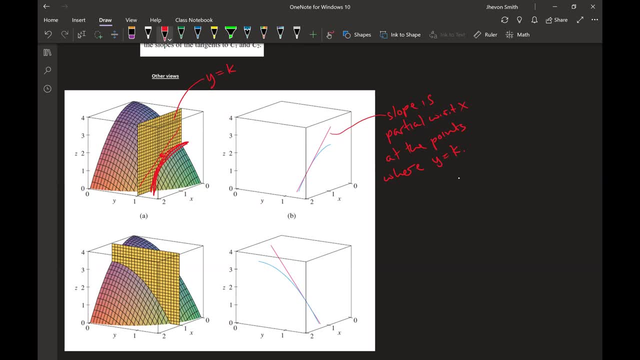 and I find a tangent line to that curve. the slope of that tangent line is a partial wither, So I'm thinking of my y as a constant, which means I'm thinking of it as a plane in three space. So the slope of that tangent line is a partial with respect to x. 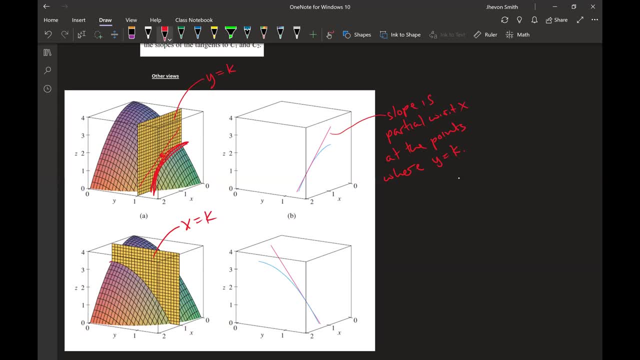 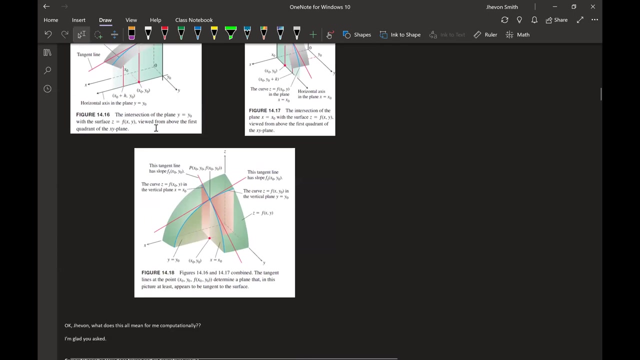 If here, if I have, x equals a constant, then the slope here equals the partial with respect to y, et cetera. right Now again, here's another visualization. This one is that these are actually from your textbooks, so you can read those slowly. 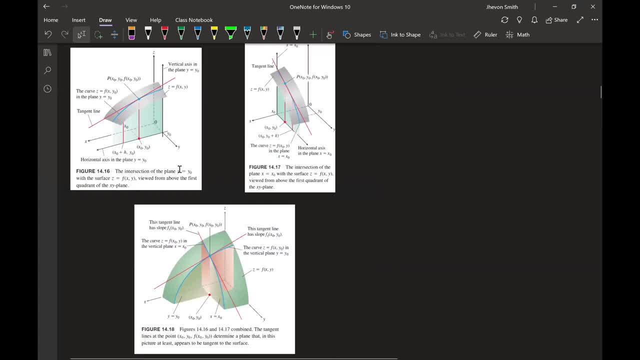 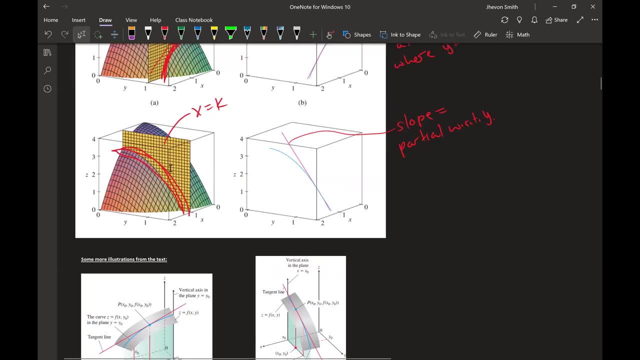 But that's the Okay, That's the visual, the visuals of what's going on, Okay. So yeah, you're like taking the slope of a tangent line, but from a very specific perspective, and you can change the constant k and you will just move this plane forward or backwards. 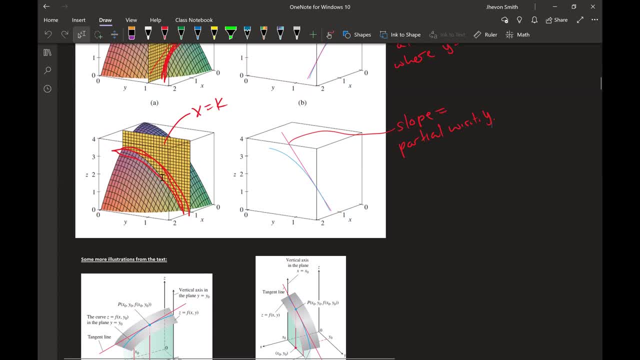 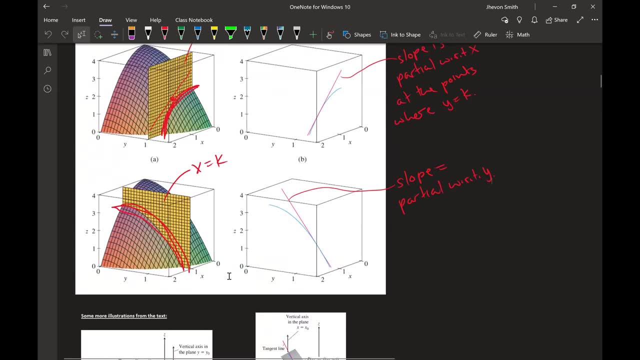 through the surface, you'll get new curves to which you can find new tangent lines, to which you can find new slopes. So the slope is a much more dynamic animal. now, right, And slicing one direction versus slicing the other direction, I can get different slopes. 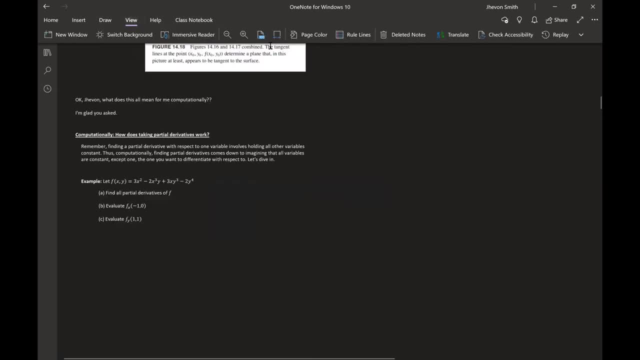 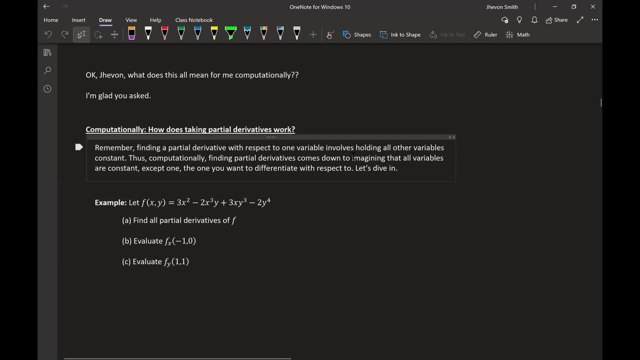 So yeah, we can now find the derivative in the x direction versus the y direction. Let's make this a little bigger, All right, So that's visually what a partial derivative is. Now let's talk about computationally what everyone likes, right? 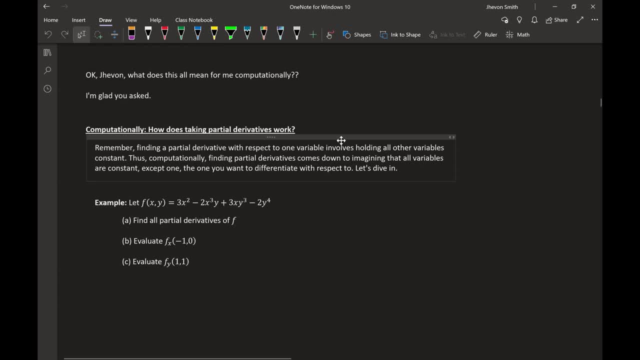 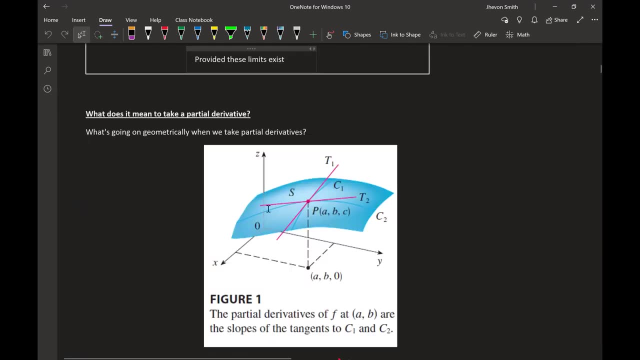 If I ask you to compute a partial derivative, how would you do it? Now, I'm not even going to ask you to use the definition of the derivative. We're not even going to touch that right. So forget about that. You will never have to worry about that. 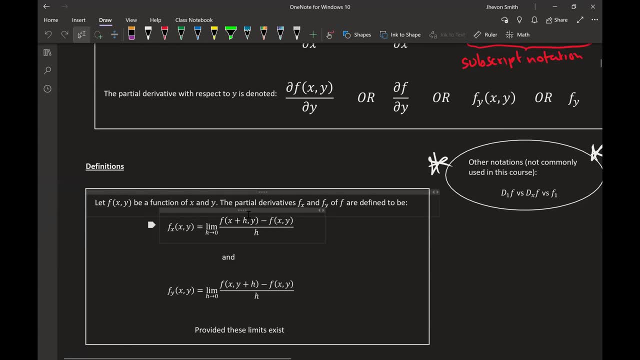 The definition is important Technically. you should know it, and you should definitely know it, because if a multiple choice problem asks you about it, you should know how to answer that problem. However, computationally speaking, we're just going to do the shortcut way. 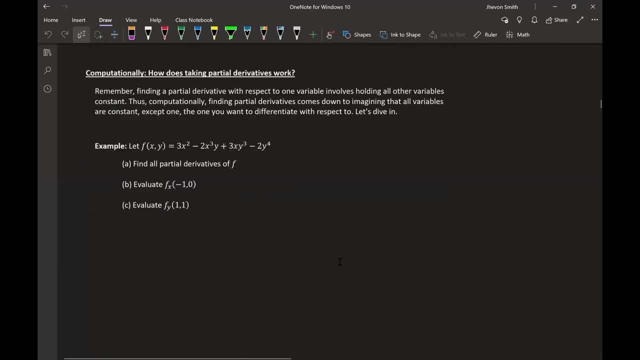 And at this point you guys do know enough to do the shortcut way. Here's the thing about computationally finding a partial derivative. It's pretty much exactly the same as you did find derivatives in Calc 1.. The only difference is here is that you hold one variable. 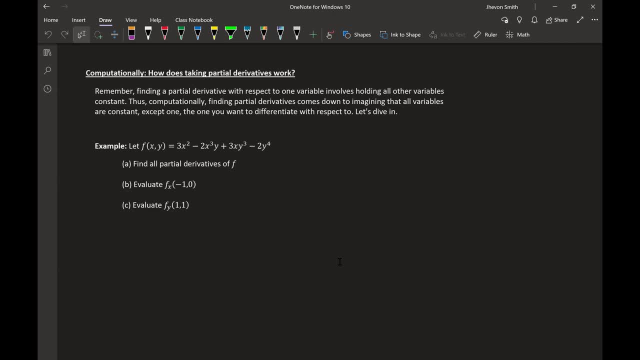 Hold all variables constant, except the one you're focused on at a time, And so here's what we're going to do: I'm going to just jump in and I'm going to show you what that would actually look like for these guys here. 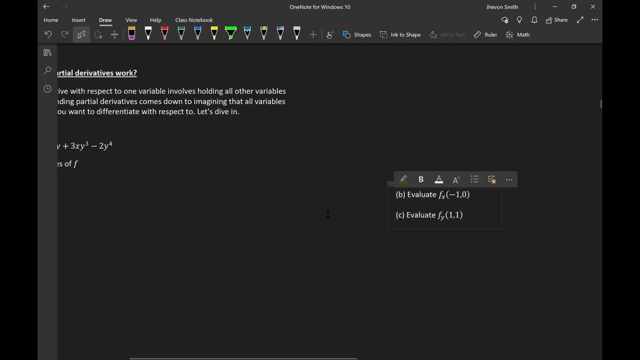 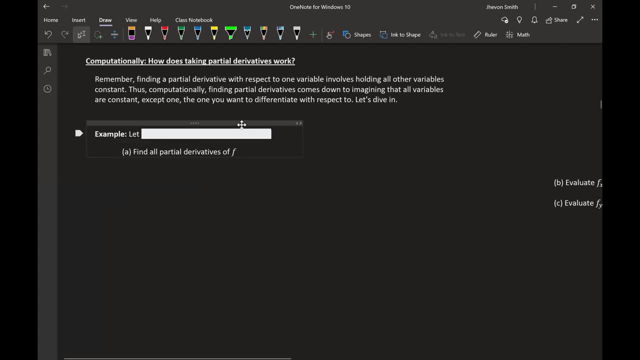 So let's move these guys over. So here's a function: f of x- y equals 3x squared. Okay, Okay. So here's my function: f of x- y equals 3x squared minus 2x cubed y plus 3xy cubed minus. 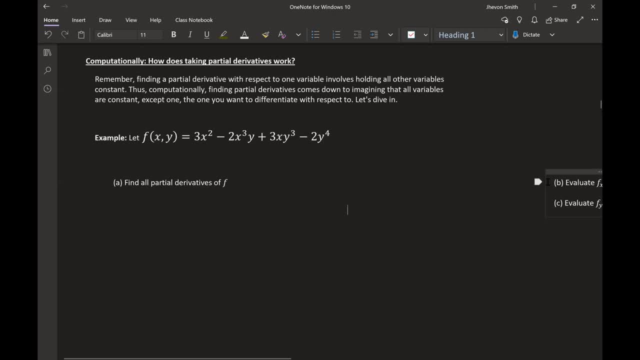 2y to the fourth: All right, Jason's all excited now Like, yes, we're doing it. Is everyone ready? Okay, They're going to. I don't think they're already at, Jason, but I'll get them ready. 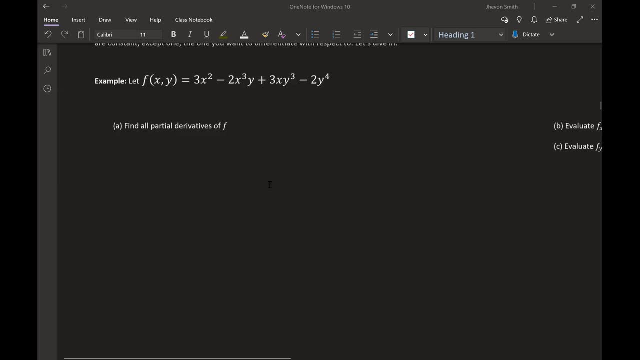 Don't worry. Okay, So find all partial derivatives of f's. Now, as far as you're concerned, you have one partial derivative for each variable that's present. So if I have a two variable function, there are two important partial derivatives. 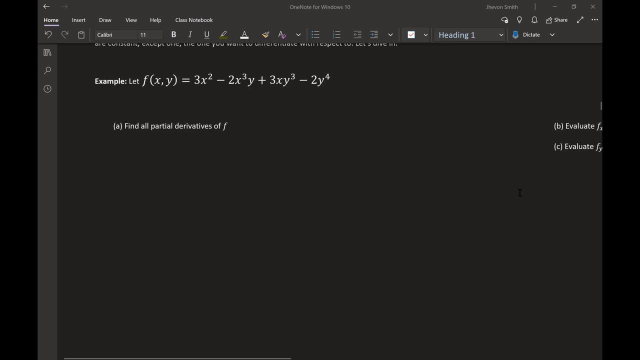 If I have a function of x and y, then the suspense I'm like really just blabbering on before showing you If I have a function x and y, you should think of there being two partial derivatives, So you'll have. 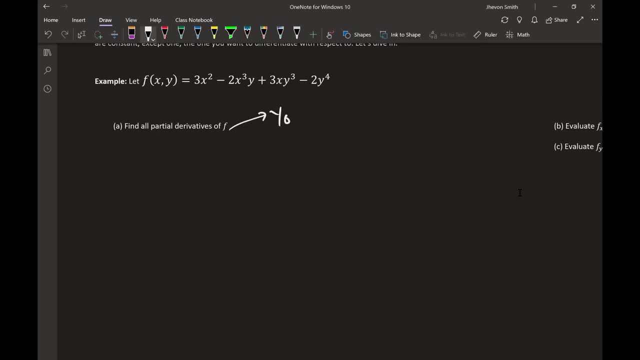 Okay, Okay, So you'll have one for each variable. So f here has two. There is the partial with respect to x and the partial with respect to y. Now let's get this bread right. What would it mean to take the partial with respect to x? 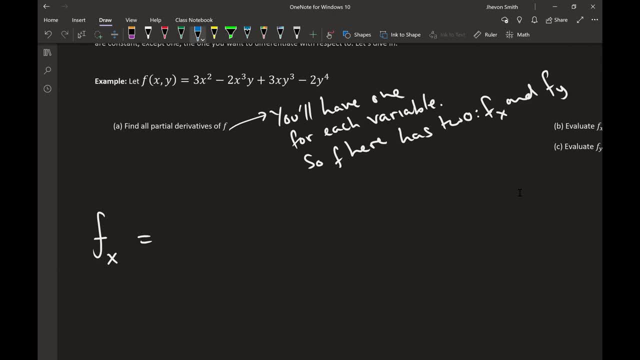 Here is what it means. It means pretend all variables are constants except x. Then you are going to actually take the derivative. Okay, Okay, Okay, Okay. Take the derivative with respect to y, with respect to x. So you're going to go to this function: three x squared, blah, blah, blah. 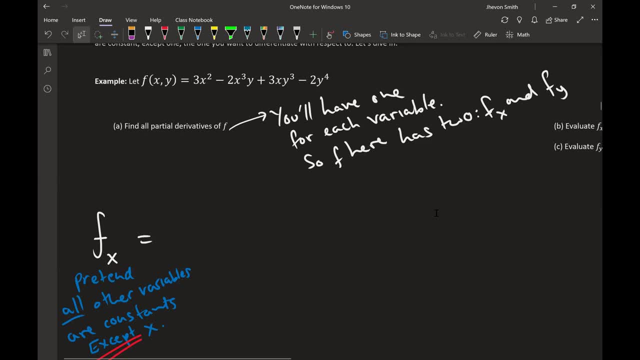 And you're going to literally take the derivative by pretending your y variable is a number. It might as well be five or two or something else. So how would I take the derivative? Well, the derivative of three x squared would be six x minus the derivative. 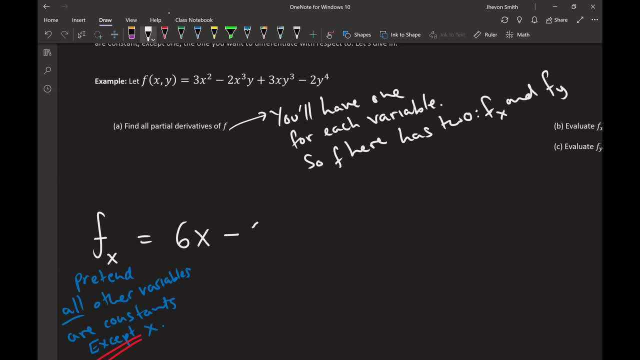 What is the derivative of two x cubed y? Well, six x squared right, then that's because i'm just keeping my y as a constant, so i leave it alone. when i have a constant times a function, the derivative is going to just be the derivative. 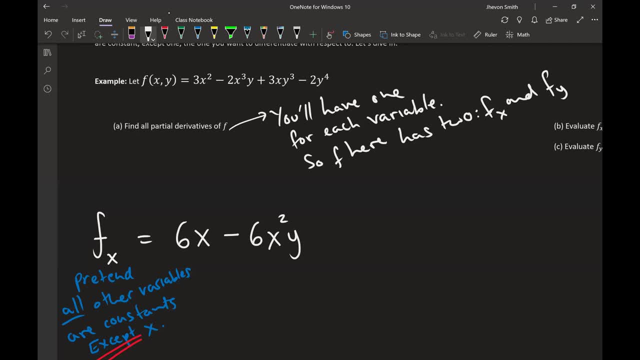 of the function times, the constant. so here i just took the derivative of the x squared and i left everyone else alone. in fact, let me actually just write it out another way. what i do is i leave the 2y alone because it's constant, and i'm going to differentiate the x cubed. 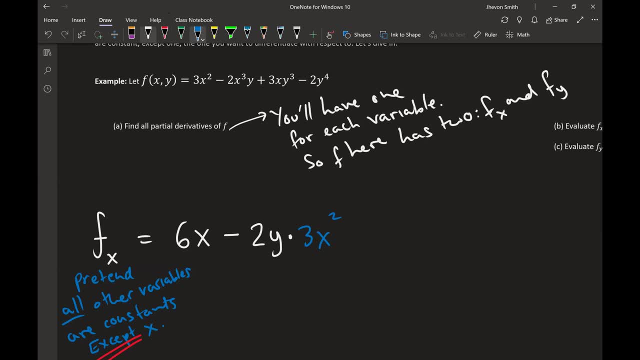 so i would get 3x squared and i continue in this fashion. so when i get to the 3xy cubed, i would leave the 3y cubed and i'm going to differentiate the x, which is just one, when i get to the minus 2y to the fourth. this is just zero. notice that this guy is constant. 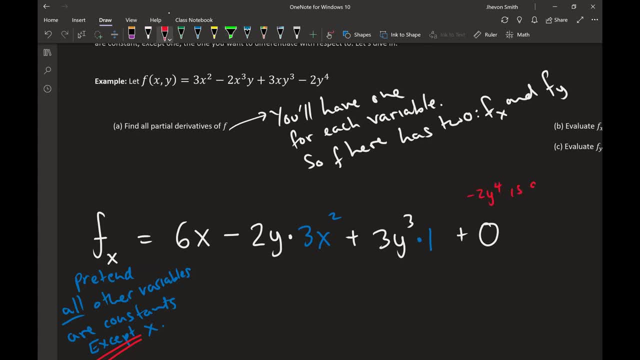 because my minus 2y to the fourth is a constant with respect to x, so the derivative of 2y4, so derivative with respect to x of minus 2y to the fourth, is zero. and so now, of course, when you'll get quicker with this in your head after you do it a few times, 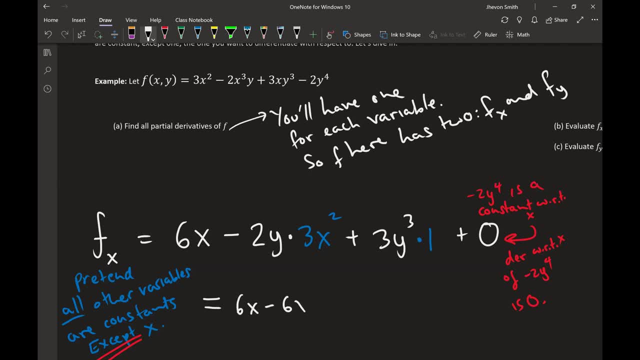 i can clean up. this is 6x minus 6x squared y plus 3y cubed. that is going to be my partial with respect to x. are we getting it? uh, i just have one quick question. yes, so in. so for this example, let's say so basically, whenever we're doing partial derivatives. 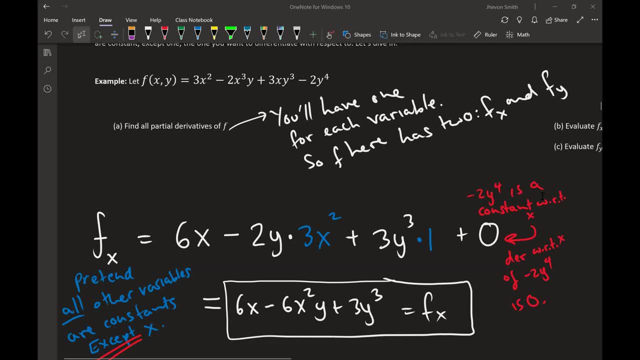 If we have a variable that's a constant and it's by itself meaning that it's not also being meaning that the variable that's also being derived isn't, I guess, attached to it? it would just automatically be zero. Yes, because the derivative of a constant is zero. 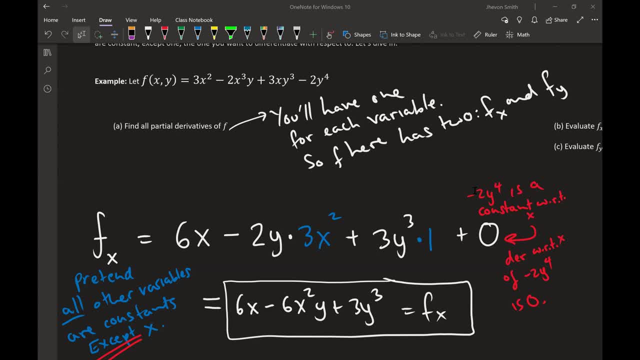 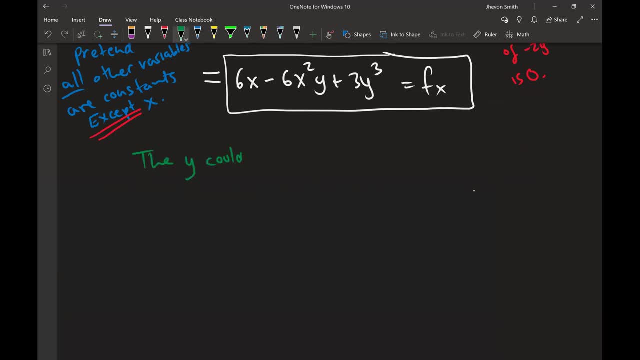 Okay, Okay, got it Right. It's literally like. it's literally like the y could be a five probably here. Does anyone want to do fy, the derivative of y, Jason, hold on, Hold on. I know you're excited, but stay with the class for all we care. 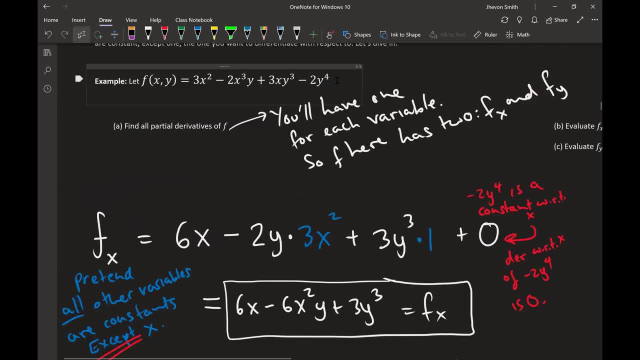 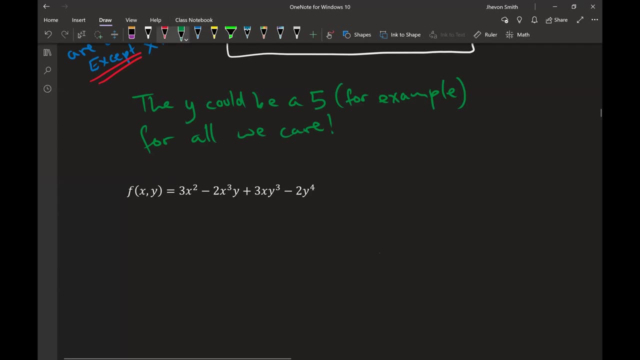 What this means is that if I look at this function- I know you already looked at this, but not everyone looked at it, Jason, So I want to make sure That we're not running too fast for everybody. So if I looked at this function here, right, I could literally just think of the y's as fives or twos or whatever your favorite number is. 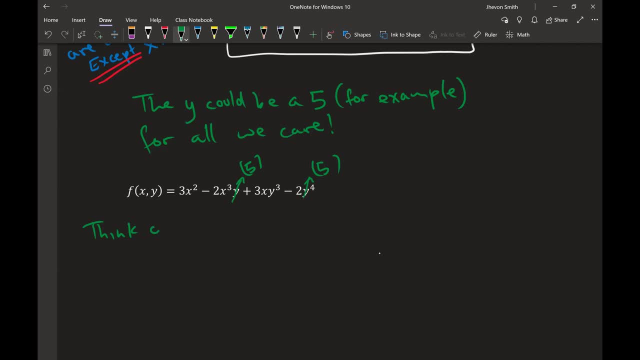 So if I think of this as 3x squared minus 2 times x, cubed times 5, plus 3x times 5, cubed minus 2 times 5 to the 4th, and I want to take a derivative, how would I have done it? 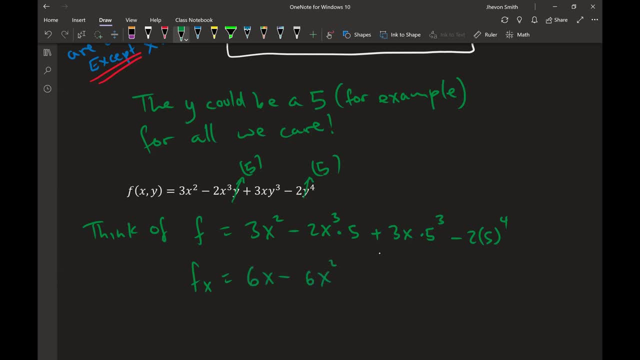 Well, that would be 6x. Here would be 6x squared times 5.. Here I would have 3 times 5 cubed, and this would be zero right, because that's a constant right. So you can literally just envision: there's just some number in place of y and everything you would have done. 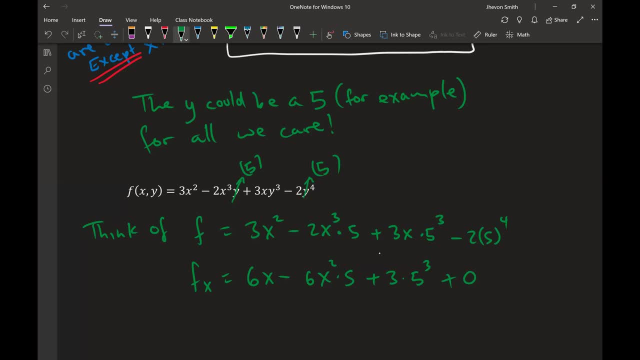 in that situation you are going to do here. So if there's no x attached to it, then it is a constant as far as you care. Okay, you're taking the partial with respect to y if it's partial with respect to x, And so yeah. 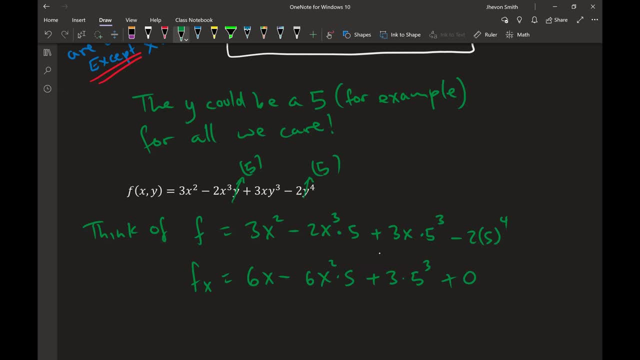 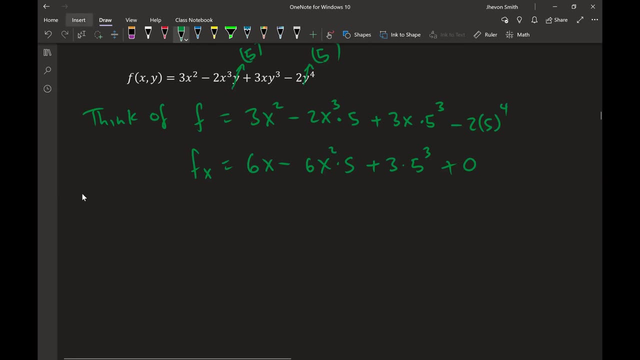 if it's by itself, there's no x attached to it, the derivative is going to go to zero when I'm finding f sub x. So here's the function again. What about partial with respect to y? You want to try it, Kayla? 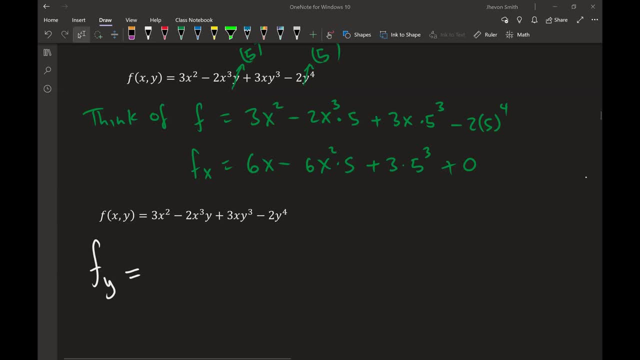 Yeah, I'll go. So the first part, 3x squared, would be zero, since x is a constant, And then you would have minus 2x cubed, because when you derive y that would be one. And then the next part would be plus 9x times y squared. 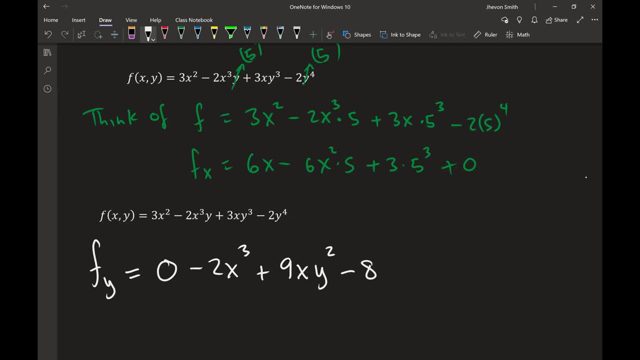 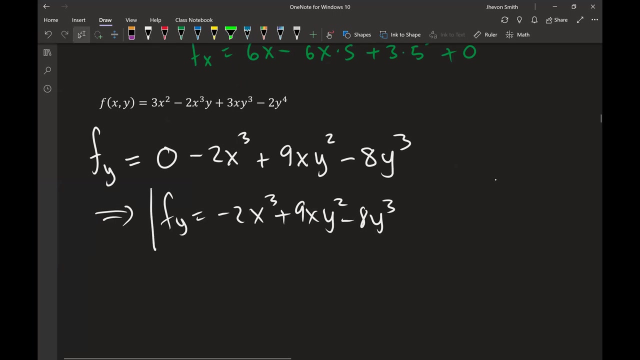 And then the last part is minus 8 times y cubed Correct. Okay, That's what I got in the first place. Is there anyone who's not getting it, Or do we think we know what's going on now? So it's when you want to find the partial derivative with respect to some variable. 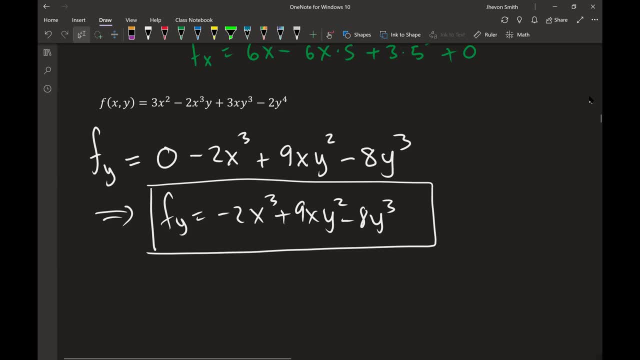 you pretend every other variable other than that one you're looking at is a constant. Now there are going to be times where we're going to have even more than two variables in play, So it's very important that you get this concept down: Every other variable except the one that you're taking the derivative with respect to, 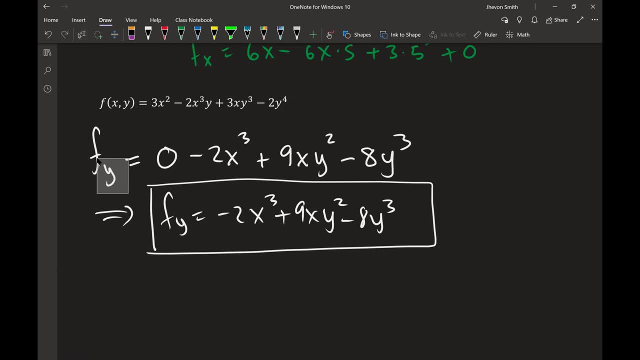 is a constant in your mind's eye, You treat it the same way you would treat a number. It doesn't matter if there were 10 other variables here. Everybody except y is a constant. Then you differentiate all the functions of y and you treat everybody else as if they were numbers. 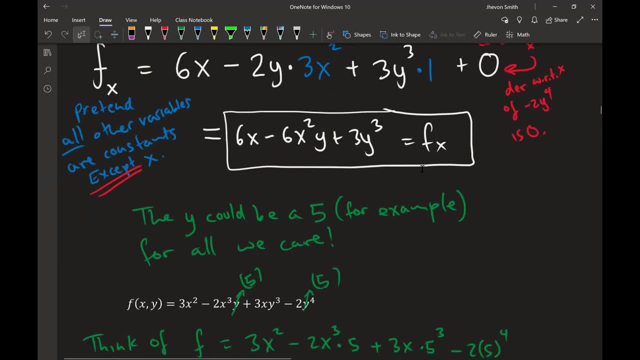 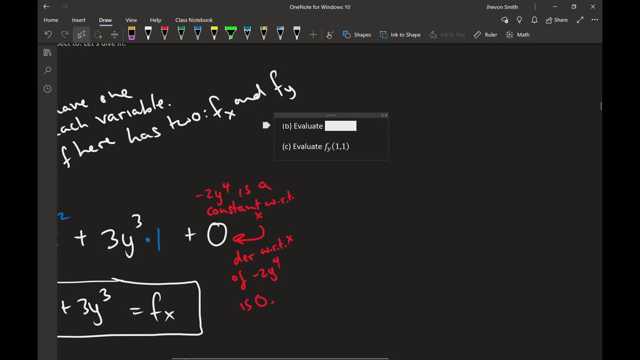 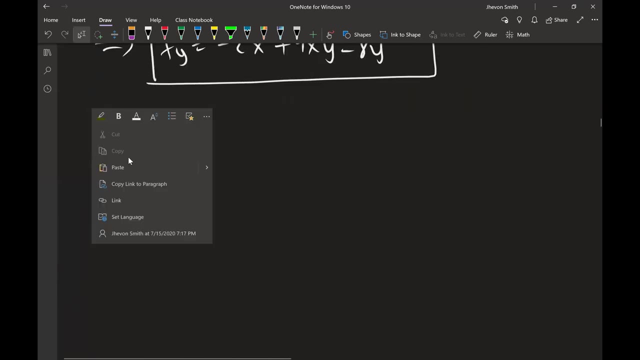 This is called a partial derivative. So these are the two partial derivatives of this function. Now, of course, once you find a partial derivative, you can treat them just as other functions. So, for example, if I went here and now, I ask you, well, evaluate the partial derivative with respect to x at the point. 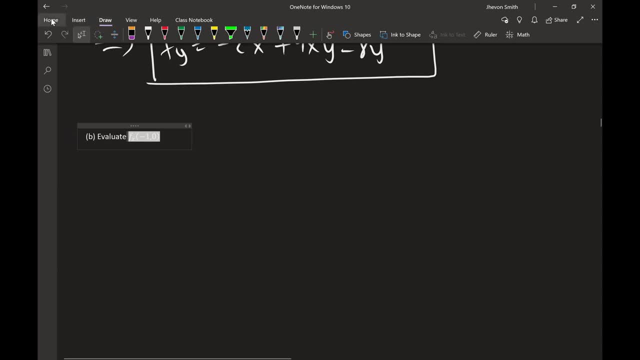 what was your reality If we take that as equals to the partial derivative of x, plus crossing cross over, which obviously is the angle that the partial derivative was compared to, Because ≤ y-y, but it was the partial derivative of x, so I". 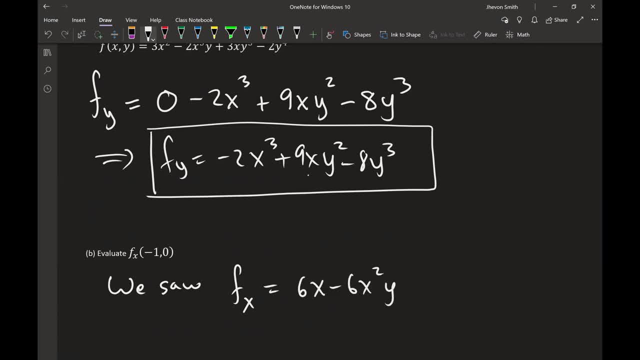 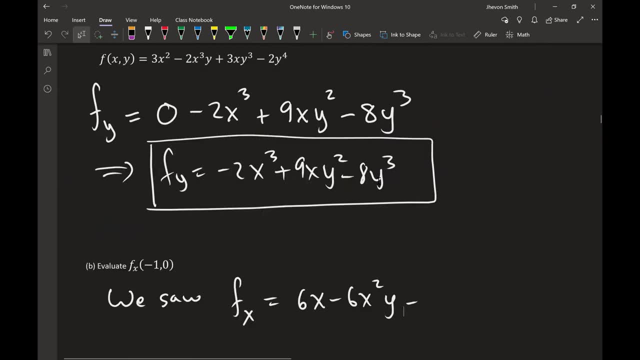 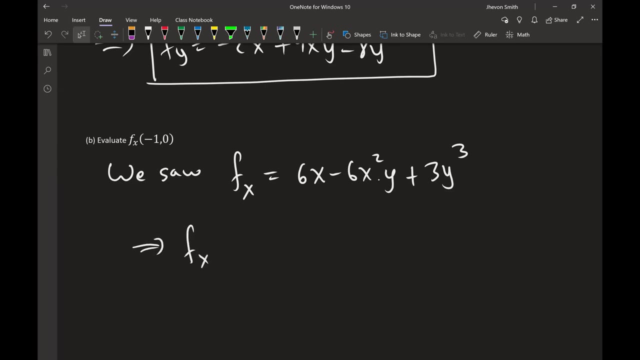 Now that's an odd Nai-Nai symptom because it's shared. I don't think it's fair that one could happen now. So that's an odd Nai-Nai symptom plus 3y cubed. So this means that if I take partial with respect to x and I evaluate it at the point, 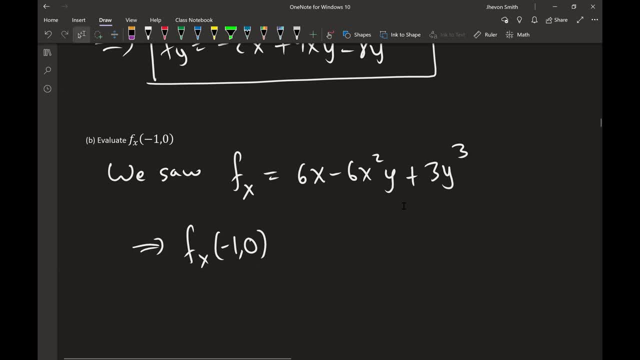 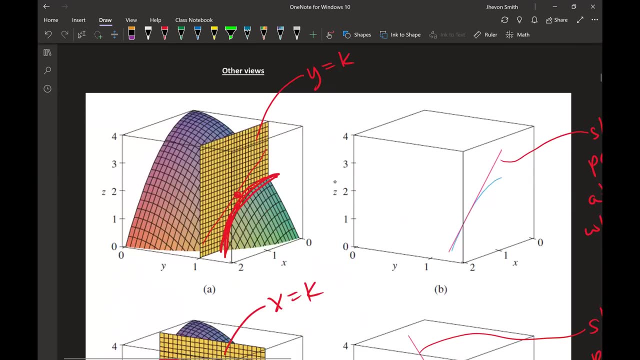 1 comma 0,. it literally means that I went to this plane. I looked at the plane y equals 0 and then I picked the particular point on that plane where my x was negative 1.. Right, So I slice through with the plane y equals 0. I go where x equals negative 1.. I find that. 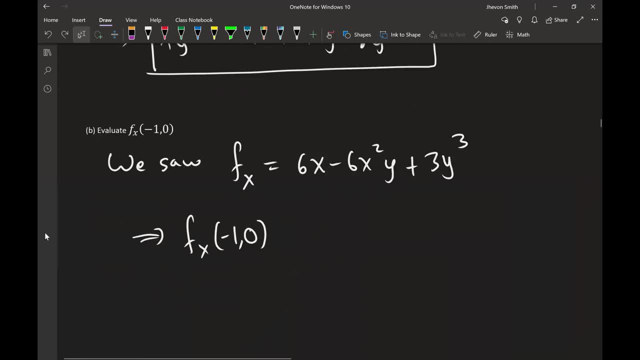 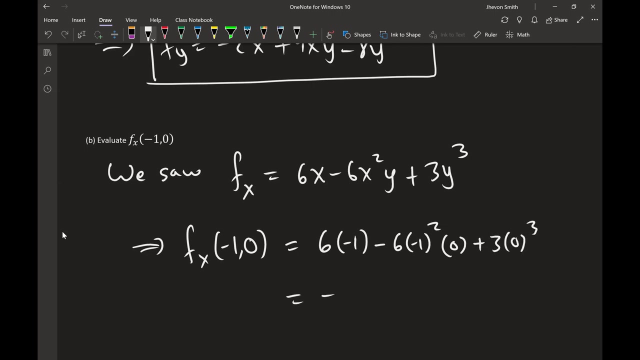 coordinate on that curve of intersection and then I evaluate the slope at that point. So I'm literally going to plug in negative 1 for x and 0s for the ys, And so that's negative 6, as Jason said in the chat. 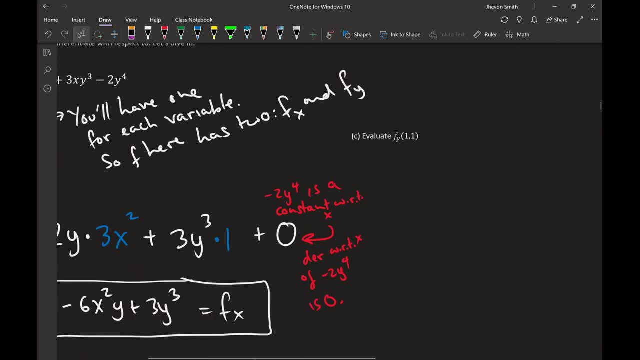 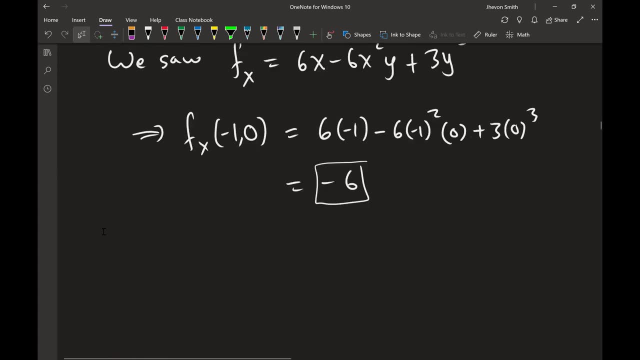 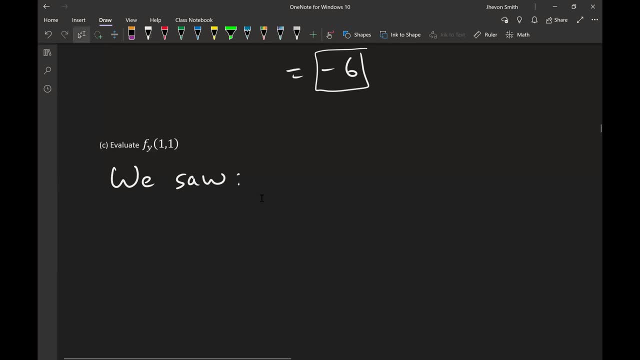 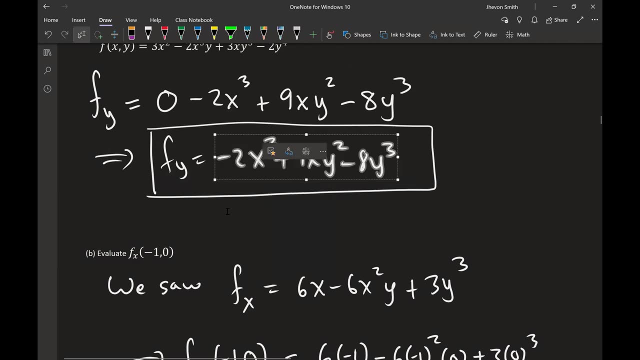 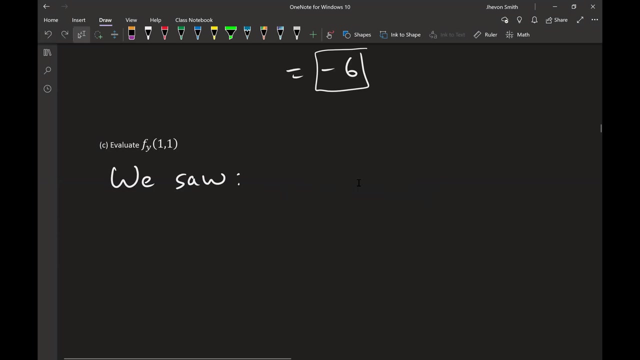 What's happening. We saw. I mean, this concept, I think, is much less confusing than the last concept, So I'm just going to do it. We have a lot more interesting stuff to get to, So let's actually just move on with our lives, Okay? So we saw. 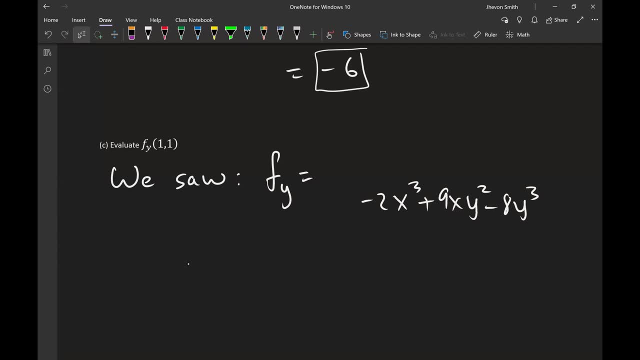 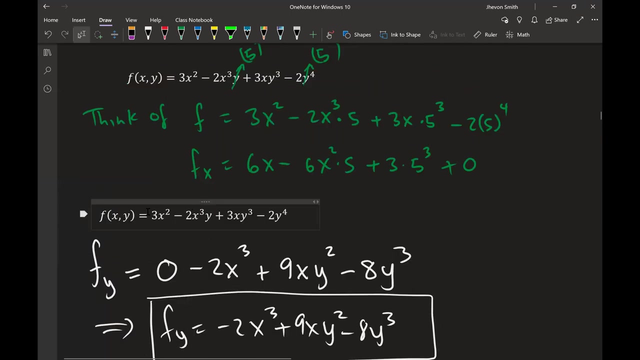 we saw, partial with respect to y was equal to this guy. So that means I think of my x as the plane. x equals 1. slicing through I would get a curve of intersection between the surface of whatever this graph looks like. It's going to look crazy. I can tell you that You can plot. 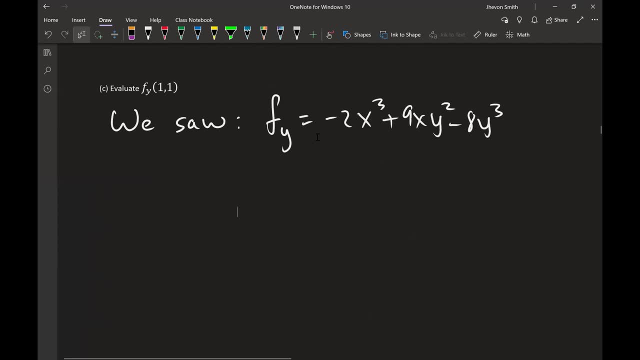 this later on in the in the website that I gave you. You can plot this in the website that I gave you to see what it looks like. but then slice through that guy with a plane: x equals 1, then find the coordinate where y equals 1, measure. 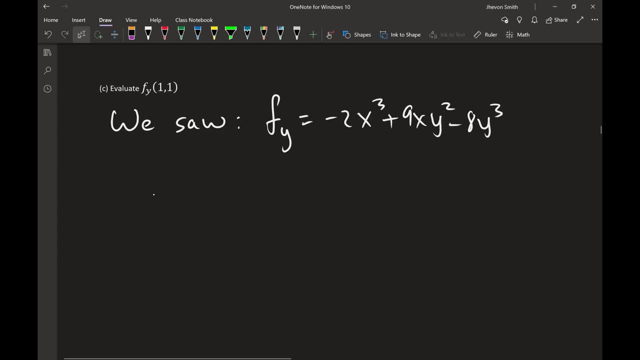 the tangent line there? What is the slope? That's what this question is asking. So this would mean that my partial with respect to y at 1, comma 1 is just literally just go in, plug in 1 for for x and x and y, So that's going to be minus 2 plus 9 minus 8.. So you get. 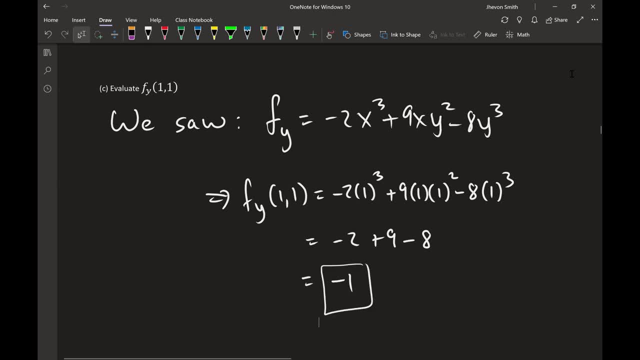 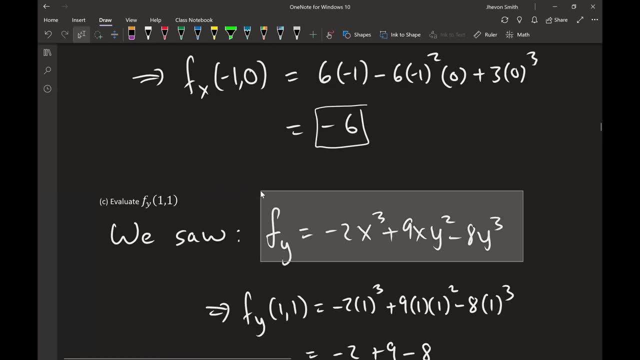 negative 1.. Alright, so hopefully that was clear. I mean finding the partial derivative is the. is the quote-unquote harder part? Plugging in the numbers should be relatively easy. Whatever is in the x-coordinate, plug it in for all the. 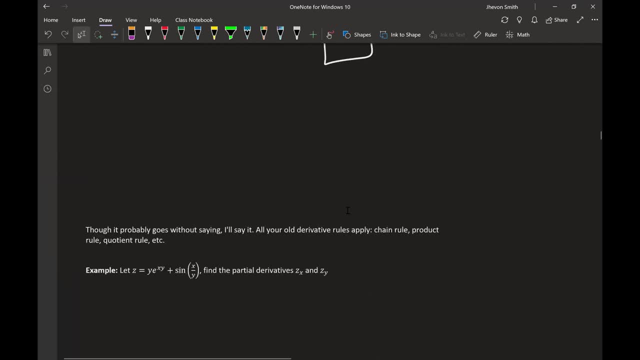 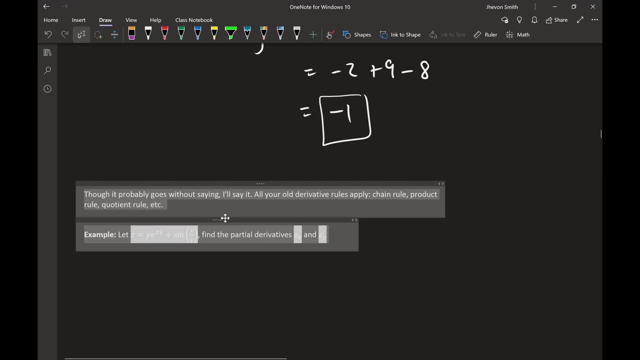 x values. Whatever is in the x-coordinate, plug it in for all the x values. Whatever is in the y-coordinate, plug it in all the y positions, etc. Alright, now I do want you to be aware. Let's make this a little bit harder, a little bit more. 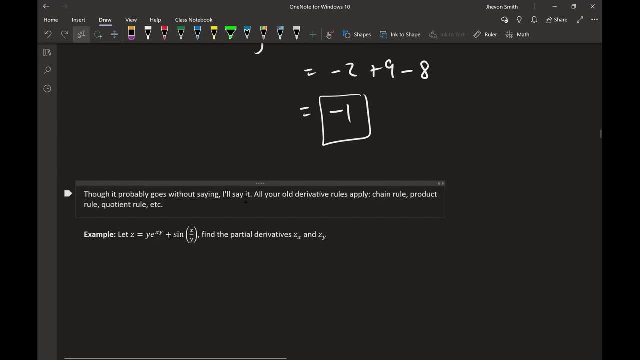 general. All your old derivative rules, they apply. Product rule- still a thing. Chain rule- still a thing. Quotient rule- still a thing. All of that stuff still a thing. Okay, so let's say I have this function. 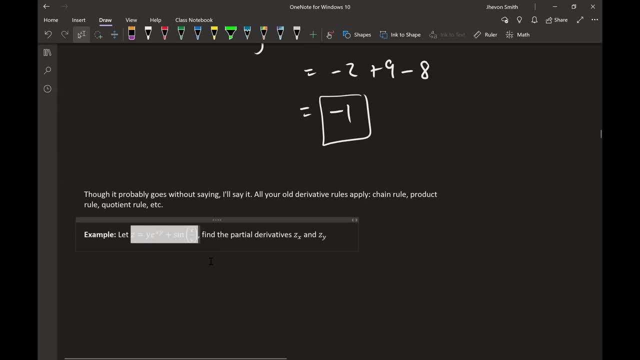 right here. Let's just actually jump into this and start finding partial derivatives. Let me make this a little bigger so you guys can see. Alright, so I want you to find the partial of Z with respect to X and I want you to find the. 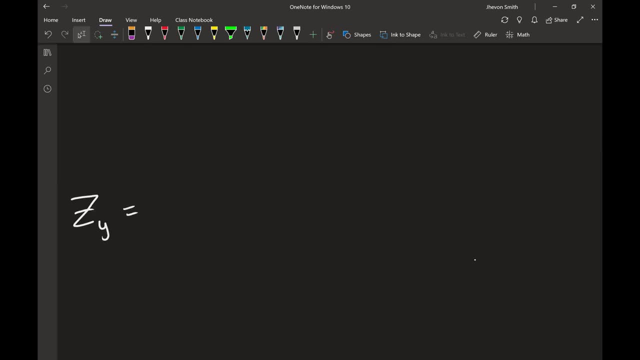 partial of Z with respect to Y and very glad that I've got these closed in order. Abdulrahman volunteered here. Who else can I call on Who's usually chatty, that there have not been very chatty so far? Now, the shy people do need to get out of their shells. 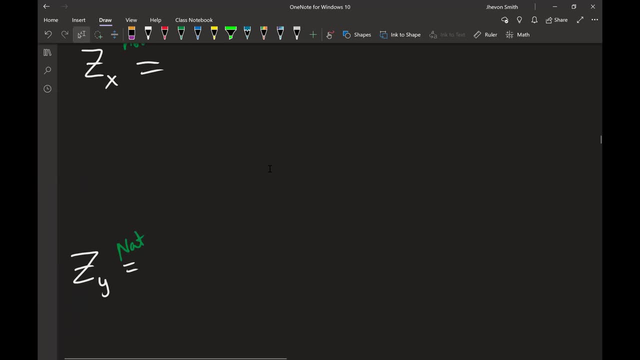 but sometimes calling on them right away is not so nice. They need to work on their shyness first. Abdulrahman, are you there? All right, tell me what's the partial of this guy with respect to x? Here's the function. 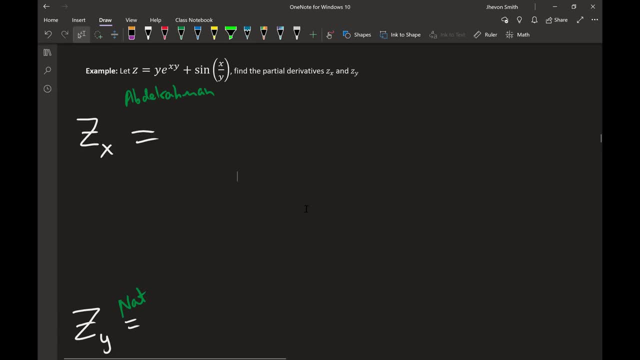 y times. e to the xy, plus sine of x divided by y. Natalie, start working on the partial with respect to y of that guy. No, Wolfram, because I know I can't see you guys. Come on, What about the first part? y. e to the xy. 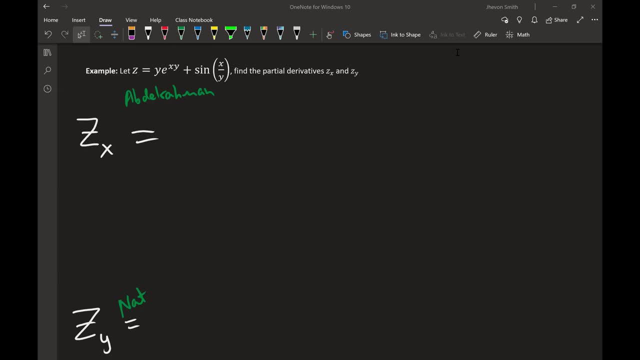 If I differentiate that with respect to x, what do I get? And, by the way, the rest of you should be doing this, Even though I didn't call on anyone specific. everybody should be writing down what they think is the answer. It's very important. 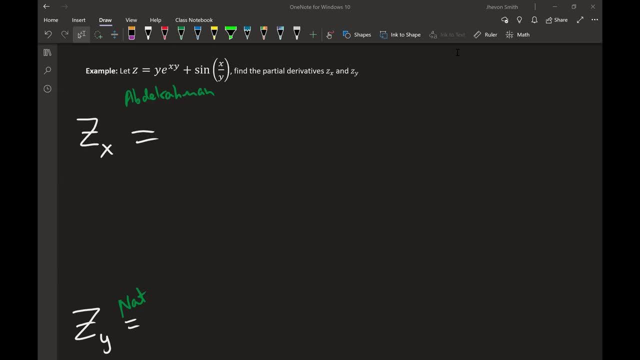 More important than you realize. If you just watch it- even if you watch me do stuff or you watch someone else do stuff and it makes perfect sense- it does not mean that you would be able to reproduce that thing on a test. You will never know what you're able to do unless you actually 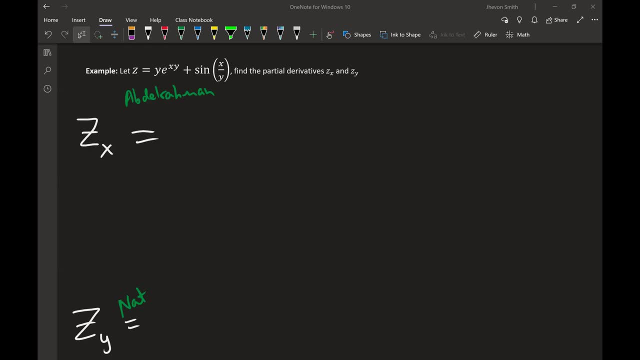 do it. OK, All right, And then what would you get? I don't know. Are you there? Oh Geez, sorry about that. I was literally here waiting and I'm like: what has taken Abdulrahman so long? 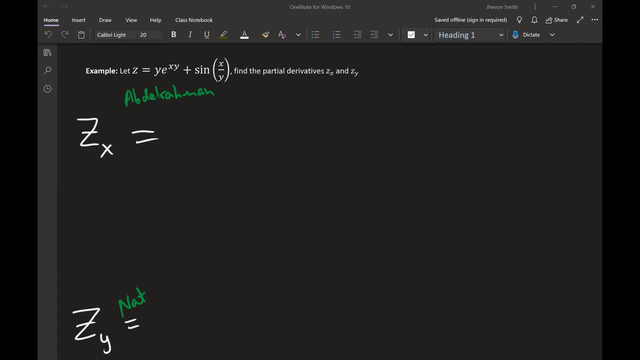 And I'm thinking he's stuck and it's just. my internet went out. You made me host again. again, i didn't make anyone host. it randomly picks someone, i don't know why, and it always picks me. well, i, i don't, i, i can't explain it. 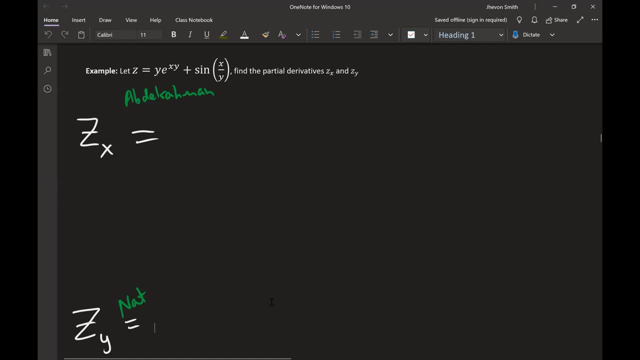 it knows you're the reason, probably. anyway, uh, let's jump back into it. so, um, when is uh? what is uh? partial respect to x? okay, so the y in the front, we would more, since it's a constant, yeah, and so we would get the derivative of e, x to the y. 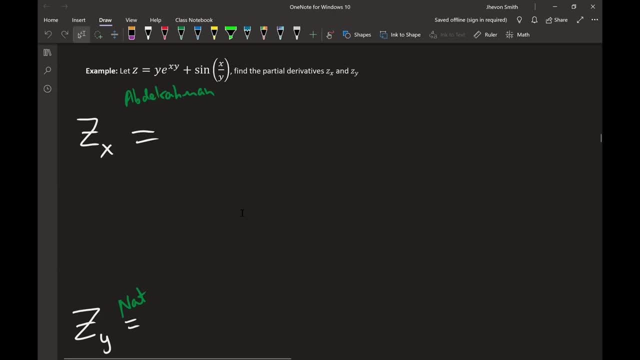 but we'd make a, l and y equal k, okay, so what would the derivative look like? be y times e to x, y, right? so remember, our general rule would be the derivative of, if we're- and now i'm thinking of- single variable calculus. you see how i write. 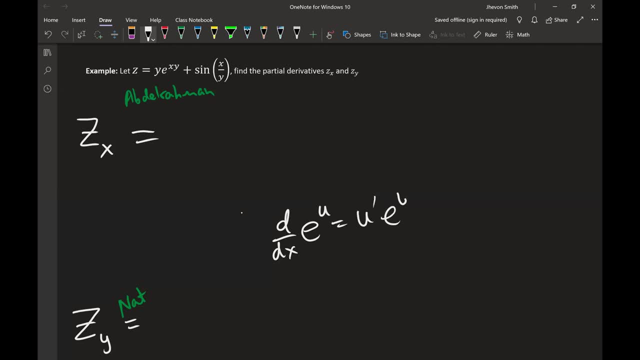 the d right. so we would get the derivative of e, x to the y, but we would make a, l and y. the derivative of e to the u is what u prime, e to the u. so i just want to take the derivative of the power times, the original function. 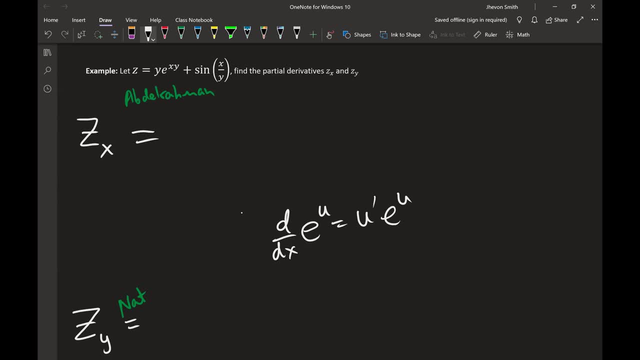 now the derivative of the power with respect to x is just y, so i would have another y. so in other words, here i have a y times y, e to the x, y. right then, um the sine function, so um the derivative of sine would be cosine and um we would leave the inside as it is, and 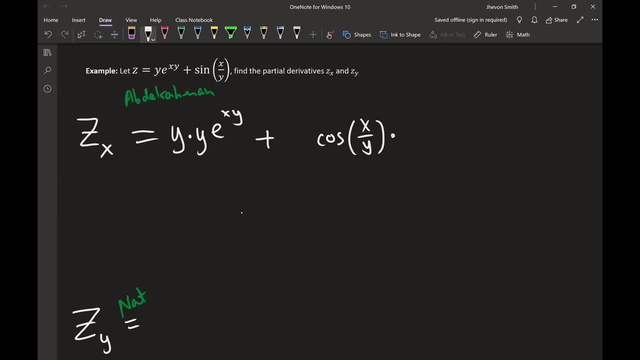 then we would um multiply it to the derivative of the inside, which is y is a constant, we would leave it on the denominator, and all of x is one, so it'd be times one over y, right? so chain rule here. so you use the chain rule for both of these. so 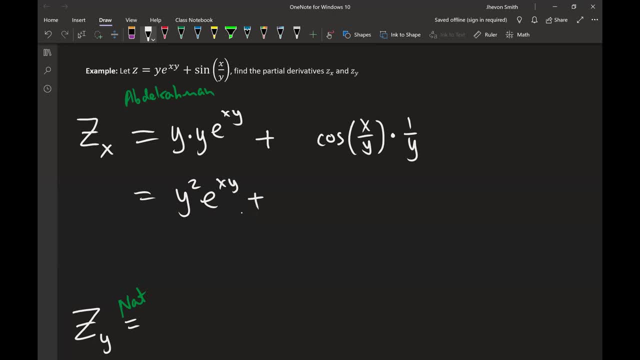 y squared e to the x y plus one over y, cosine of x over y. right and notice that, uh, what we're using here is a chain rule. the same thing here is a gain rule. same thing here as well. actually, it's a product rule. Uh, we didn't need the product rule here. 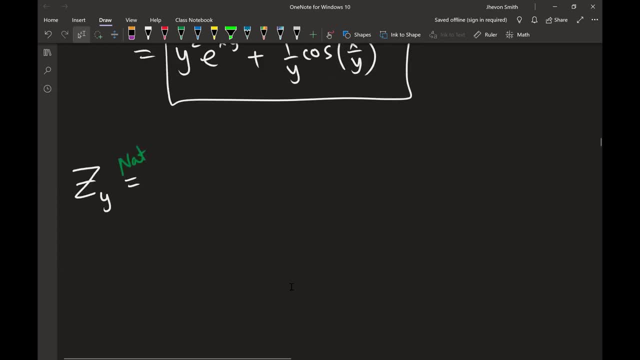 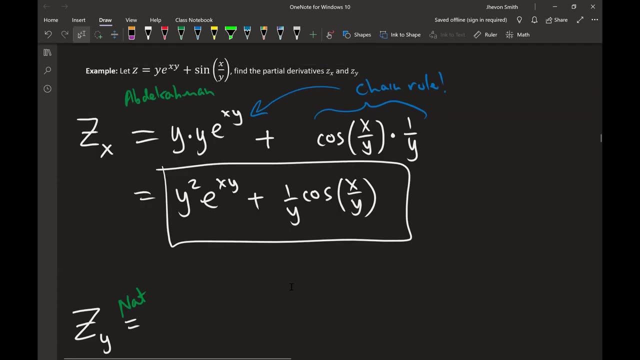 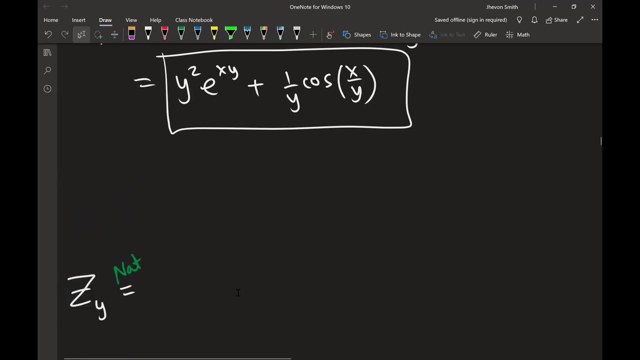 Uh, we needed for the part with respect to y, though, Natalie, did you finish that? Yeah, So for the first part, looking at it, looking at it with respect to y. So I got e to the x, y plus x to the e, sorry, x times e to the x, y times y. 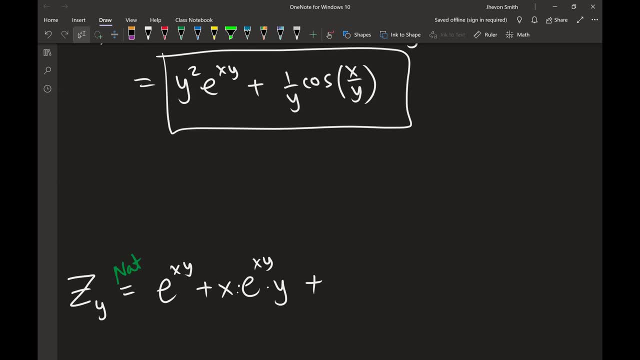 And then for the second part it was a chain rule. So I got plus cosine x over y in the inside times negative x y. I mean not times negative x over y, squared Right. So here our z was y, e to the x, y, plus the sine of x over y. 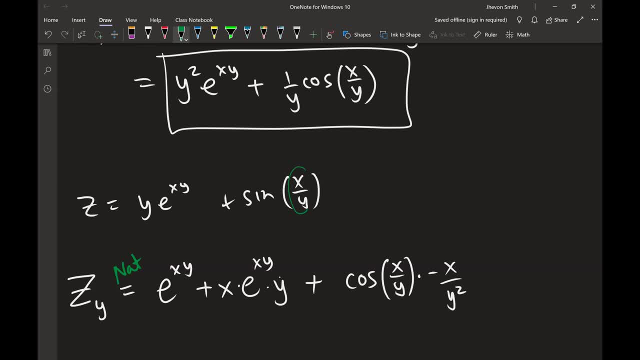 And again, you can think of the, the inside here, as x, y to the minus one. So the derivative of that is going to be minus x, y to the minus two, which is what that that guy is. But here what we did is we use the chain rule. 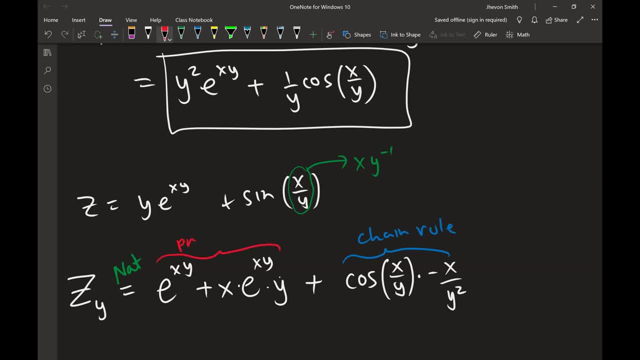 And here what we did is we use the product rule, Because here I have two functions of y: e to the x, y is a function of y and y is a function of y. So I have to differentiate one, leave the other, then leave the first, differentiate the other one. 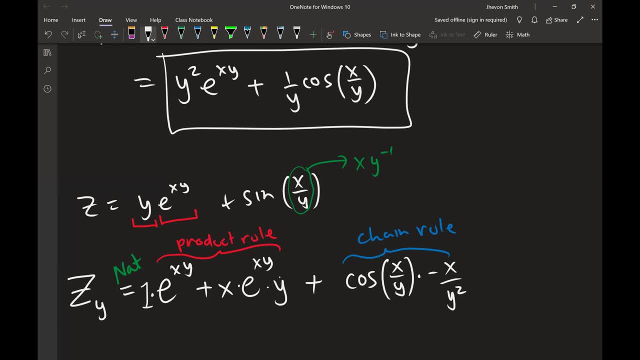 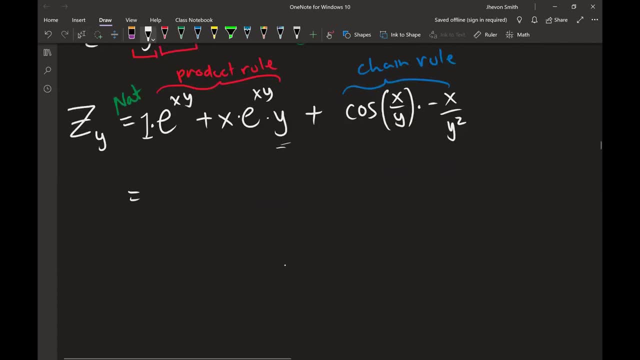 So I differentiate the y and you would get here the one, Then you leave the y, which is here, and then you differentiate the exponential So that you can actually clean up. Yeah, So e to the x- y plus x, y, e to the x- y minus x. 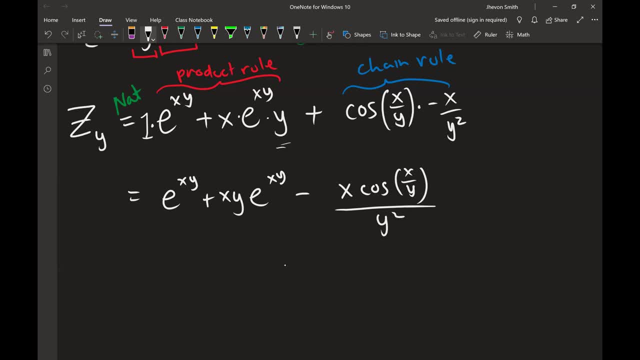 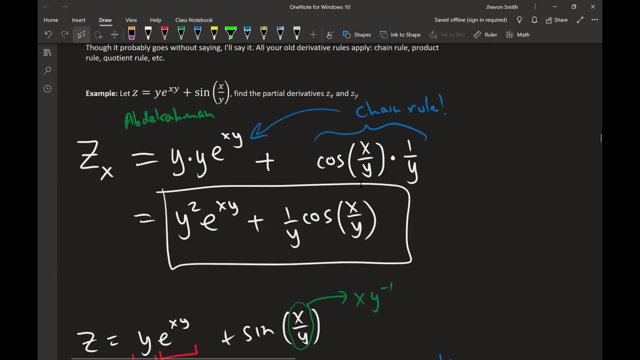 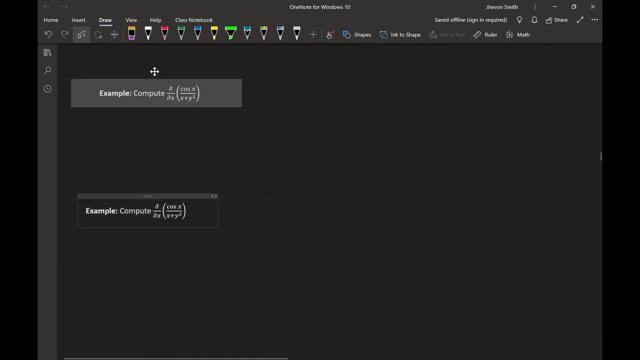 Right, And that's your partial respect to y. All right, good job people. All right, let's move on. That's what I got, like you know. thank God, I got it right for the two- both of them. 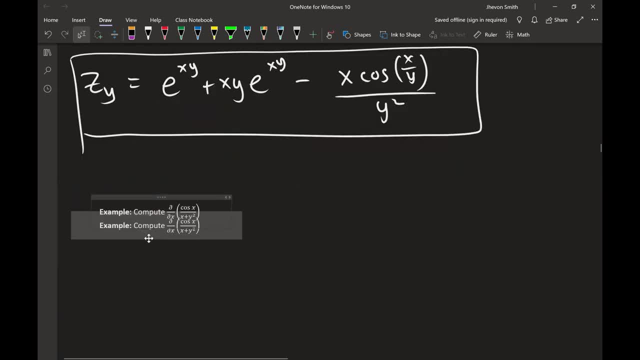 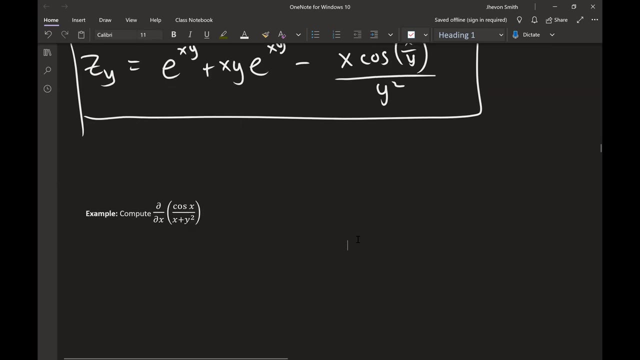 Yes, I know, Jason, I know. All right, here's another one, And at this point I'm not teaching you anything new. I just want you guys to get a lot of practice. All right, Jason? partial derivative of that with respect to x: go. 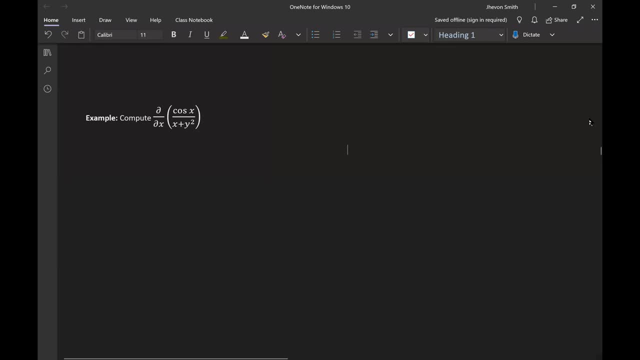 All right, Let me take some time to solve it, then I'll announce it. Yeah, I couldn't even tell that Natalie had social anxiety, so I don't know. It's not what she's saying in the chat, It's fine. 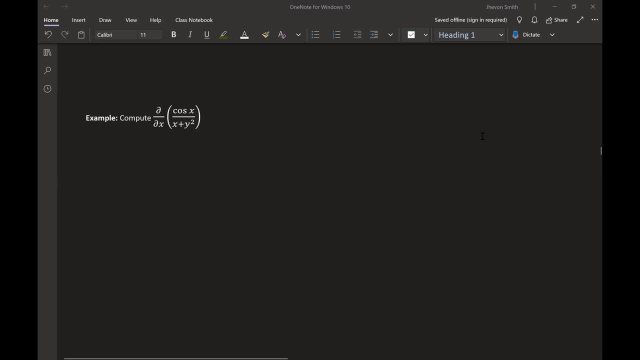 Okay, Natalie's probably a very tough opponent to play in poker because she says she's nervous, but at the same time her voice didn't crack nothing. There was no indication- Like there's no indication- of anything stirring below the surface. 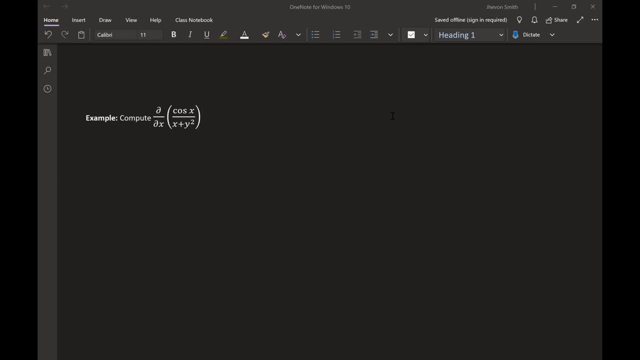 All right, Anyway, the rest of you should be trying this as well. partial derivative, with respect to x, of cosine divided by x plus y squared. All right, Jason, I'll give you another 30 seconds. According to what I'm assuming, I would say, like you know, parentheses negative sine. 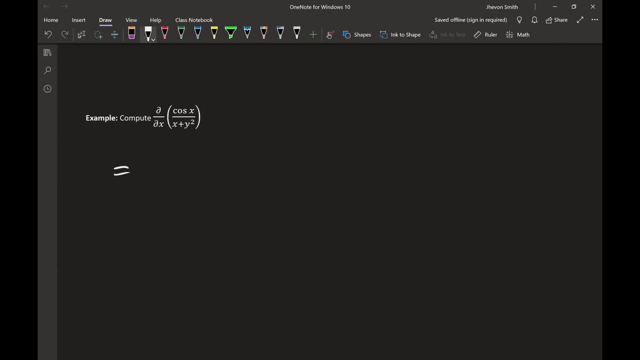 x times parentheses X plus y squared. subtract cosine x over parentheses of parentheses x plus y squared, you know, to the square power. Okay, yeah, so we need the quotient rule. so it's the bottom times the derivative of the top minus the top times the derivative of the bottom over the bottom squared quotient. 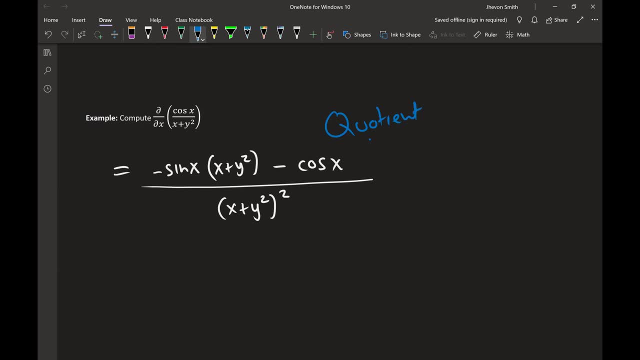 rule. That was right. Well, yeah, That's what I had. Okay, All right, I had an idea This would be the answer And he's like, well, yeah, yeah, of course I mean what. 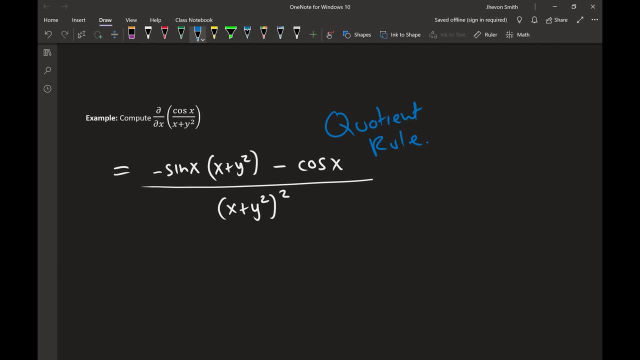 You didn't expect me to get it right, Okay. so, yep, that is quotient rule. Okay, good, We can move on Now. I wanted to be aware that implicit differentiation also a thing that can be used. So sometimes we don't just have our z equals some f of xy. sometimes our z is kind of mixed. 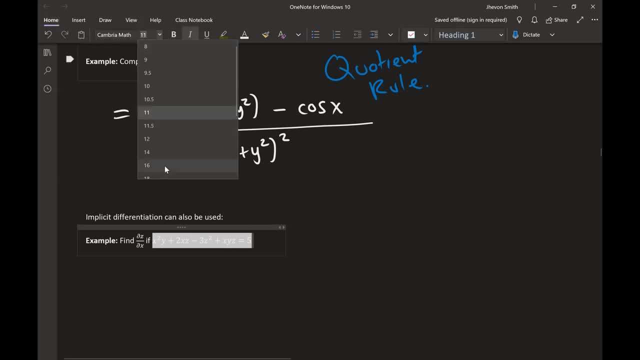 together with everyone else, And this is in a situation- this gives us a situation where we need implicit differentiation. So here I am thinking of my z as a function of x and y, but it's kind of mixed up with the x's and y's. 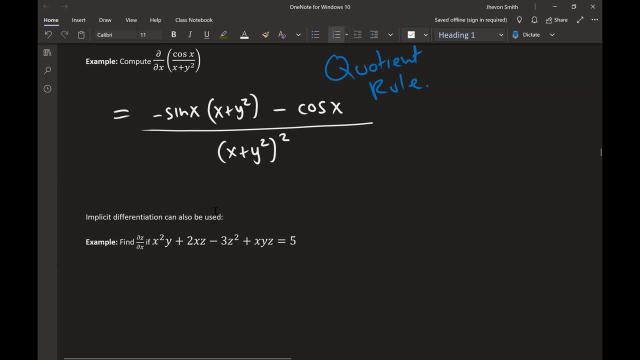 We can actually go through and start finding derivatives here, in the same way we did implicit differentiation. Now there's gonna be a really neat trick that I'm going to show you guys, And it's gonna be an interesting one. It's going to be like when you see what I'm about to share. 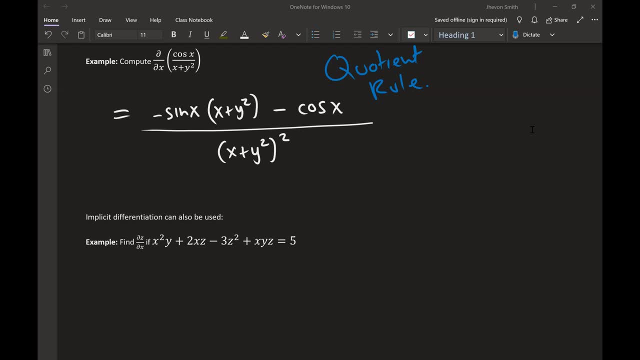 this example right here, this one right here. you see this right here. This one is going to be a very nice example, Cause now you're gonna realize that you could go back to calc one and you're going to be able to use this trick. 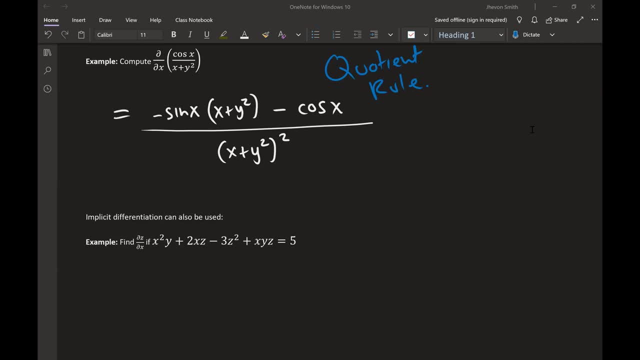 that I'm gonna tell you, And you could have done implicit differentiation in calc one so much easier. But for now let's actually go through with our calc one brain and kind of work out this problem. So here's what it would look like. 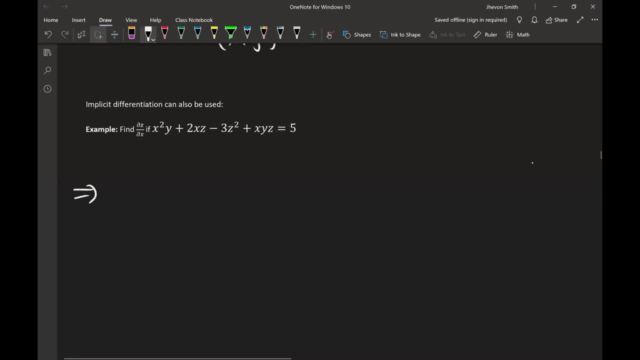 So you would go through and again you would differentiate each term with respect to X. Now, whenever you differentiate a term that again think of Z as an inside function. Hopefully you guys remember how implicit differentiation work from calc one. I'm not gonna do that. 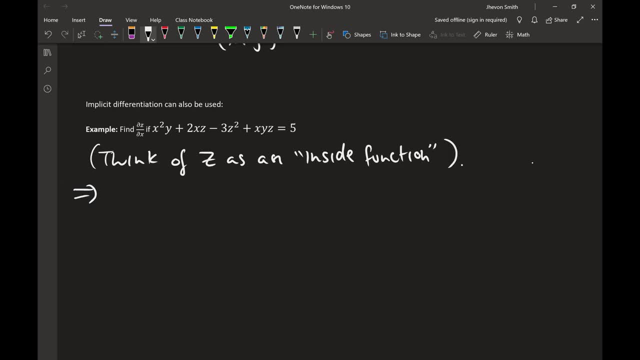 Okay, So, okay, Quick refresher from calc one. So let's say you had X, Y cubed, minus Y squared plus X equals seven, And you want to find, find D, Y, D, X. So let's see an example from calc one. 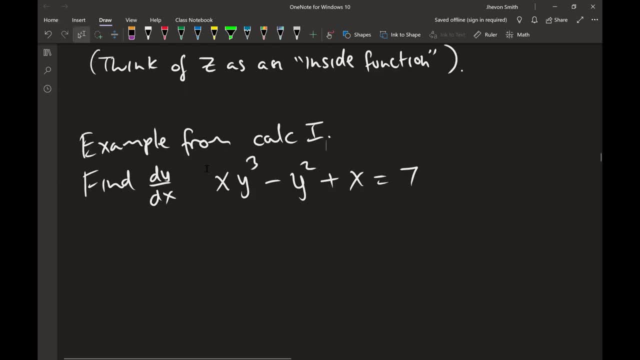 What did we do? Well, you went through and you differentiated each term. However, you just had the awareness that whenever you were differentiating a Y term, you had to multiply it by the derivative. So, for example, you would have go through here: 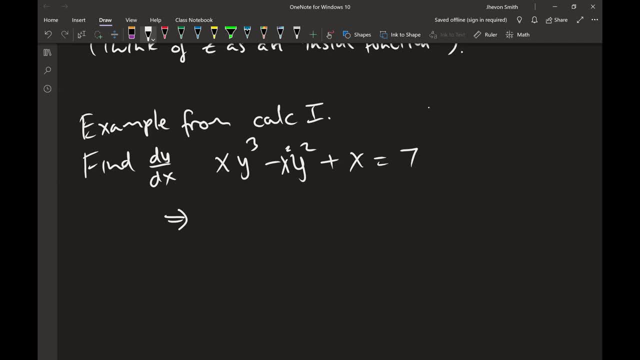 I'm getting a message saying my internet is unstable. Are you guys still hearing me? Someone, just give me a check. Okay, All right, All right. So here you go through and you differentiate. You would here, you would think of X and Y. 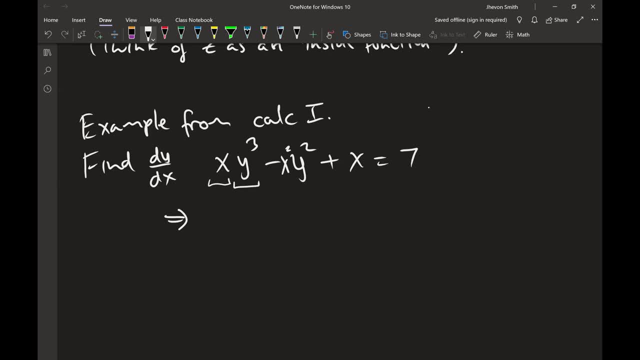 as both functions of X. So now you have to actually do the product rule. So you differentiate the X, you would leave the Y cubed, Then you would leave the X and you would differentiate the Y cubed, But because the Y was a function of X. 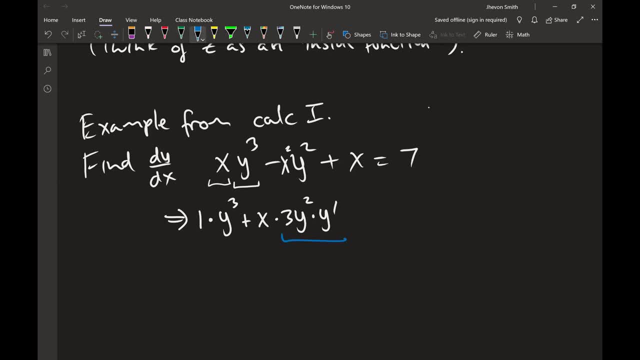 you have to multiply by Y prime. So here you apply chain rule, because Y is an inside function. It's some function of X, but you just don't know what Right. So this means that when you see Y cubed it's really like there's some F of X cubed. 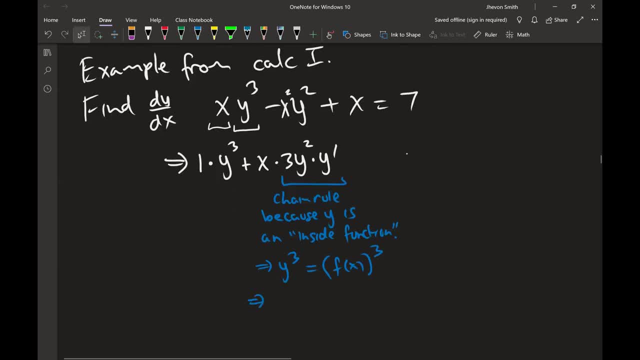 And so when. and so this means that the derivative with respect to X of Y cubed is going to be the derivative with respect to X of some function cubed Which is going to be chain rule. differentiate the outer function, multiply by the derivative of the inner function. 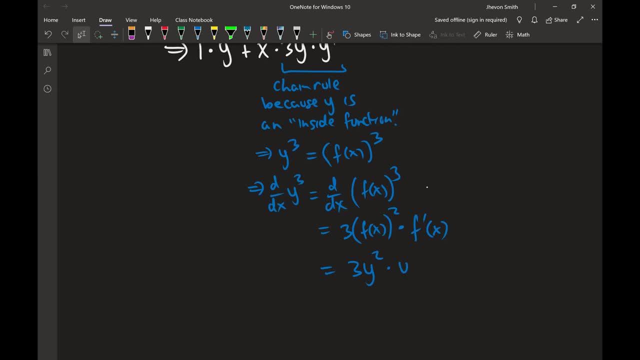 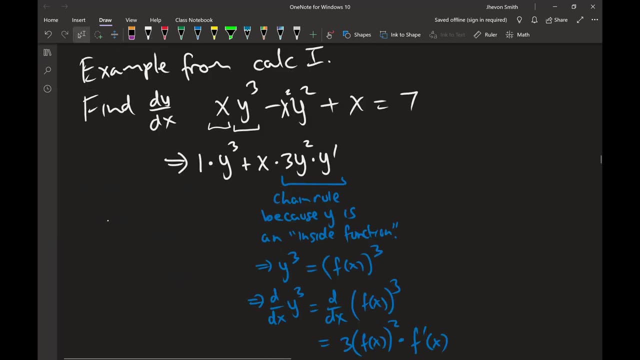 And so that would give you the three Y squared times Y prime, And that's where the Y prime came from. So now you do that for the rest of them. So you go through, differentiate the X, leave the Y plus. you leave the X, differentiate the Y. 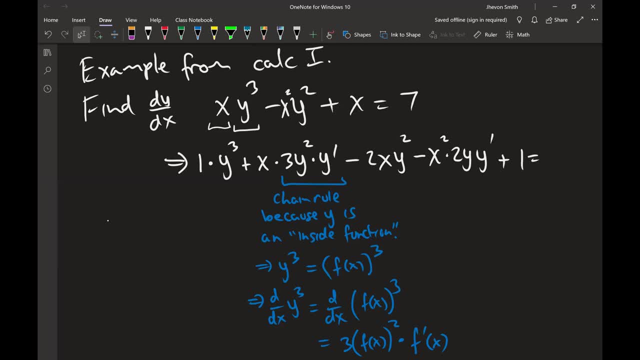 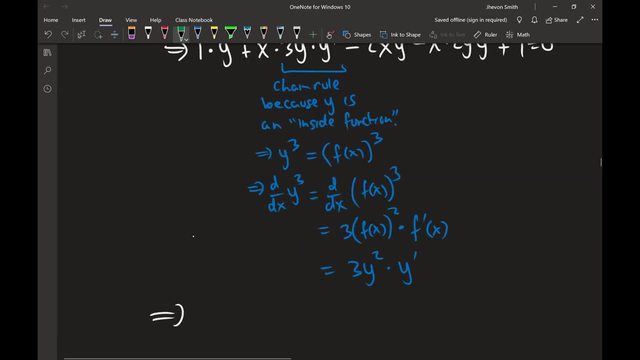 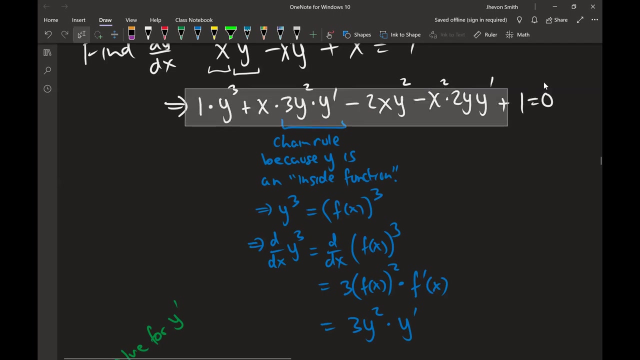 multiply by Y prime Plus derivative of X is one, derivative of the seven is zero, Then what you're going to do is, at that point you solve for the Y prime. So we'd go through here, Uh, just copying it down. 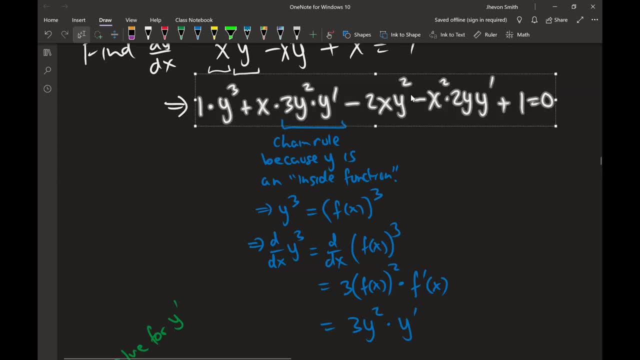 So I'm just going to copy it down. So I'm just going to copy it down. So I'm just going to copy it down. So I'm just copying it down. So I'm just copying it down here so I can see. 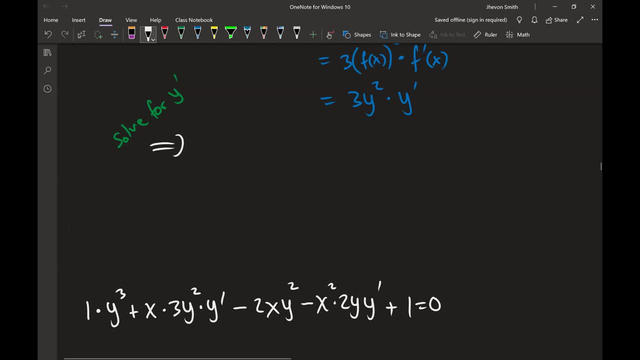 Then we'd go through here and we'd group all the guys that have Y primes and factor it out. So here I would have three X- Y squared That takes care of this guy. Then I would have minus two X squared Y. 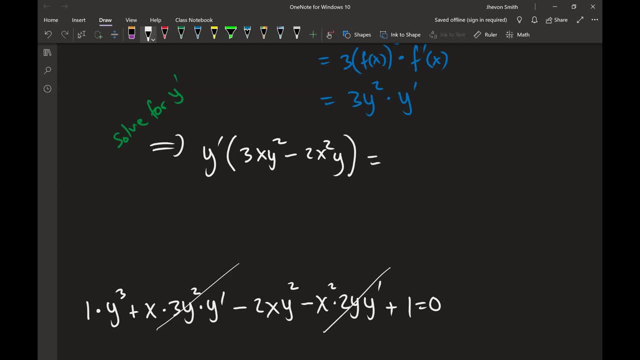 That takes care of that guy. Those were the guys with derivatives in them. We'll move everyone else to the other side. So here I'd have minus. let me open brackets. You would throw in the Y cubed. That would be this guy. 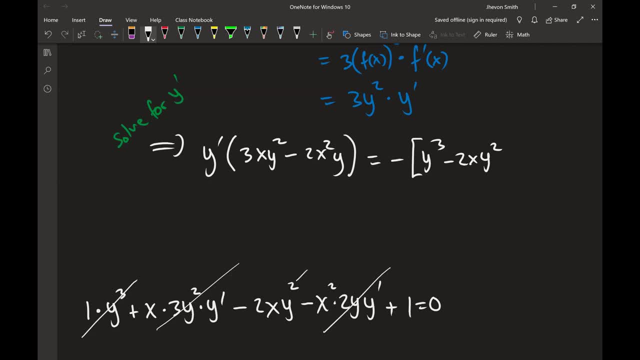 Then you'd throw in the two X squared, That would be this guy, Then you'd throw in the one, That would be that guy, And then you would say: Y prime is equal to well minus well Y cubed, minus two X Y squared plus one. 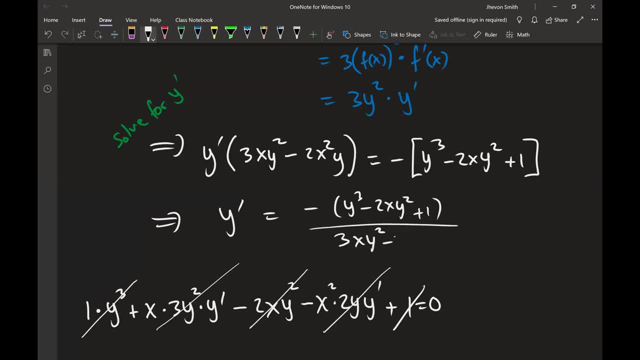 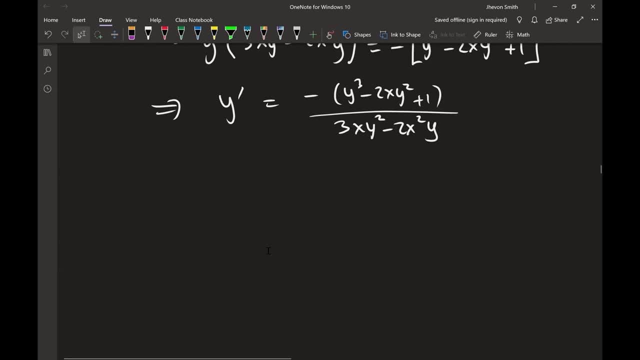 divided by three X, Y squared, minus two X squared Y. So that's what we'd get, So quick crash course in implicit differentiation from Calc one. You guys should have been experts at Calc one, so I'm not going to go any further into that. 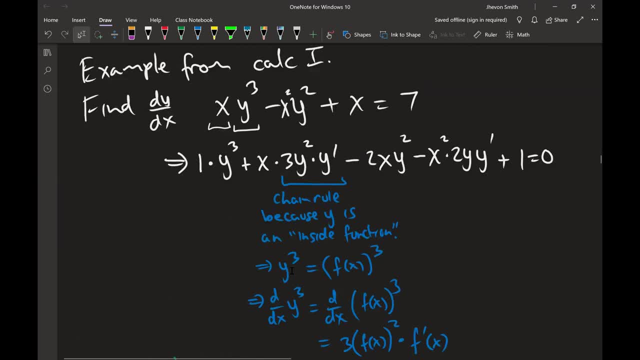 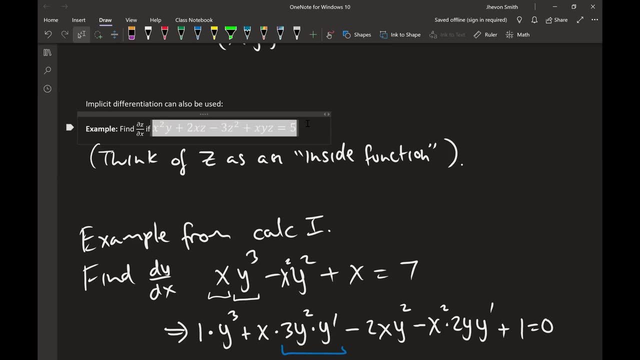 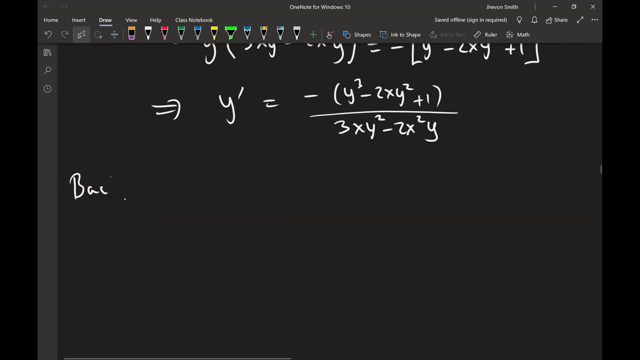 We're going to come back to this and I'm going to give you the red pill, But right now let's actually continue. So I want to do that similar process here. Okay, Okay, Okay, Okay, And then again. 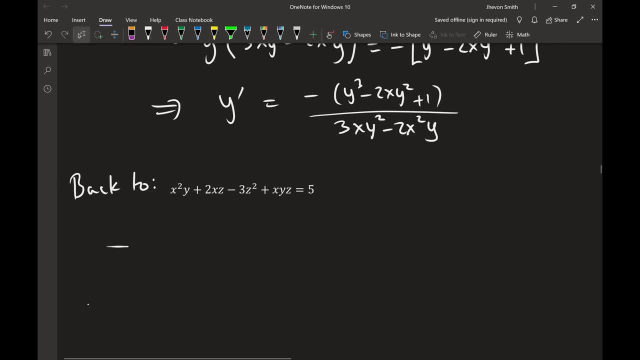 I'm just going to go through and I'm going to find the partial derivatives. So here I start by the first term: X squared Y. I need to differentiate that with respect to X. Well, that's two X, Y, Cause my Y is a constant. 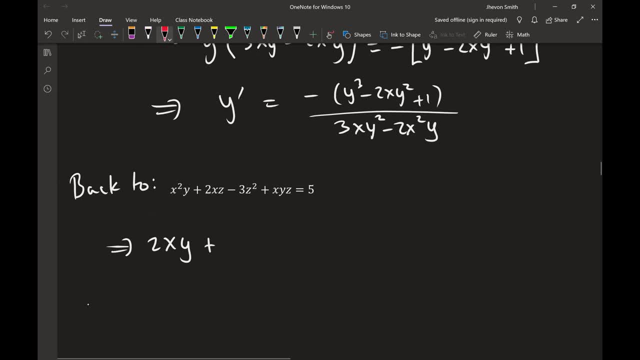 Plus. now I move to this part here- the two X Zed. I think of my Zed as an inside function, though, because that is the dependent variable, which means there are potentially XS that are mixed inside the Zed. I just can't see them. 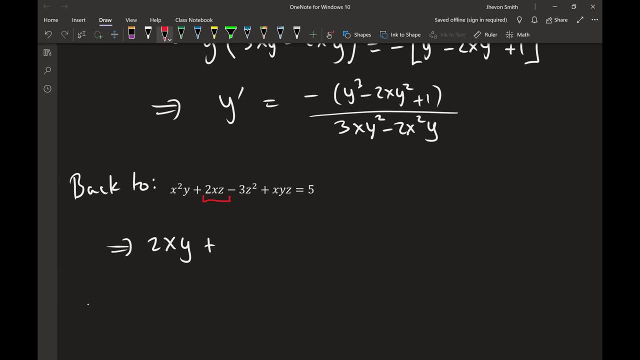 Which means I think of these two guys as being functionals, functions of x, and I need to do the product rule. So I would differentiate the x, leave the z plus. leave the x, differentiate the z, but now that is partial of z with respect to x. 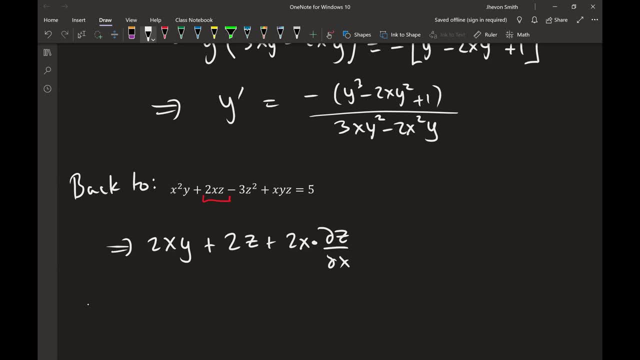 I don't use z prime because prime is too vague in the multivariable case. I'm using the Leibniz notation, So now. so for this I would need the product rule, because z is a function of x, specifically, and y. 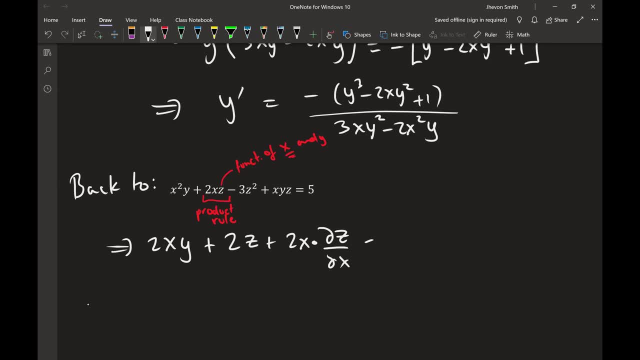 All right, so now I continue like this. Take the derivative of three z squared. Well, that's going to be six z times the partial of z with respect to x, Then again. so here I need the chain rule, And so that's this term here. 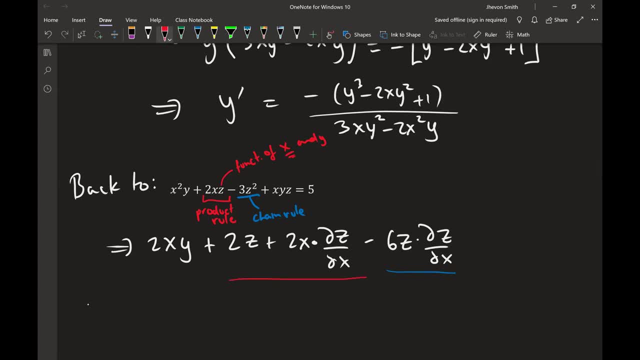 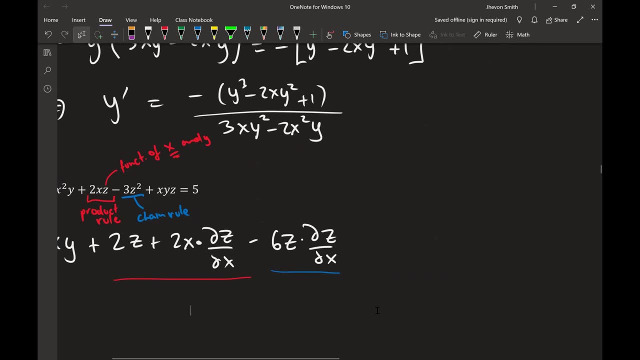 Product rule was this term here. Now, if I move on to the last term- x, y, z- I would need another product rule. I would then go: differentiate the x, leave the y and the z, plus, leave the x and the y, differentiate the z. 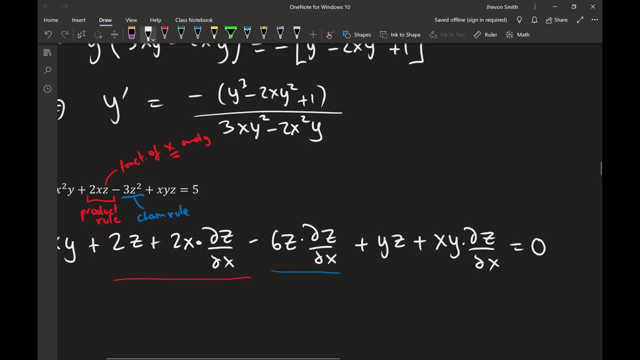 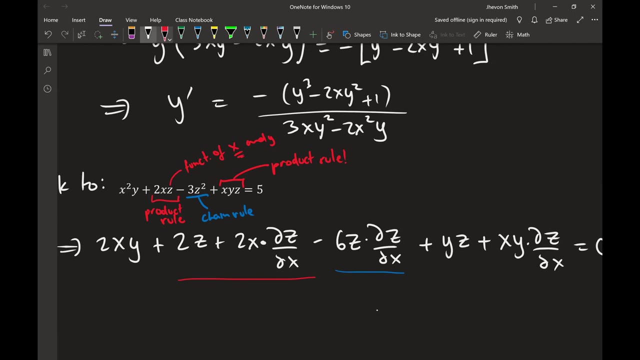 partial of z with respect to x. Derivative of five. z squared five is zero. So again here I need another product rule. Now we have our derivative being taken. Now what I do is again we play that same game. 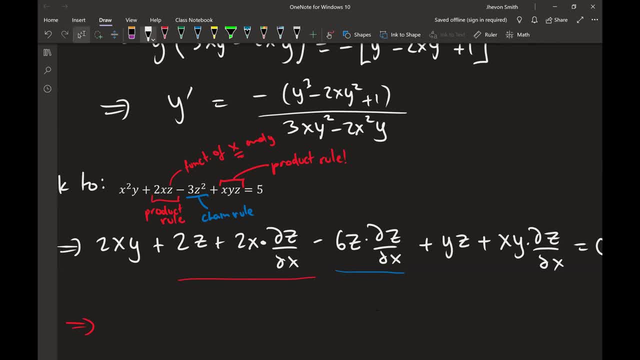 I group, all the guys with the I group, all the guys with the partial. with respect to z, I would have two x. I would take care of this guy. I would have minus six z. That would take care of this guy. I would have plus x- y. 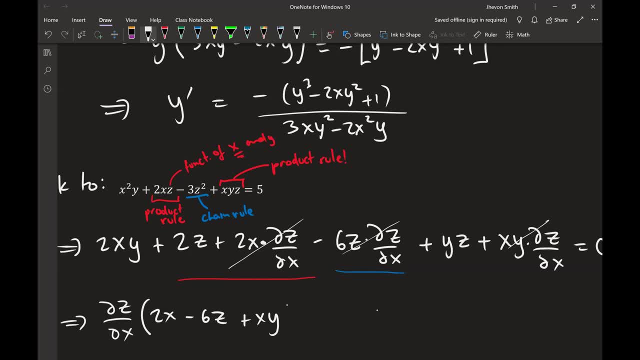 That would take care of this guy. That's all of them. Then I would move everyone else to the other side. So the two x- y takes care of this guy, The two z takes care of this guy, The plus y- z takes care of this guy. 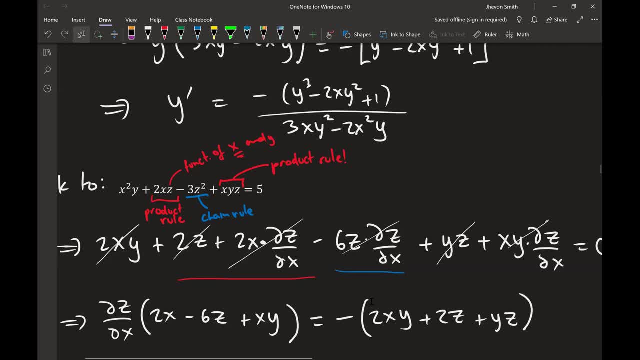 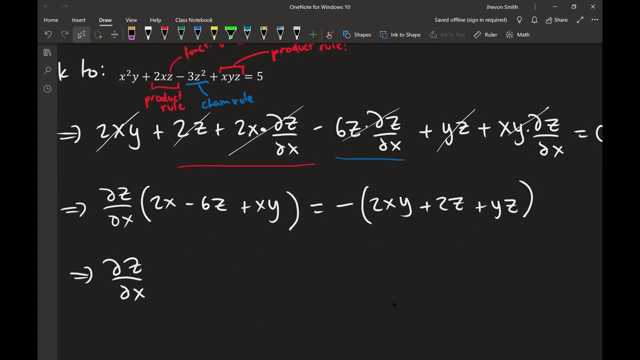 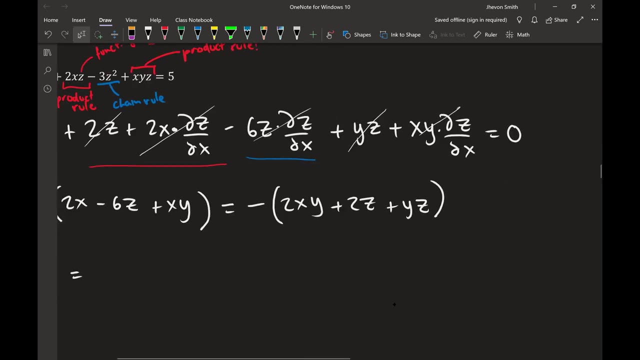 And that's that's it Now. what we have is: I can just divide both sides, Professor, wouldn't it be equal to plus five? Because where did the five go? I differentiated. Derivative of five is zero. Derivative of five is zero. 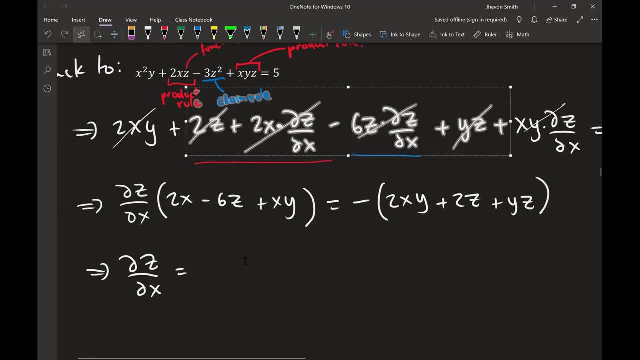 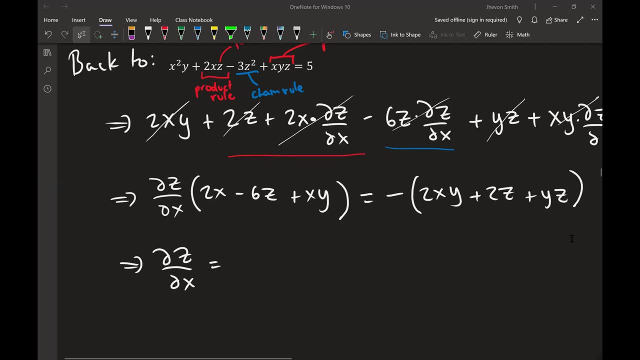 Right, Like this line here that I did all the strikethroughs, I'm taking derivatives, So there is no five. Okay, double checking. Can you guys hear me? I'm just suspicious that I'm losing connection again. We can hear you. 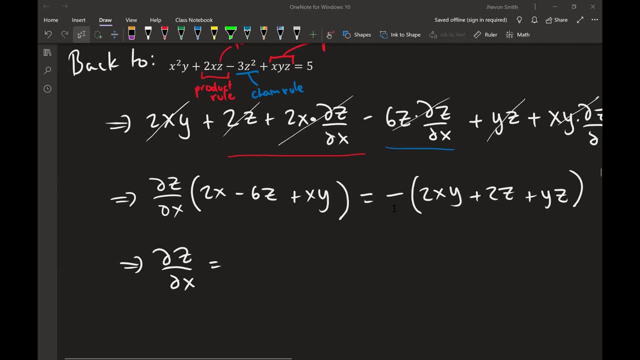 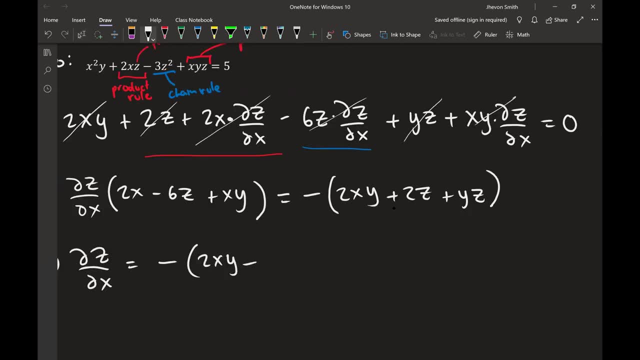 Okay, All right, good, So the derivative of five is zero, So that's why it's not there. Now I just do this divide. So this is this: This over two: x minus six, z plus x, y, Right? 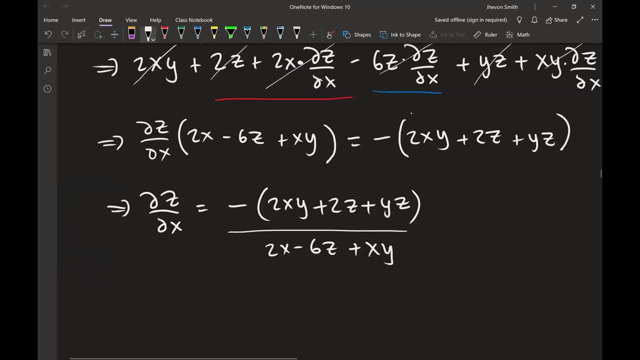 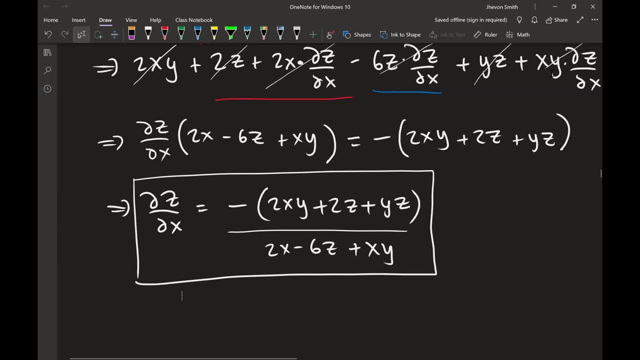 So that's our derivative with respect to x. implicitly. Okay, Now you guys ready for this? Are you ready, though? Are you guys ready? If you're not sitting down, sit down. Okay, Here's what I want you to notice. 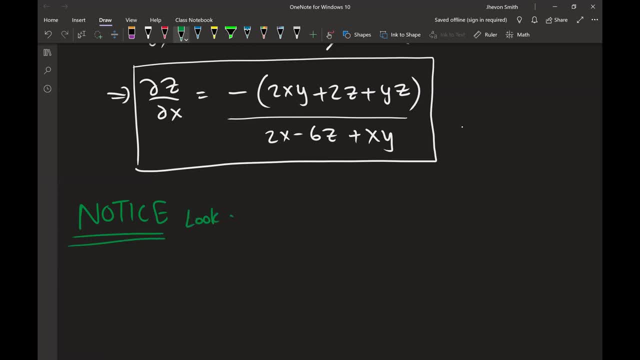 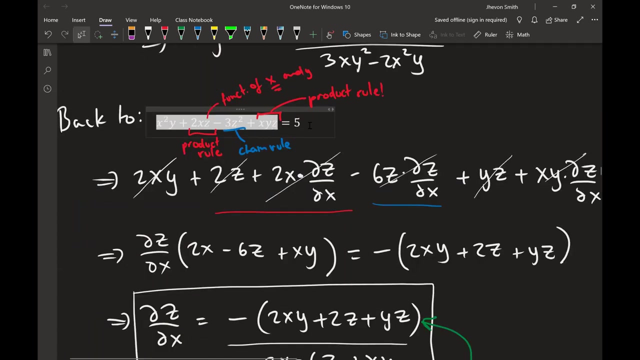 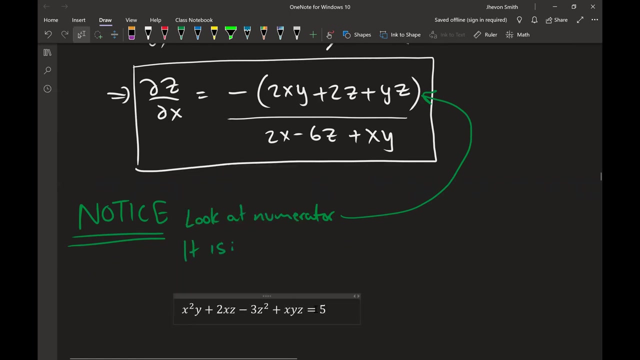 You guys ready? Look at the numerator of the answer I just got. It is watch this internet cut out just as I get to the suspense. the good part, Okay, Look at. look at the function. Okay, Look at the numerator. just the numerator alone and the original function. 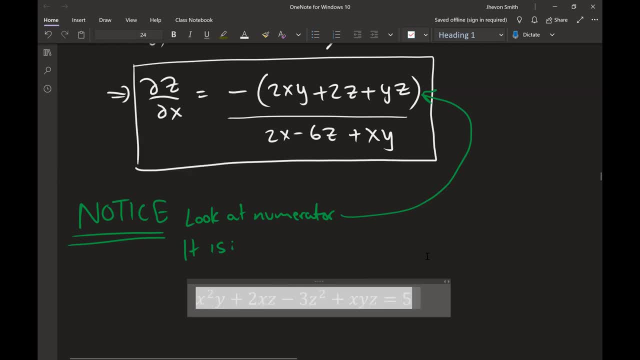 And tell me what you notice. How does the numerator compare to the original equation that I gave you? Look, How does the numerator compare to the original equation that I gave you. Look, Look, It's just a partial worlds ratio. Look. 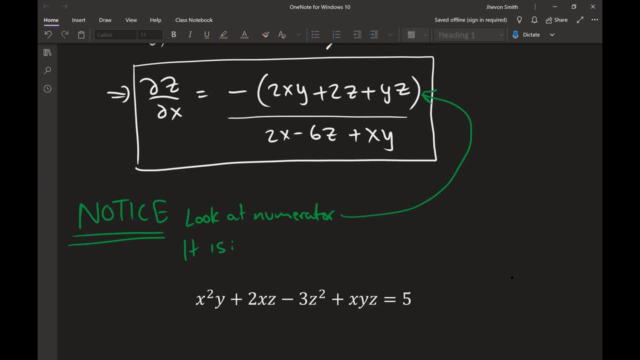 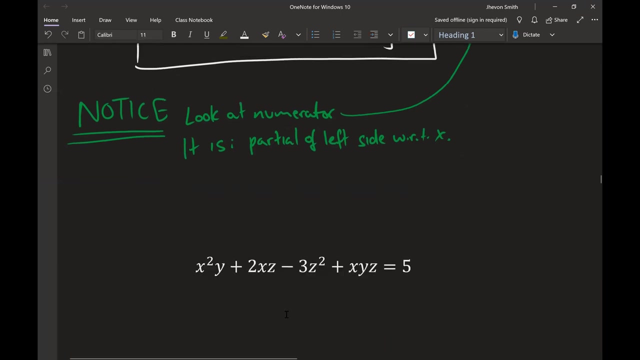 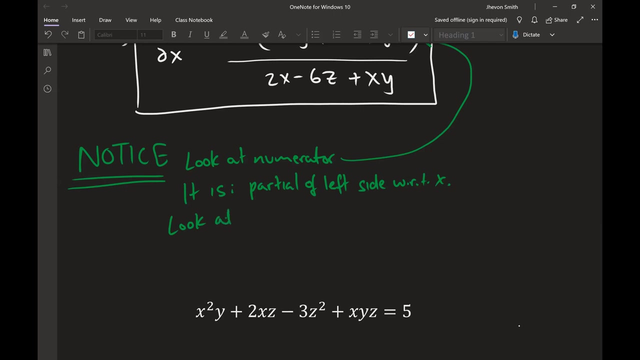 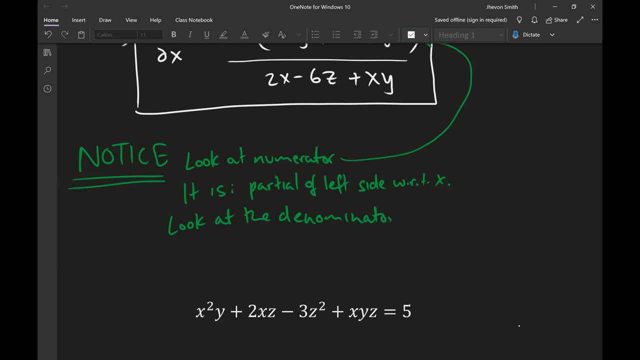 I'm going to show you. I mean, some of you probably see it already, but let me look at the denominator. It is partial of the left side with respect to z. Now let's look at the denominator. So here's a way we can actually express that answer. 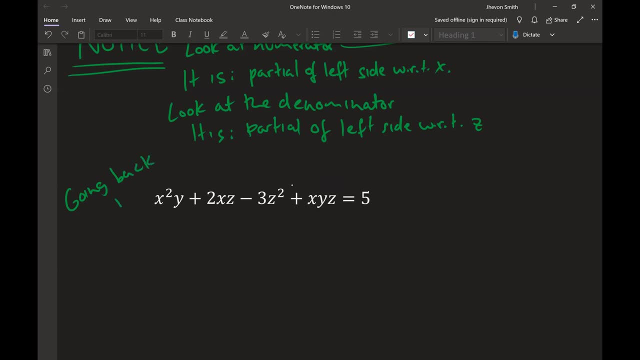 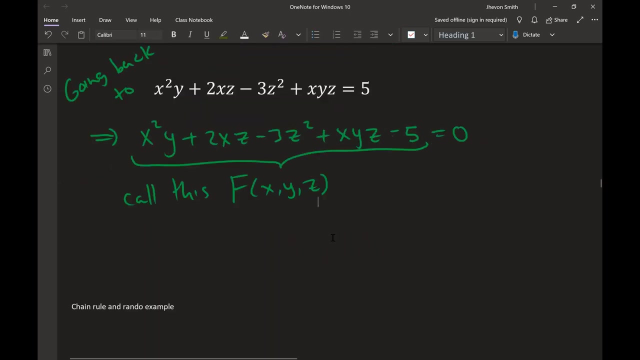 So, going back to this guy, if I bring everything to the right side or the left side and call this entire left side big F, then here's what I want you to notice: The partial with respect to x, partial of z with respect to x is equal to negative. the partial 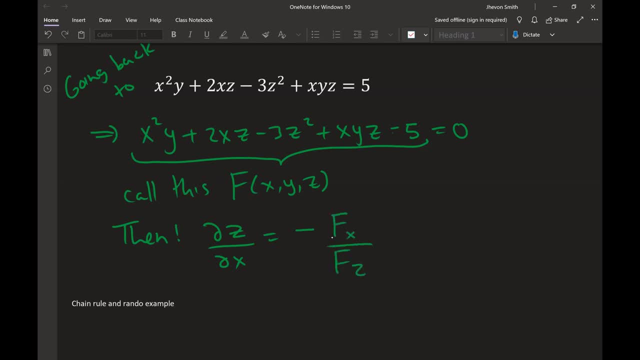 of big F with respect to x divided by the partial of big F with respect to z. In other words, if I were to take the partial of everybody with respect to x and divide by the partial with respect to z, that's actually the answer that I would have gotten if I did implicit differentiation. 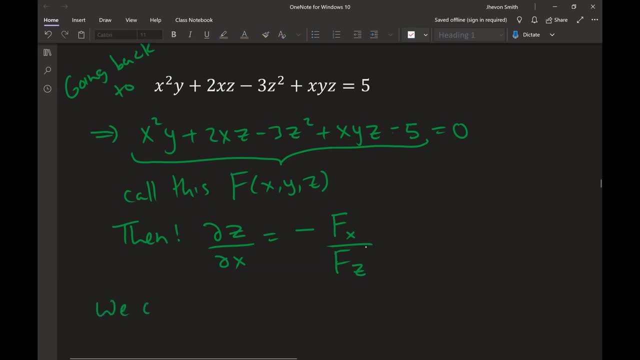 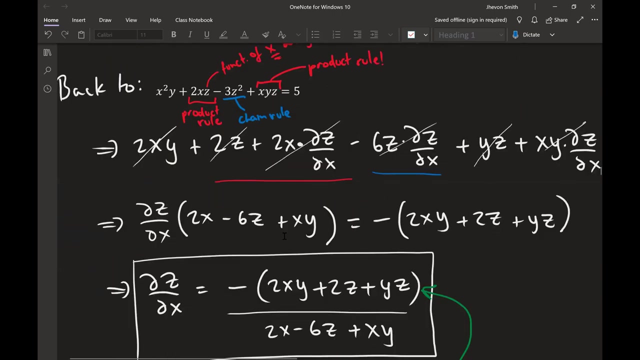 I could now use this formula right And you can get the answer right away, without going through all of these techniques— these— techniques— technical stuff- where you're moving stuff again. Now here's— here's where it's really going to catch you. 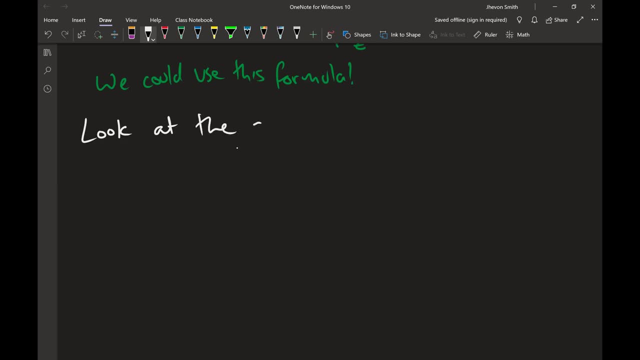 Look at the Calc 1 example again. What I— what I want to show you is that a formula like this will work in general, and it even works in Calc 1, but they couldn't tell you about it in Calc 1 because you didn't know about a partial derivative. 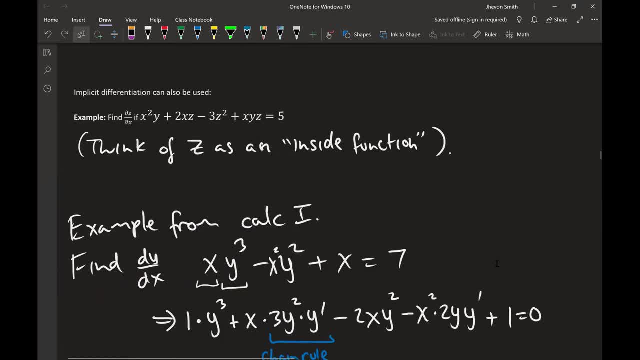 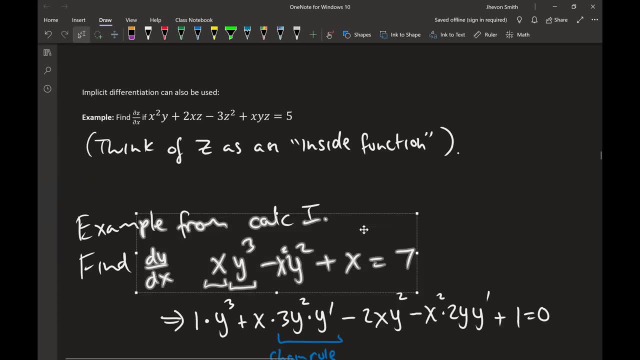 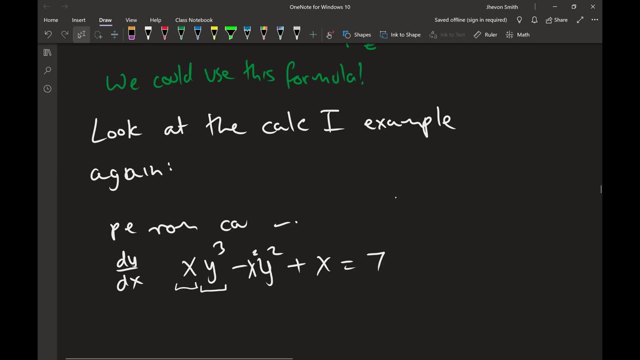 Let me show you Go back to the Calc 1 example. Implicit differentiation probably caused you a lot of headaches. back in Calc 1. Let me show you how trivial it is and could have been. So: find dy dx. if this is true, What I could do is think of this guy here as big F then 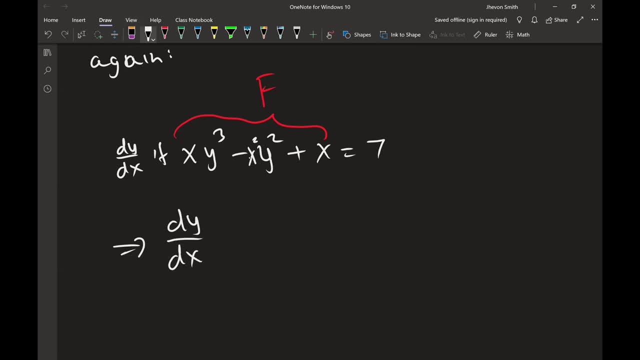 Then my dy dx is just going to be the negative partial with respect to x over partial with respect to y. Go through here. take the partial with respect to x. what do you get? Well, you get y cubed minus 2xy squared plus 1.. 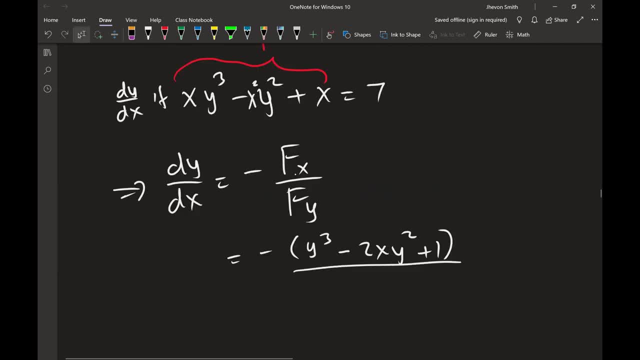 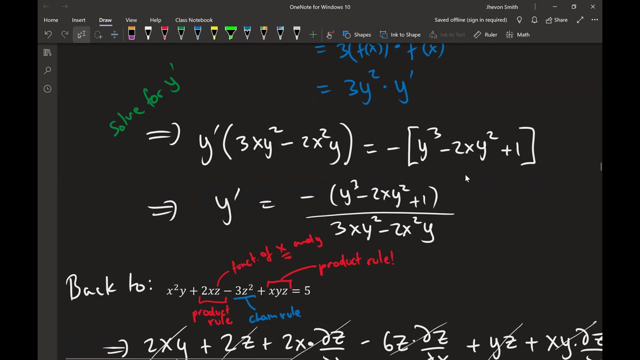 Take the partial with respect to y. what do you get? You would get 3xy squared minus 2x squared y plus, well, 0.. Now look at that And look at what we got before. It's the same guy. 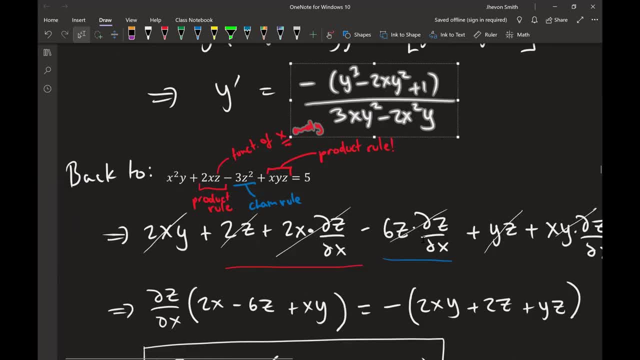 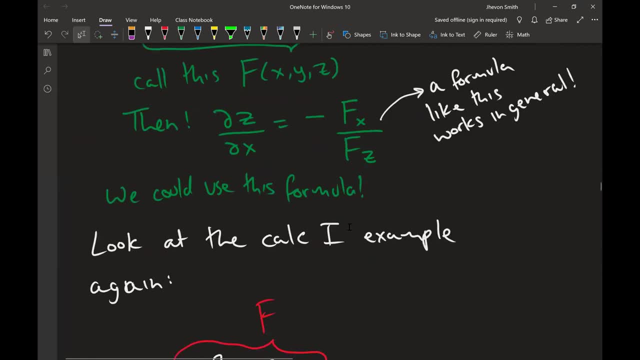 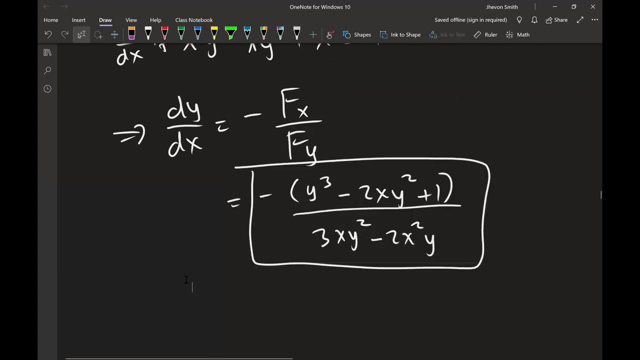 Like implicit differentiation, Didn't have to be. this game where you're applying the chain rule and you're collecting terms and you're moving things to the other side. You could literally use partial derivatives and a simple formula, this ratio, and find an implicit derivative with this. 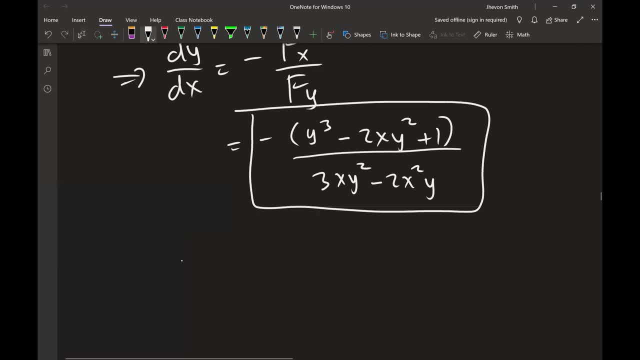 Now this. so if we wanted say the partial of x with respect to y, we could do minus f y over f x. Are you guys still there? I want to make sure I didn't like lose internet. We're here. 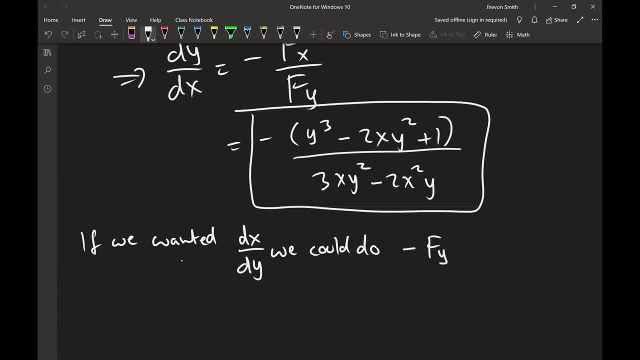 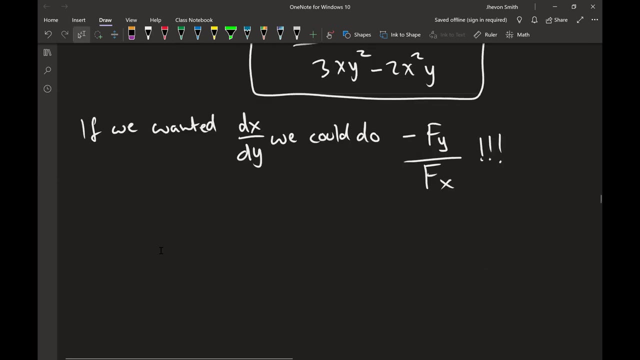 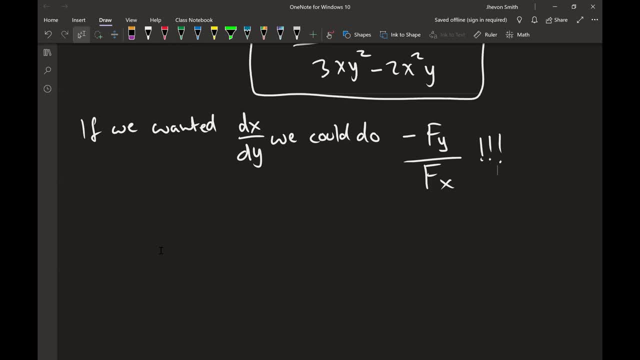 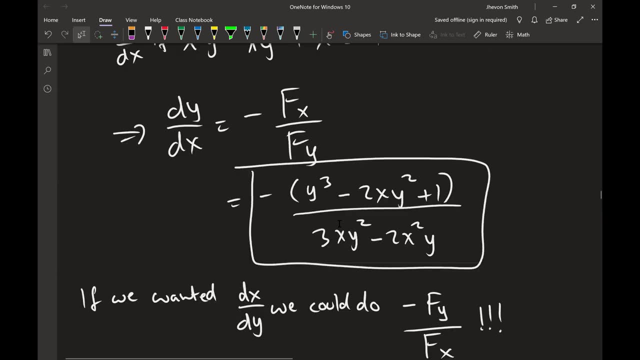 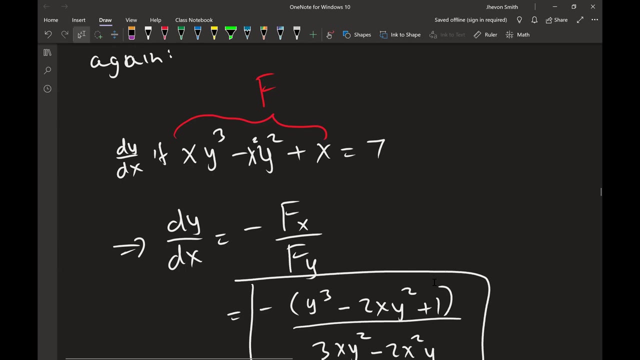 Yeah, Yeah, Yeah, Yeah. So that equals. how gross is that? Like literally, look at that. I could literally just look at this and write down the answer. I can look at this and write down the answer. Let's try it again. 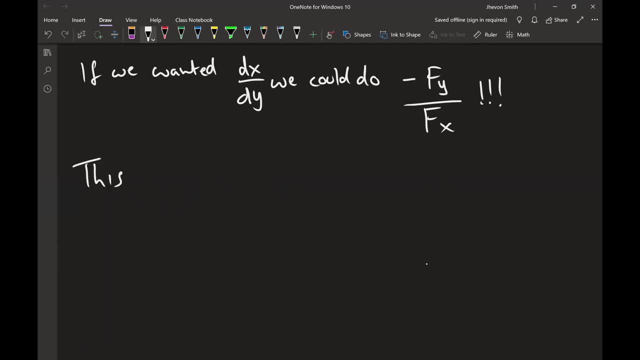 By the way, this comes from a generalization of the chain rule that you will see next, that you'll see in the next class. stay tuned for two, one, three. all right, let me give you guys an example to do, see if you can apply this. all right, so. 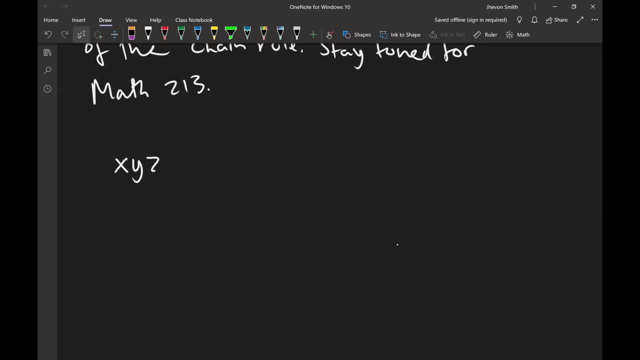 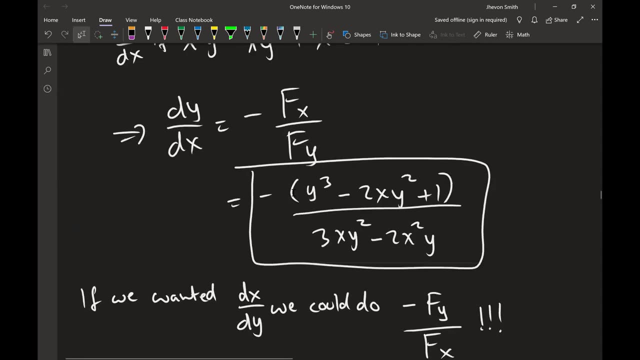 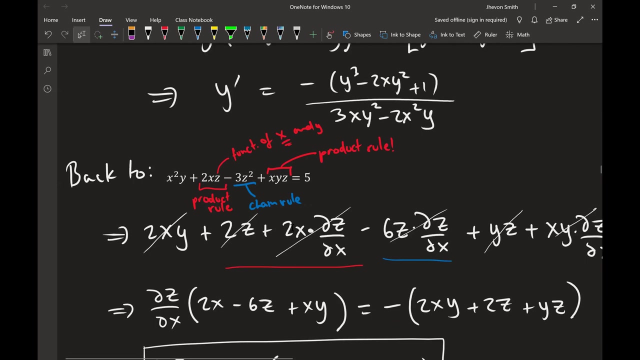 yeah, uh, the last time that we did like. you know why is it negative instead of positive for the numerator? the negative always comes by because we're moving things to the other side. the guys that don't have derivatives attached to them, they are moved to the other side, so it's always going. 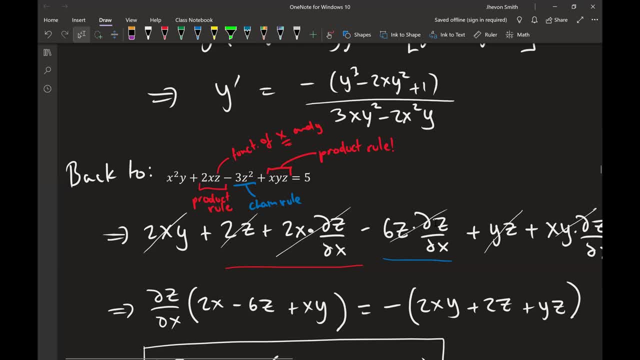 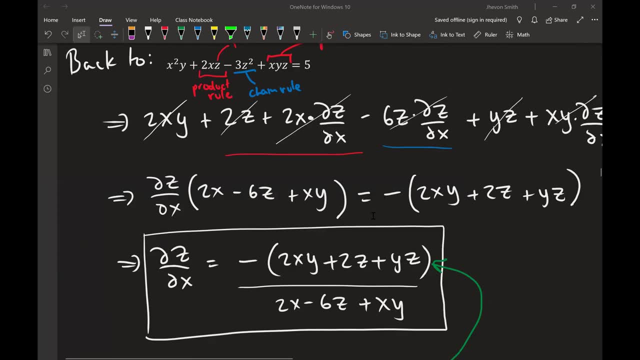 to be a negative because for this problem, because i, when i was trying to solve it, i got jason positive two x y plus two z plus y z over huh over what i got: positive two x y plus two z plus y z over two x minus six z plus x y. okay, you made a mistake if the, if you don't have the negative. 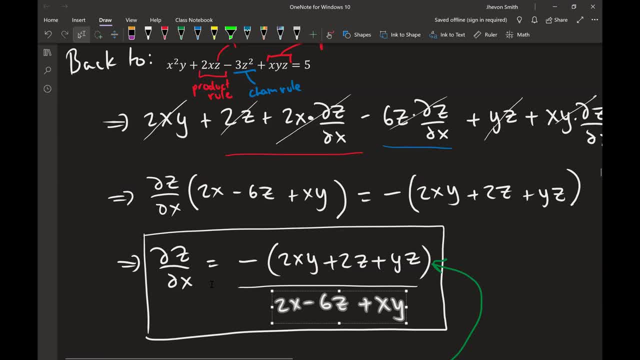 here. you might have a change in sign here, but there definitely should be a negative. if you had two x y plus two z plus y z on the top, you should have six z minus two x minus x y on the bottom. you made a. you made an arithmetic error. 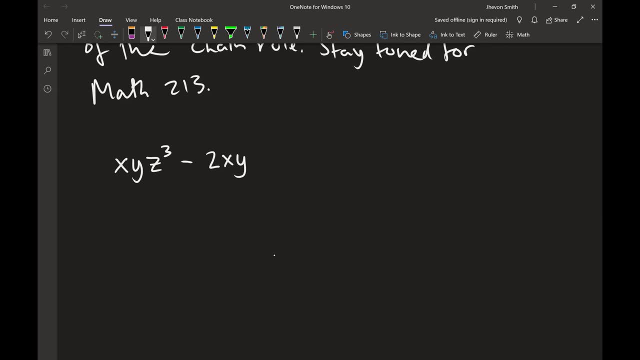 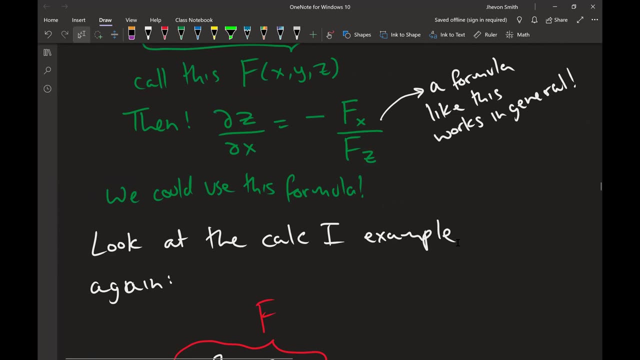 i just want to know what's with the negative, since it's like easy over dx, it's, it's a, very, it's a. what do you mean? what's with the negative? the negative comes from moving things to the other side to get something to the other side, you just, you subtract them. well, how are we able to move? 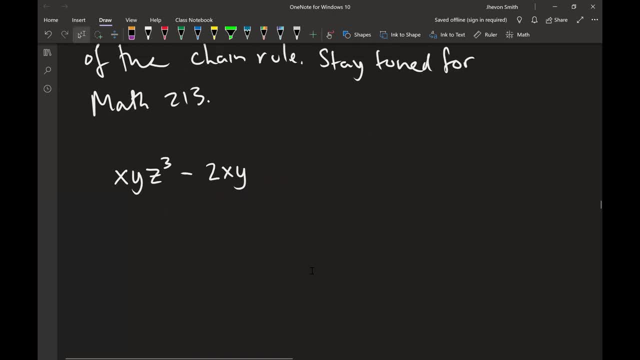 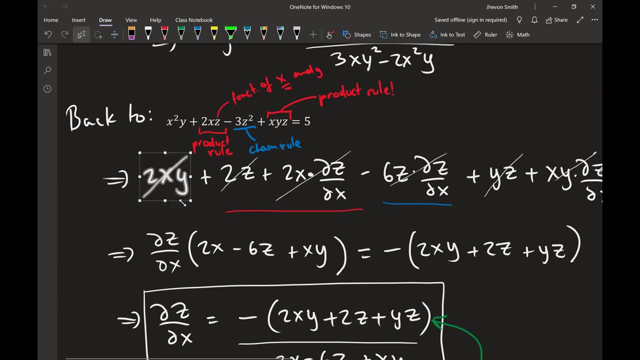 them from the other side. we can interview. please go up by subtracting them from the other side. how would i move this to the other side? i would subtract it. so what do you just basically did with the five though why? it's because of the five i mentioned. 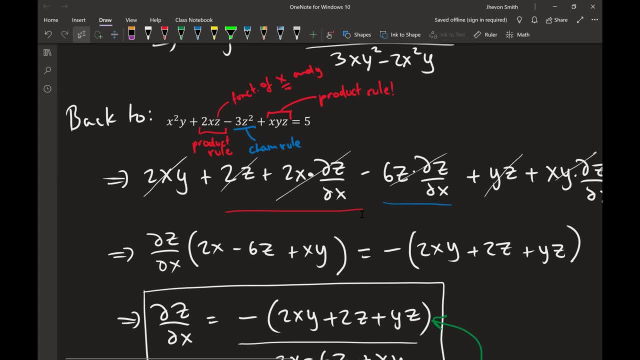 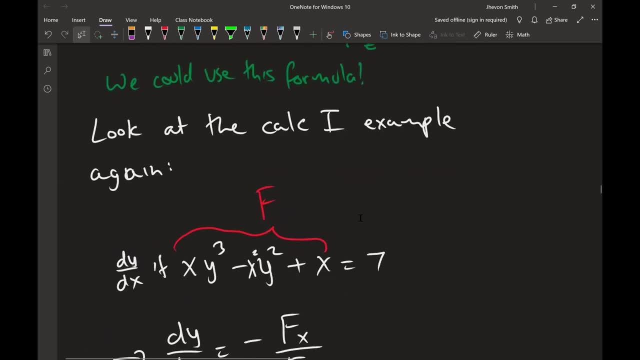 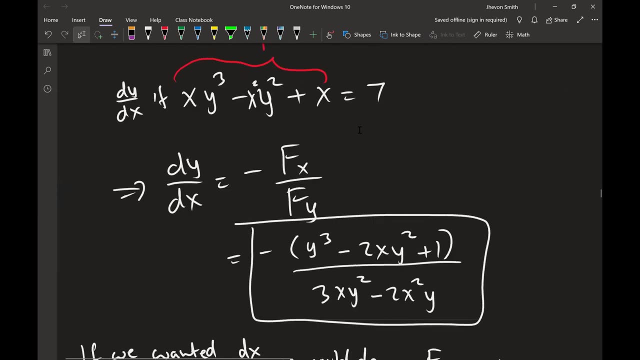 that already. the five is a constant. the derivative of five is zero. the five disappears once i start taking derivatives. why do you have to move things around? why can you just see? what i'm trying to say is: you don't have to move things around. you can use a formula like this: 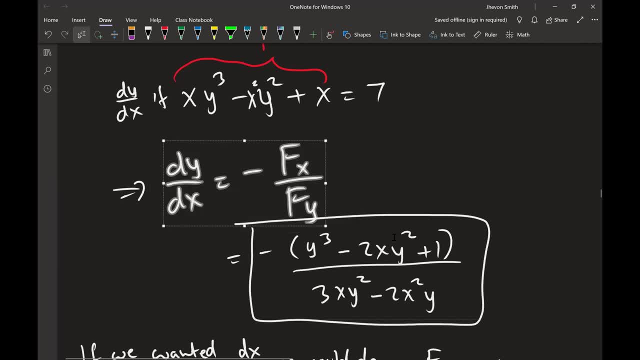 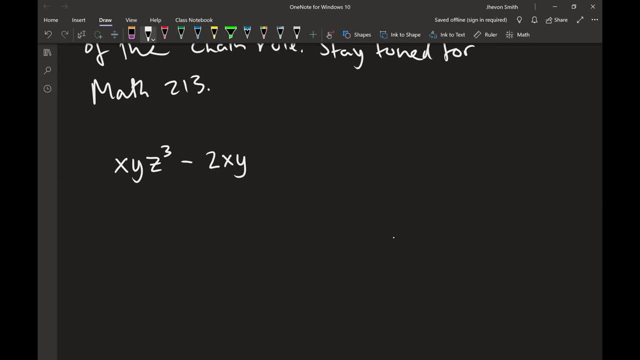 that's the point of this whole thing that i'm trying to show you. you don't have to move things around. let me actually uh, show you again. uh, let's say, i had this. what if i had to find the partial of y with respect to z? 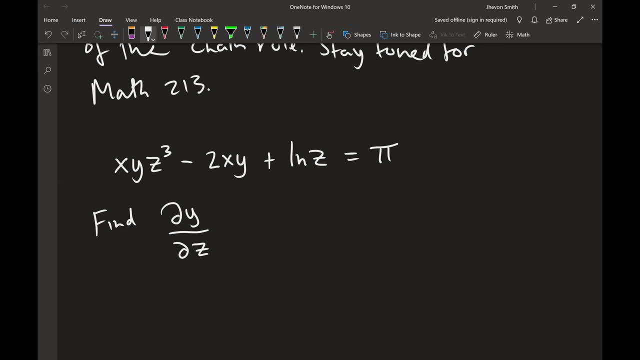 so here you're thinking of y as the inside function. your x and z are independent variables. you could simply go: oh, this is going to be minus big f with respect to z, over the partial of big f with respect to y. the answer is going to be: go through, take the partial with respect to z, you'll. 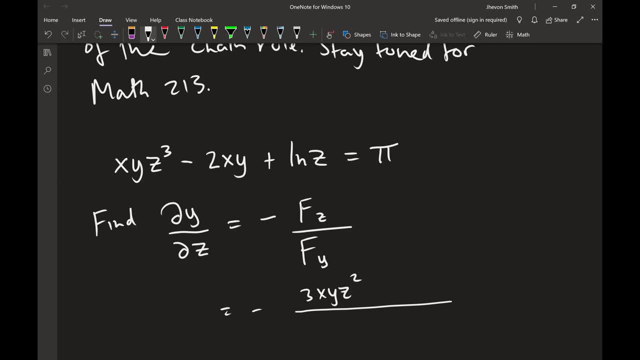 get three x, y, z squared, then you would have plus one over z. then you go through and take the partial with respect to z, plus two z squared, and you pop up a bigger f with respect to y, with respect to y, with the partial with respect to yum, because you've broken it with a small particular function. 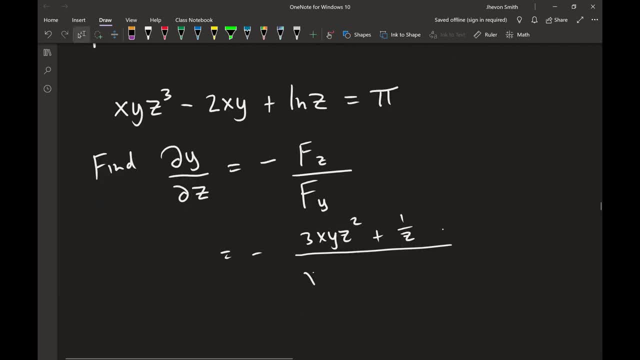 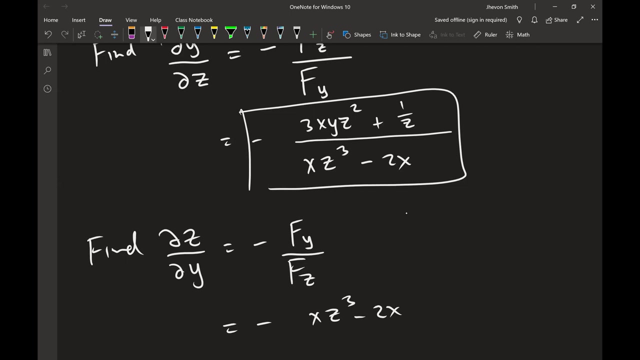 to y, you would have x, z cubed minus 2x. That's your answer. If I had asked you find the partial with respect to z of y, what I would have done is minus partial y over partial z. Then that would just be x, z cubed minus 2x over 3xy, z squared plus 1 over z.